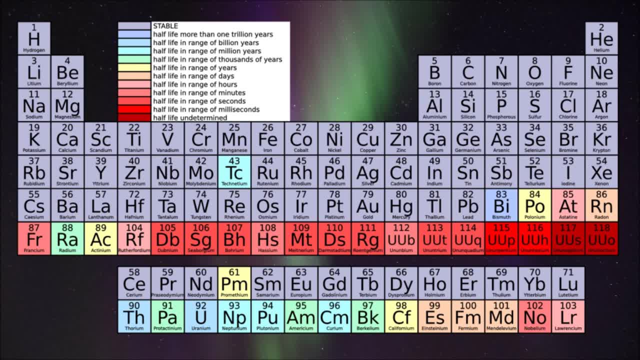 H, hydrogen, H-E, helium, L-I, lithium B-E, beryllium B, boron C, carbon N, nitrogen, O, oxygen F, fluorine, N-E, neon, N-A, sodium, M-G, magnesium, A-L, aluminum, S-I. 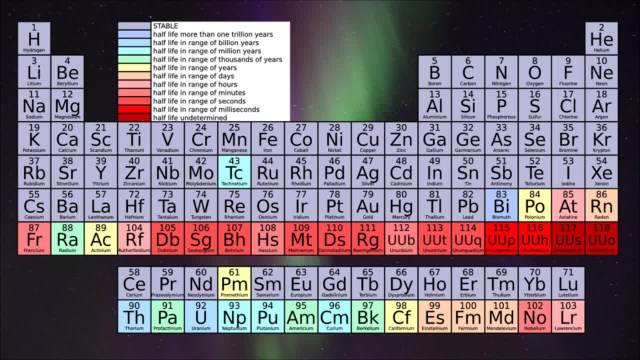 silicon, P, phosphorus S, sulfur, Cl, chlorine, Ar, argon, K, potassium, Ca, calcium, Sc, scandium, Ti, titanium V, vanadium, Cr, chromium, Mn, manganese, Fe, iron, Co, cobalt, Ni, nickel, Cu, copper, Zn, zinc. 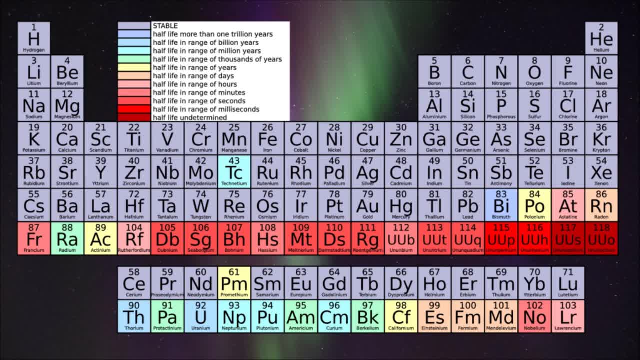 Ga, gallium, Ge, germanium, As. arsenic, Se, selenium, Br, bromine, Kr, krypton, Rb, rubidium, Sr, strontium, Y, yttrium, Zr, zirconium, Nb, niobium, Mo, molybdenum, Tc, technetium, Ru, ruthenium, Rh, rhodium. 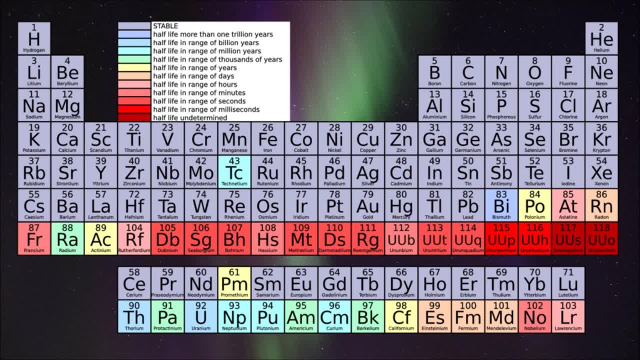 Pd, palladium, Ag, silver, Cd, cadmium In indium, Sn, tin, Sb, antimony, Te, tellurium, I, iodon, Xe, xenon, Cs, cesium. 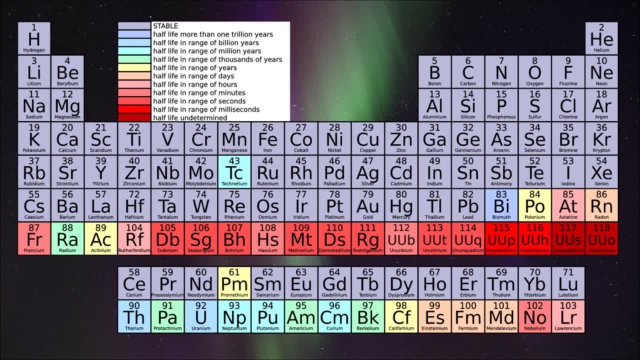 Ba, barium, La lanthanum, Ce, cerium Pr. praseodynium, Nd, neodynium, Pm, promethium, Sm. samarium, Eu, europium, Gd gadolinium. 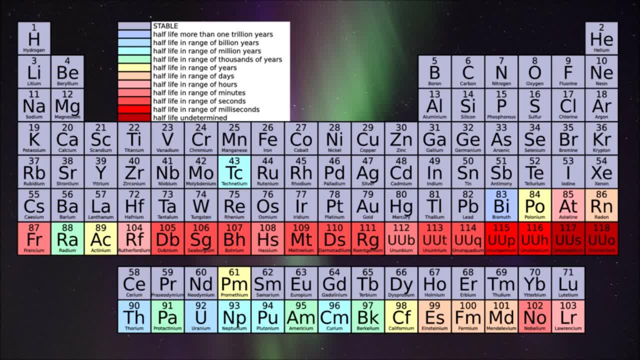 Tb. gadolinium, Rb. cadolinium B. Turbium D Y. Dysprosium H O. Holmium E R. Erbium T M. Thulium Y B Yturbium. L U, Lutetium H F, Hafnium T A, Tantalum W, Tungsten R E, Renium O S, Osmium I, R, Iridium P, T, Platinum A U Gold. 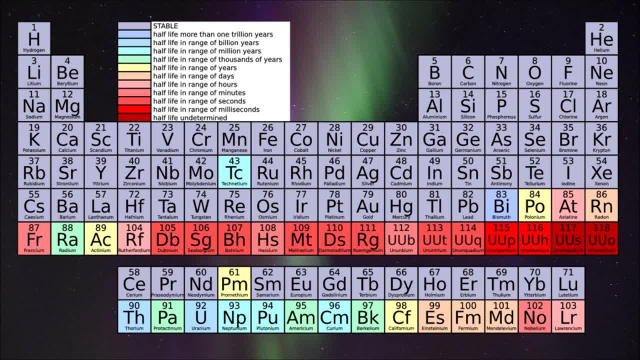 H G, Mercury, T L, Thalium P B, Lead B I, Bismuth, P O, Polonium A, T, Astatine, R N, Radon, F R Francium, R A Radium. 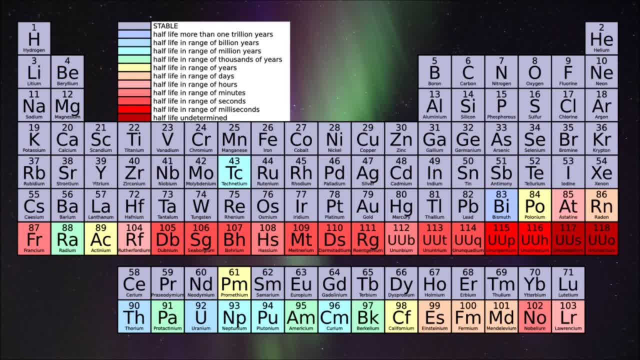 A C. Actinium T H. Thorium P A. Protactinium U. Uranium N P. Neptunium P U. Plutonium A M. Emeritium C M. Curium. 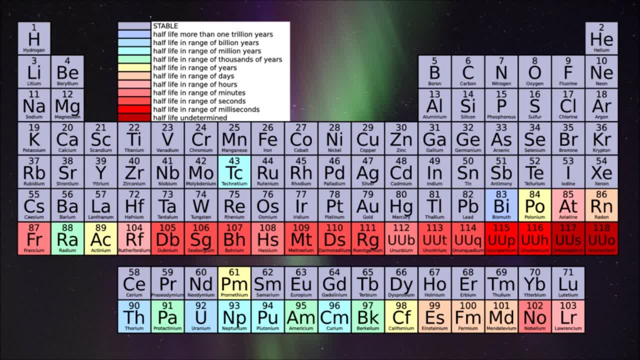 HHydrogen, HE, Helium, LI, Lithium, BE, Beryllium, BB, Boron, CCarbon, NNitrogen, OOxygen, FFluorine, NE, Neon, NA, Sodium, MG, Magnesium, AL, Aluminum, SI, Silicon, PP, Phosphorus. 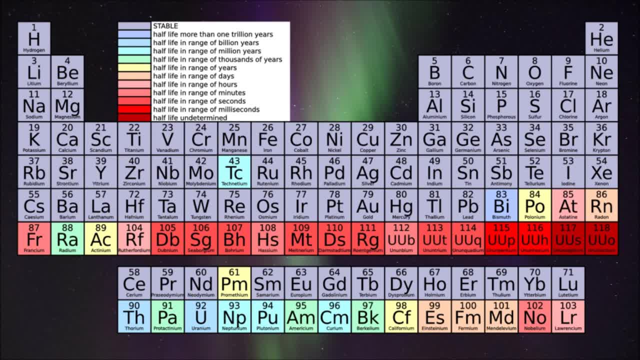 S. Sulfur, CL Chlorine, AR Chlorine, NE, Neon, NA, Sodium, MG, Magnesium, AL, Aluminum, SI, Silicon, PP. Phosphorus, CL Chlorine- AR Chlorine. 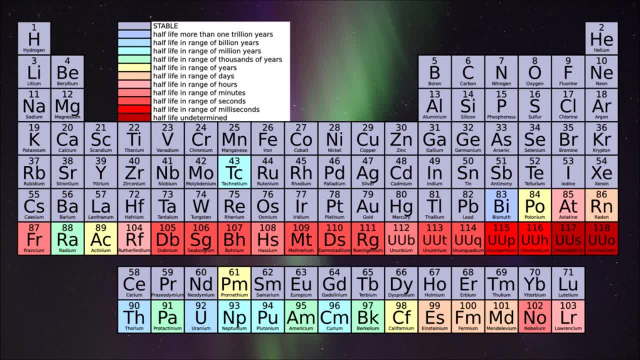 Argon K, Potassium, CA, Calcium, SC, Scandium, TI, Titanium V, Vanadium, CR, Chromium, MN, Manganese, FE, Iron, CO, Cobalt, NI, Nickel, CU, Copper, ZN, Zinc, GA, Gallium, GE, Germanium. 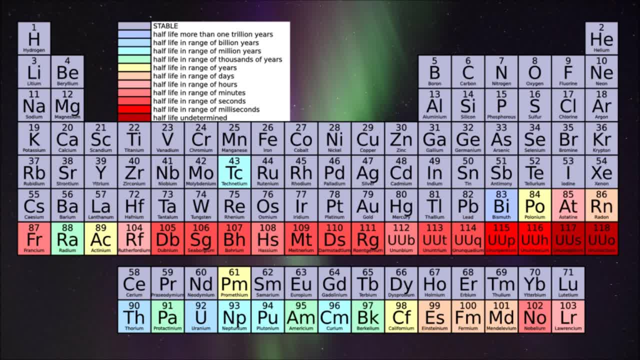 AS. Arsenic, SE, Selenium, BR, Bromine, KR, Krypton, RB, Rubidium, SR, Strontium Y, Yttrium, ZR. Zirconium. NB, Niobium, MO, Molybdenum, TC, Technetium, RU, Ruthenium, RH, Rhodium, PD, Palladium, AG, Silver, CD, Cadmium. 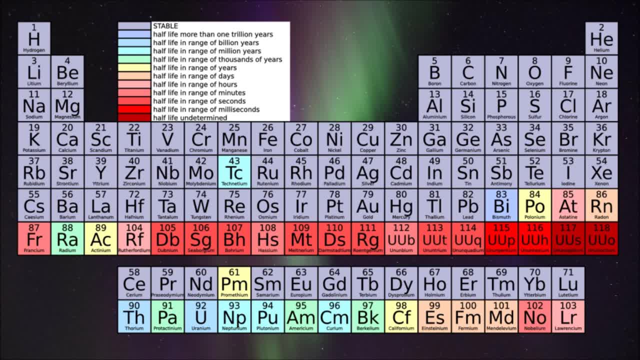 IN Indium, SN, Tin, SB, Antimony, TE, Tellurium, IIodon, XE, Xenon, CS, Caesium, BA, Barium, LA Lanthanum, CE, Cerium. 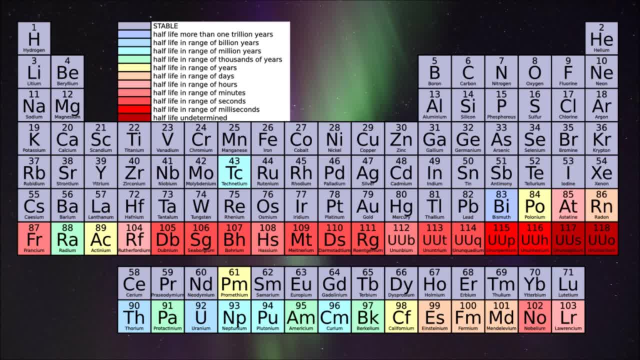 PR: Praseodyneum ND, Neodyneum PN, Neodyneum RD, Neodyneum PS, Neodyneum M, Prometheum S, M, Samarium. 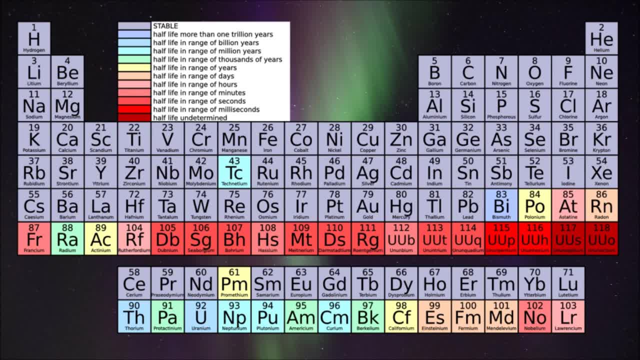 E U Europium G D. Gadolinium T B. Terbium D Y. Dysprosium H O. Holmium E R. Erbium T M Thulium. Y B, Ytterbium, L U, Lutetium H F, Hafnium T A, Tantalum W, Tungsten R E, Rhenium O S, Osmium. 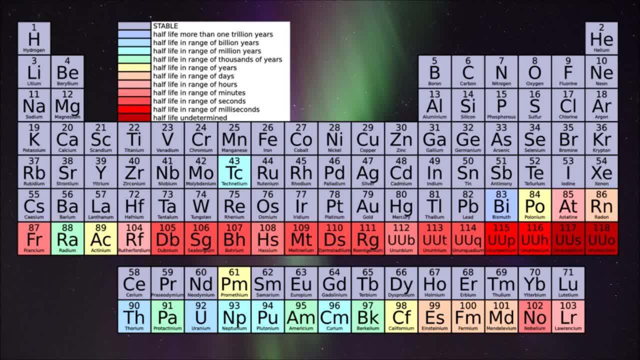 I R, Iridium P T, Platinum A U, Gold, H G, Mercury, T L, Thallium, P B, Lead B I, Bismuth, P O, Polonium. A T, Astatine R N, Radon F R, Francium R A, Radium A C, Actinium T H, Thorium P A, Protactinium. U. Uranium N P, Neptunium P U, Plutonium A M, Emeritium C M, Curium B K, Birkelium C, F, Californium. 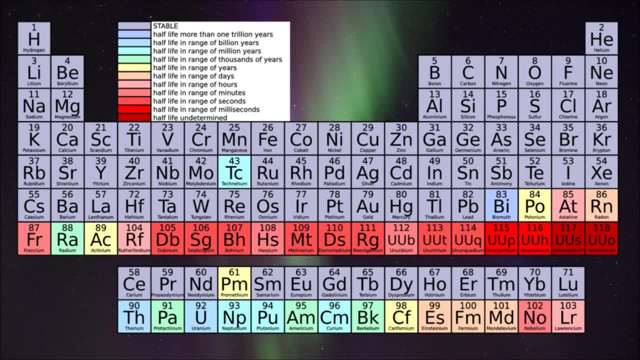 E S, Einsteinium, J D, Vegetation, F, T, P severely hurt my local systems: P S, Rosal A, Triangular L A, Licorice A, F, Exocele. 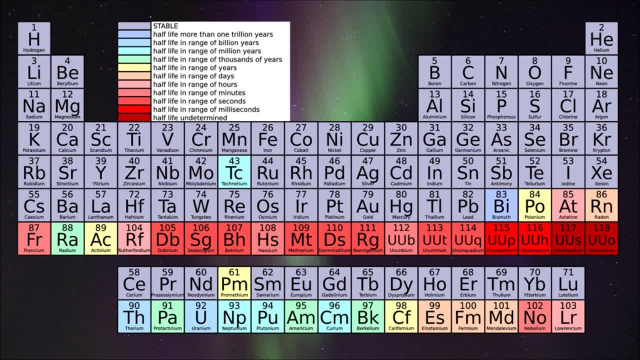 D儿ugin A, Miguel J Odo A, Pas B, Di Zip Qasty QR S. anaerobic DB. Dubnium, SG, Cyborgium, BH, Borium, HS, Hassium, MT, Metnerium, DS, Darmstadium. RG. Runtinium CN. Copernicium UUT. Anuntrium FL. Florovium UUP. Anunpinchium, LV, Livermorium UUS. Anunseption UUO- Anunoxium. 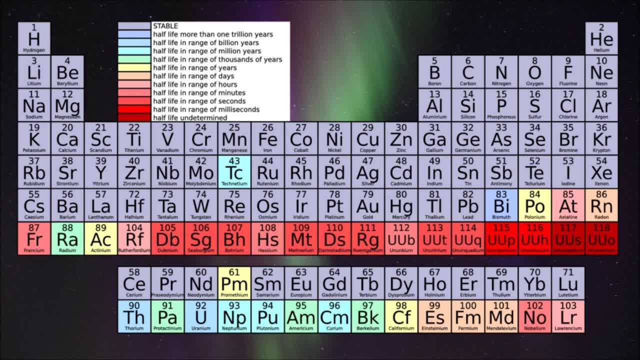 HHydrogen, HE, Helium LI, Lithium BE, Beryllium, BB, Boron, CCarbon, NNitrogen, OOxygen, FFlorium, NE, Neon, NA, Sodium. 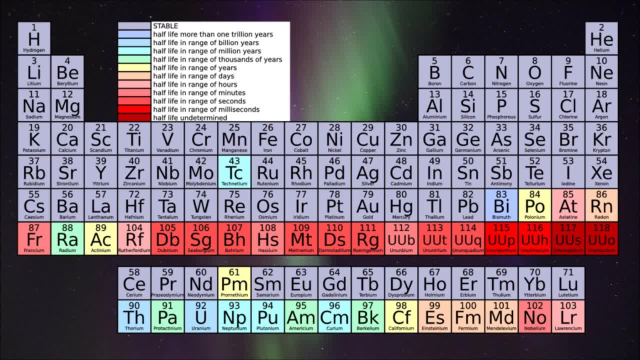 MG, Magnesium, AL, Aluminum, SI, Silicon P, Phosphorus S, Sulfur, CL, Chlorine, AR, Argon K, Potassium, CA, Calcium, SC. Scandium. 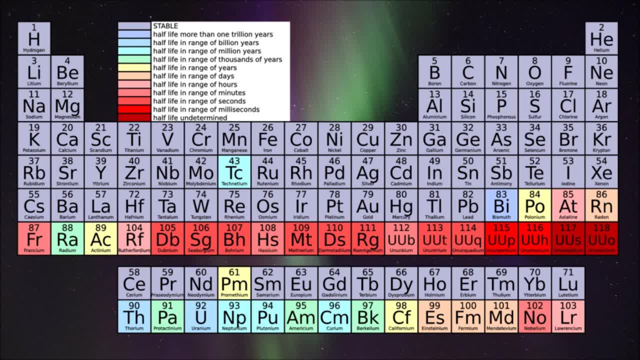 TI, Titanium, V, Vanadium, CR, Chromium, MN, Manganese, FE, Iron, CO, Cobalt, NI, Nickel, CU, Copper, ZN, Zinc, GA, Gallium. 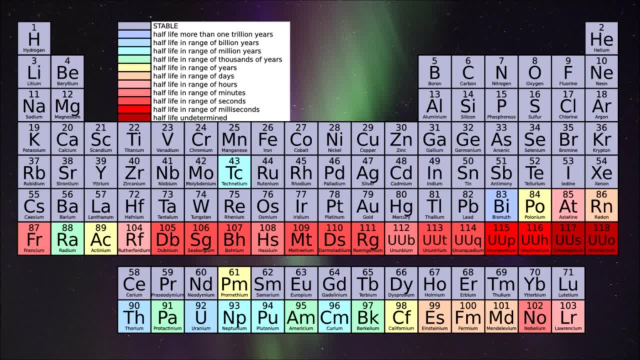 GE, Germanium, AS, Arsenic, SE, Selenium, BR, Bromine, KR, Krypton, RB, Rubidium, SR, Strontium Y, Yttrium. ZR, Zirconium, NB, Niobium, MO, Molybdenum, TC, Technetium, RU, Ruthenium, RH, Rhodium PD, Palladium, AG, Silver. 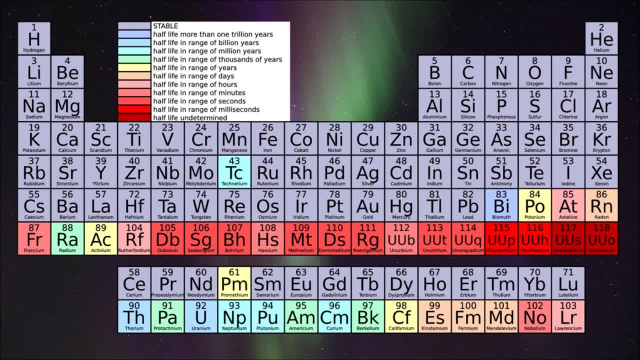 CD, Cadmium IN Indium, SN, Tin, SB, Antimony, TE, Tellurium I, Iodon, XE, Xenon, CS, Cesium, BA, Barium, LA Lanthanum. 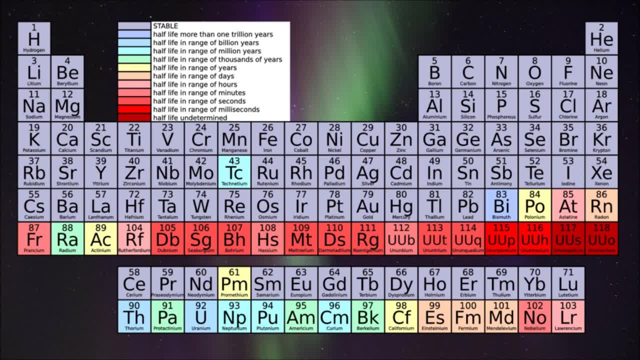 CE: Cerium PR, Praseodynium ND, Neodynium PM, Promethium, SM, Cimmerium EU, Europium GD, Gadolinium TB, Terbium. 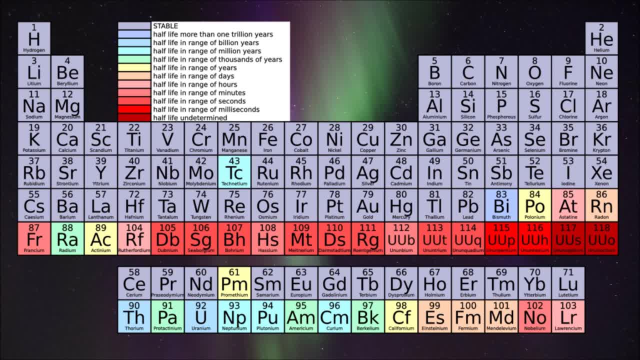 DY. Dysprosium HO. Pulmium ER, Erbium TM, Thulium YB, Ytterbium LU, Lutetium HF, Hafnium, TA, Tantalum. 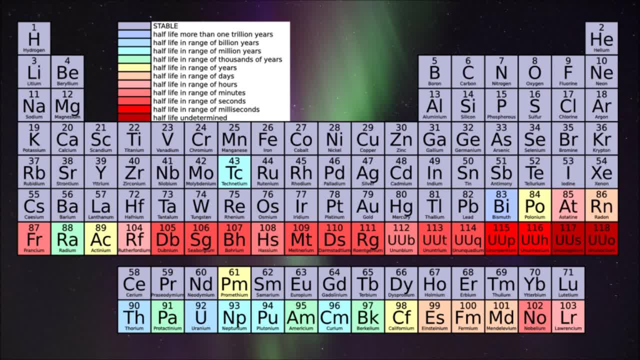 W Tungsten RE, Rhenium, OS, Osmium, IR, Iridium, PT, Platinum, AU, Gold, HG, Mercury, TL, Thallium, PB, Lead. 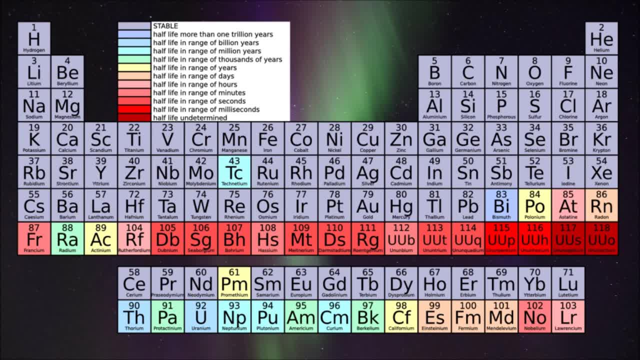 BI Bismuth PO. Polonium AT. Astatine, RN. Radon, FR. Francium, RA. Radium AC, Actinium, TH, Thorium, PA, Protactinium. 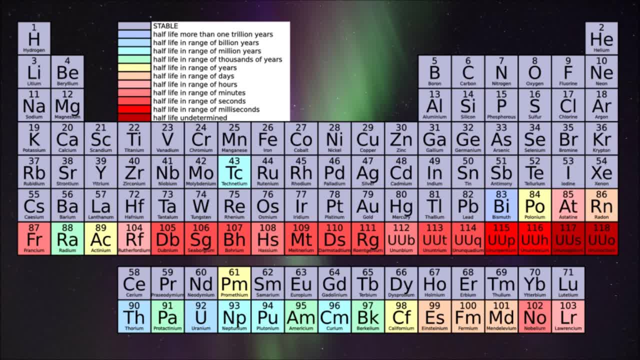 U. Uranium, NP, Neptunium, PU, Plutonium, AM, Ameritium, CM, Curium, BK, Berkelium, CF, Californium, ES, Einsteinium. FM, Fermium, MD, Mendelevium, NO, Nobelium, LR, Laurentium, RF, Rutherfordium, DB, Dubnium, SG, Cyborgium, BH, Borium. HS. Hassium, MT, Mitnerium DS, Darmstadium RG, Runtinium, CN, Copernicium, UUT. Anuntrium FL Florovium. UUP. Anunpinchium LV. Livermorium UUS. Anunseptium UUO. Anunoxium H, Hydrogen, HE, Helium LI, Lithium. 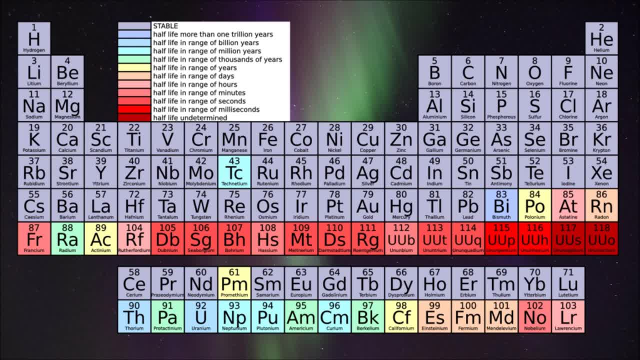 BE, Beryllium, BB, Boron, CC, Carbon, NNitrogen, OOxygen, FFluorine, NE, Neon, NA, Sodium, MG, Magnesium, AL, Aluminum. 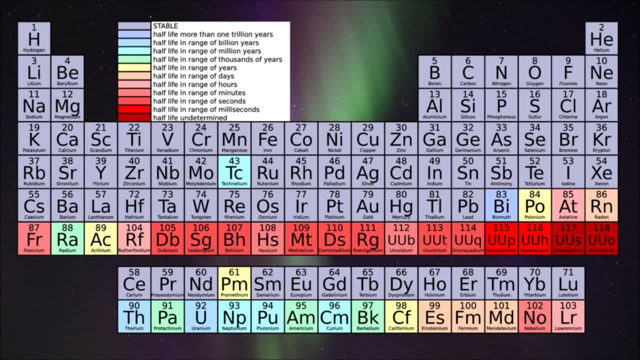 SI, Silicon, PP, Phosphorus, SP, Sulfur, CL, Chlorine, AR, Argon, KP, Potassium, CA, Calcium, SC, Scandium, TI, Titanium. 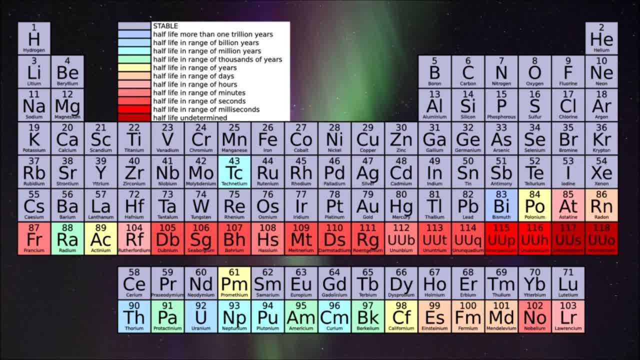 VVanadium, CR, Chromium, MN, Manganese, FE, Iron, CO, Cobalt, NI, Nickel, CU, Copper, ZN, Zinc, GA, Gallium, GE, Germanium. 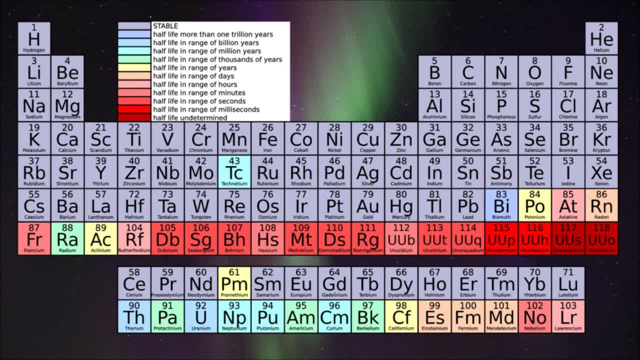 AS. Arsenic, SE, Selenium, BR, Bromine, KR, Krypton, RB, Rubidium, SR, Strontium Y, Yttrium, ZR. Zirconium. 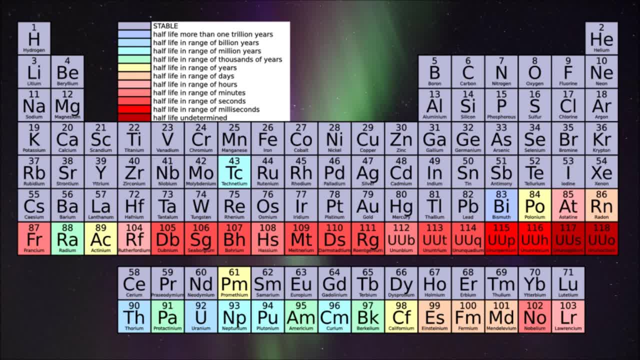 NB, Niobium, MO, Molybdenum, TC, Technetium, RU, Ruthenium, RH, Rhodium CD, Palladium, AG, Silver CD, Cadmium. 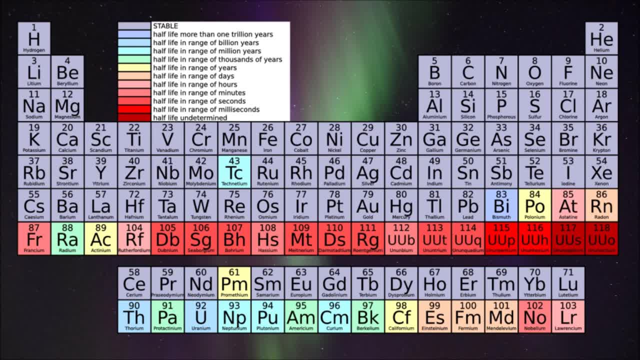 IN Indium, SN, Tin, SB, Antimony, TE, Tellurium I, Iodine, XE, Xenon, CS, Cesium, BA, Barium, LA Lanthanum. 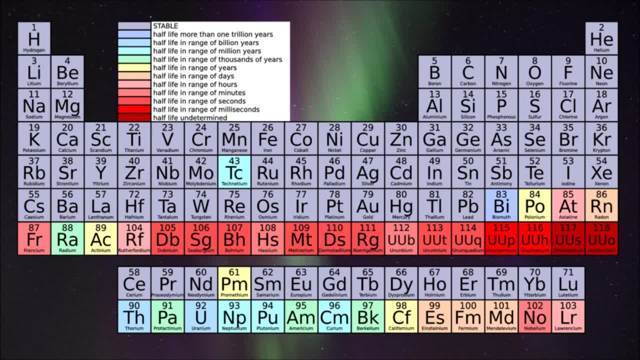 CE Cerium PR, Praseodynium ND, Neodynium PM, Promethium, SM, Samarium, EU, Europium GD, Gadolinium, TB, Terbium. DY. Dysprosium HO. Holmium ER. Erbium TM. Thulium YB. Ytterbium LU. Lutetium HF. Hafnium. 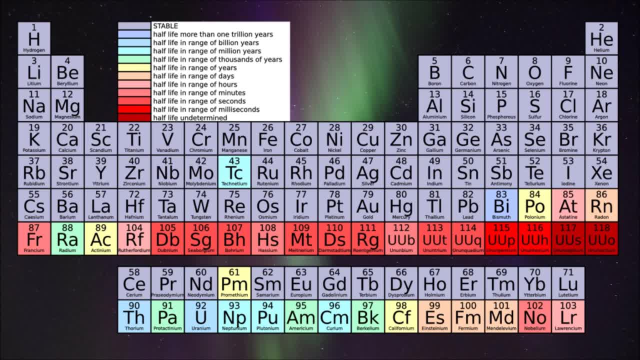 TA. Tantalum W Tungsten RE, Rhenium, OS, Osmium, IR, Iridium, PT, Platinum, AU, Gold, HG, Mercury, TL, Thallium. 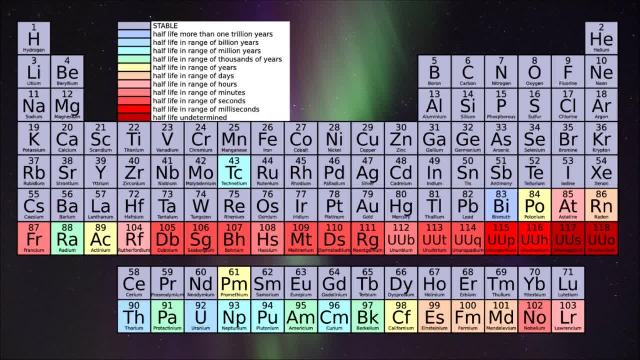 PB Lead BI. Bismuth PO. Polonium AT, Astatine, RN. Radon FR. Francium, RA. Radium AC, Actinium TH, Thorium. 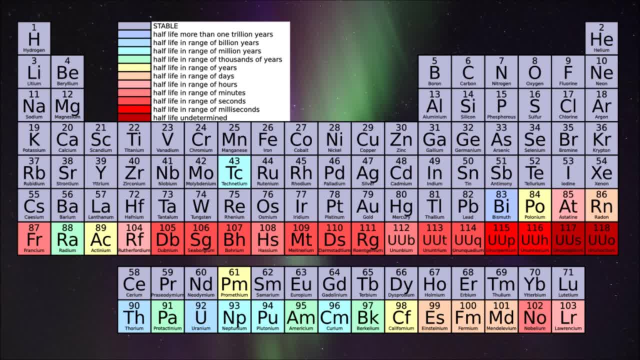 PA, Protactinium U, Uranium, NP, Neptunium, PU, Plutonium AM, Emeritium CM, Curium PK, Berkelium, CF, Californium. ES, Einsteinium, FM, Fermium, MD, Mendelevium, NO, Nobelium, LR, Laurentium, RF, Rutherfordium, PB, Dubnium, SG, Cyborgium. BH, Borium, HS, Hacium, MT, Mitnerium, DS, Darmstadium, RG, Runtinium, CN, Copernicium, UUT. Anuntrium. FL. Fluorovium UUP. Anunpincium LV. Livermorium UUS. Anunseptium UUO. Anunoxium H, Hydrogen, HE, Helium. 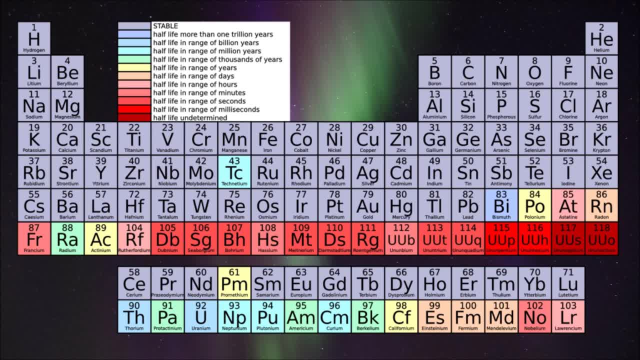 LI, Lithium, BE, Beryllium, BB, Boron, CC, Carbon, NNitrogen, OOxygen, FFluorine, NE, Neon, NA, Sodium, MG, Magnesium. 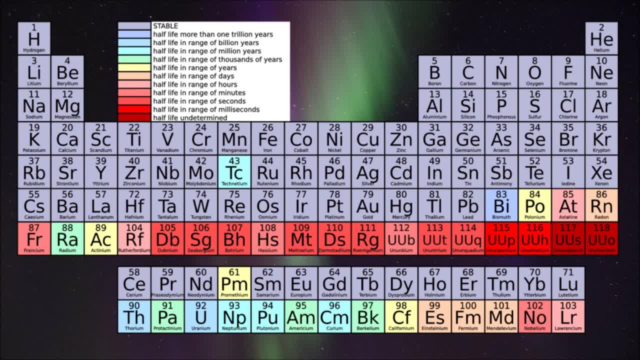 AL, Aluminum, SI, Silicon P, Phosphorus S, Sulfur, CL, Chlorine, AR, Argon K, Potassium, CA, Calcium, SC. Scandium. 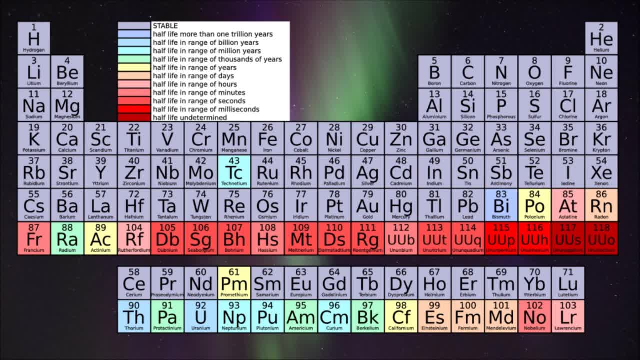 TI, Titanium, V, Vanadium, CR, Chromium, MN, Manganese, FE, Iron, CO, Cobalt, NI, Nickel, CU, Copper, ZN, Zinc, GA, Gallium. 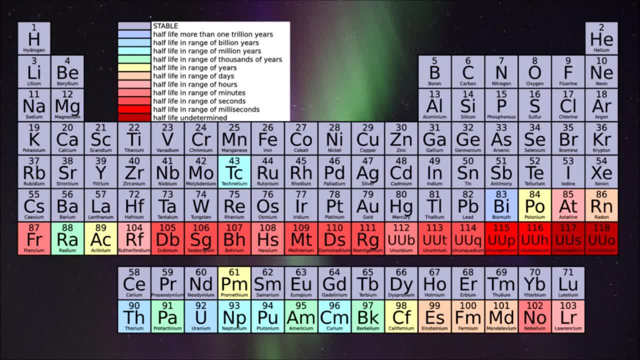 GE, Germanium, AS, Arsenic, SE, Selenium, BR, Bromine, KR, Krypton, RB, Rubidium, SR, Strontium Y, Yttrium. ZR, Zirconium, NB, Niobium, MO, Molybdenum, TC, Technetium, RU, Ruthenium, RH, Rhodium PD, Palladium, AG, Silver. 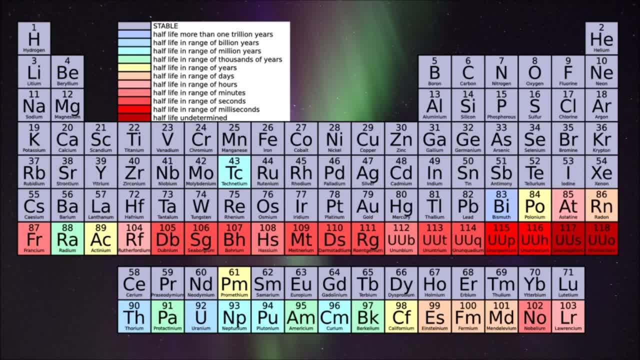 CD Cadmium IN Indium SN, Tin, SB, Antimony ET Tellurium IIodon, XE, Xenon, CS, Cesium, BA, Barium. 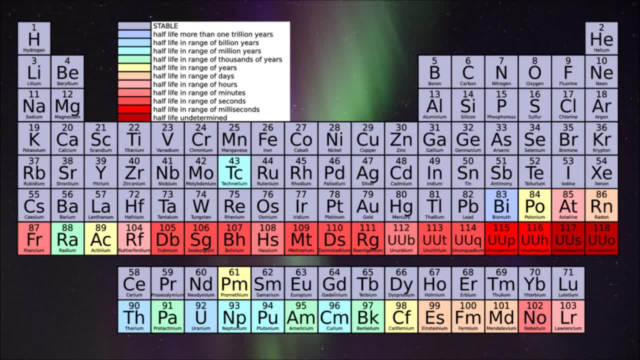 LA Lanthanum, CE, Cerium PR, Praseodynium ND, Neodynium PM, Promethium, SM, Samarium, EU, Europium, GD, Gadolinium. 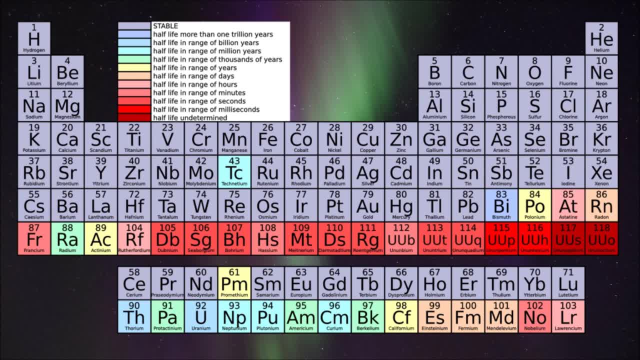 TB. Terbium DY. Dysprosium HO. Holmium ER. Erbium TM. Thulium YB. Ytterbium LU Lutetium. HF, Hafnium, TA, Tantalum, W, Tungsten, RE, Rhenium, OS, Osmium, IR, Iridium, PT, Platinum, AU, Gold. 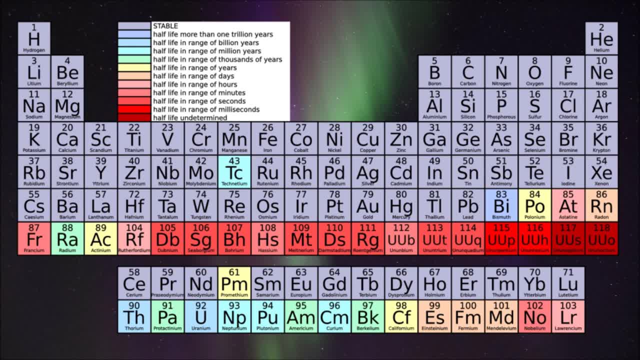 HG Mercury TL. Thallium, PB, Lead BI, Bismuth PO. Polonium AT, Astatine RN. Radon FR, Francium, RA Radium. 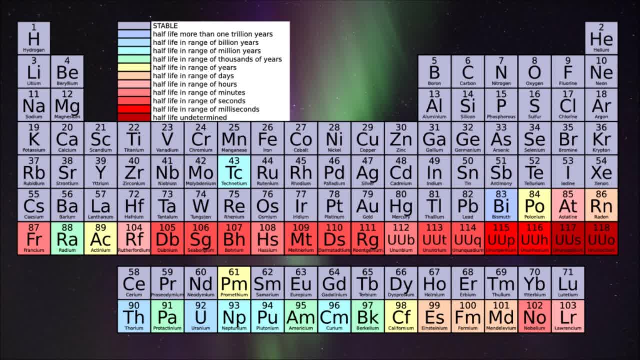 AC, Actinium, TH, Thorium, PA, Protactinium U, Uranium, NP, Neptunium PU, Plutonium AM, Ameritium, CM, Curium. BK, Berkelium, CF, Californium, ES, Einsteinium, FM, Fermium, MD, Mendelevium, NO, Nobelium, LR, Laurentium, RF Rutherfordium. DB, Dubnium, SG, Cyborgium, BH, Borium HS, Hassium, MT, Metnerium, DS, Darmstadium, RG, Runtinium, CN, Copernicium. UUT. Anuntrium FL. Florovium UUP. Anunpincium LV. Livermorium UUS. Anunseptium UUO- Anunoxium. 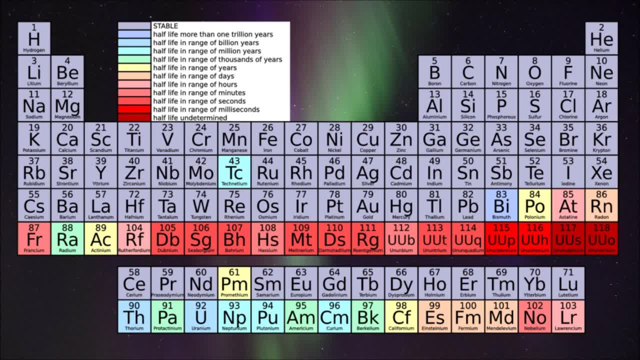 HHydrogen, HE, Helium LI, Lithium BE, Beryllium, BB, Boron, CC, Carbon, NNitrogen, OOxygen, FFluorine. 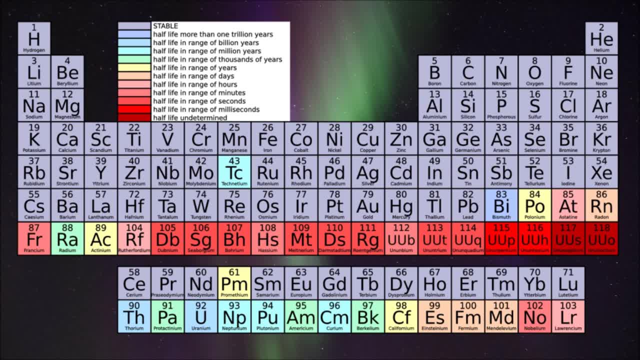 NE, Neon, NA, Sodium, MG, Magnesium, AL, Aluminum, SI, Silicon, P, Phosphorus S, Sulfur, CL, Chlorine, AR, Argon, K, Potassium. 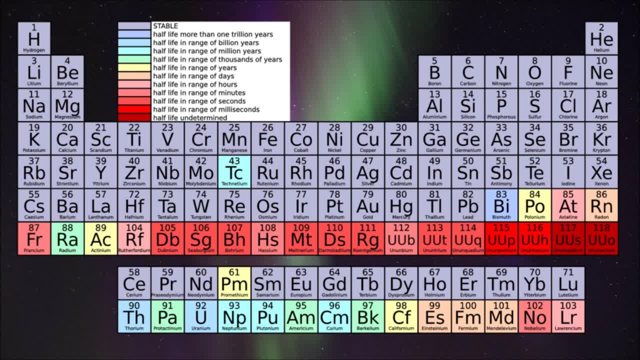 CA, Calcium, SC, Scandium, TI, Titanium V, Vanadium, CR, Chromium, MN, Manganese, FE, Iron, CO, Cobalt, NI, Nickel, CU, Copper. 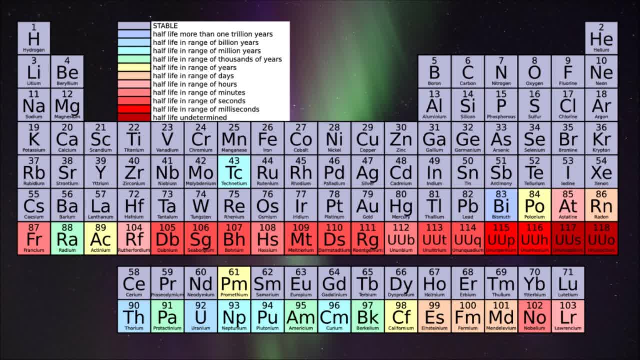 ZN, Zinc, GA, Gallium, GE, Germanium, AS, Arsenic, SE, Selenium, BR, Bromine, KR, Krypton, RB, Rubidium, SR, Strontium. Y Yttrium, ZR, Zirconium NB, Niobium, MO, Molybdenum TC, Neon TC, Technetium RU, Ruthenium, RH, Rhodium. 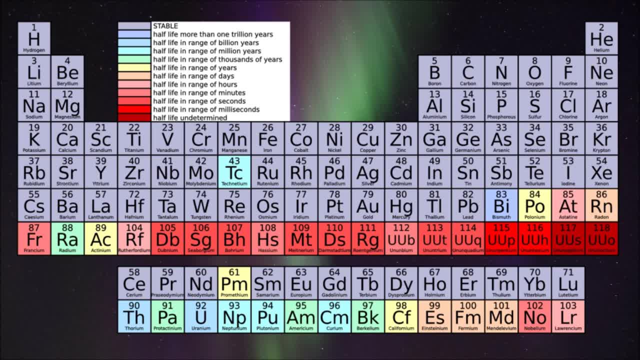 PD, Palladium, AG, Silver, CD, Cadmium IN Indium, SN, Tin, SB, Antimony, TE, Tellurium, IIodon, XE, Xenon. 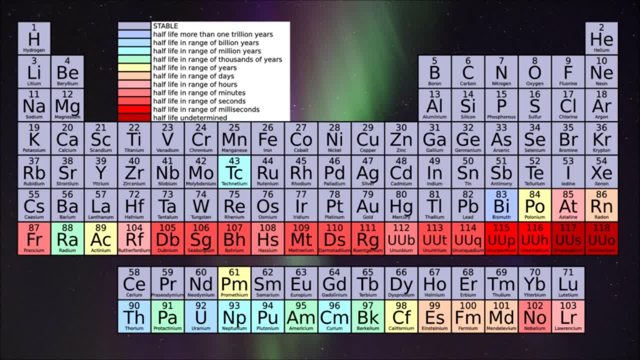 CS, Cesium, BA, Barium, LA, Lanthanum CE, Cerium PR, Praseodynium, ND, Neodynium PM, Promethium, SM, Cimmerium. 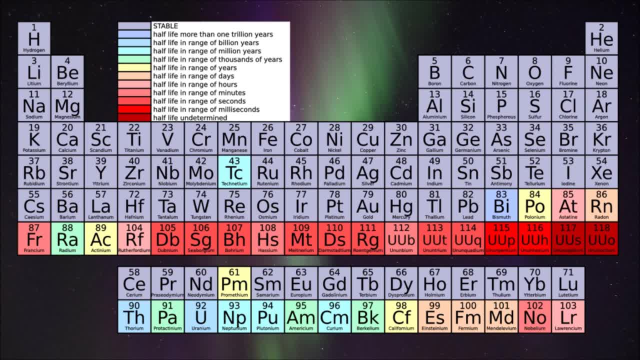 EU, Europium GD. Gadolinium TB. Terbium DY. Dysprosium HO. Holmium ER. Erbium TM. Thulium YB. Ytterbium. LU. Lutetium HF, Hafnium, TA, Tantalum W, Tungsten RE, Rhenium, OS, Osmium, IR, Iridium PT, Platinum. 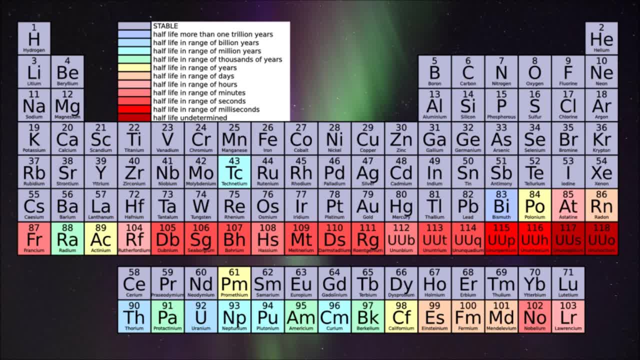 AU Gold, HG, Mercury, TL, Thallium, PB, Lead, BI, Bismuth, PO, Polonium, AT, Astatine, RN, Radon, FR. Francium. 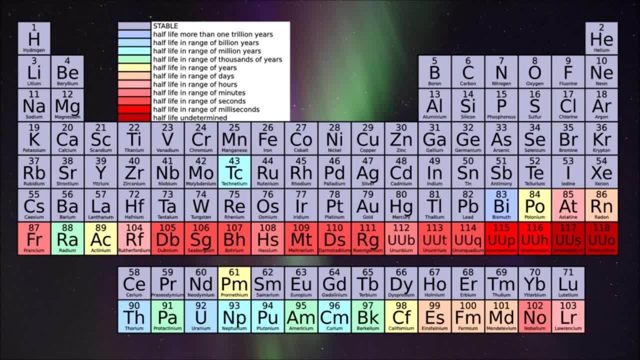 RA, Radium AC, Actinium TH, Thorium PA, Protactinium U, Uranium NP, Neptunium PU, Plutonium AM, Ameritium. CM, Curium, BK, Berkelium, CF, Californium, ES, Einsteinium, FM, Fermium MD. Mendelevium, NO Nobelium LR Lorentzium. RF Rutherfordium DB Dubnium SG, Cyborgium BH, Borium HS, Hassium MT, Mitnerium DS Darmstadium, RG Runtinium. 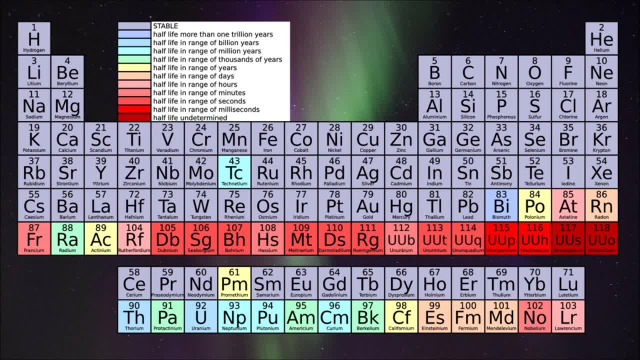 CN. Copernicium UUT. Anuntrium FL. Fluorovium UUP- Anunpincium LV. Livermorium UUS- Anunseption. UUO, Anunoxium, HHydrogen, HE, Helium, LI, Lithium, BE, Beryllium, BB, Boron, CC, Carbon, NNitrogen, OOxygen. 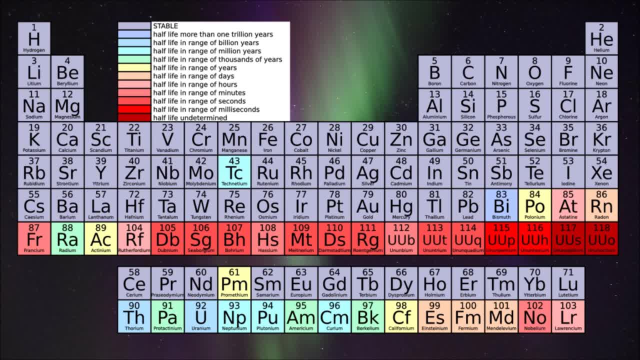 FFluorine, NE, Neon, NA, Sodium, MG, Magnesium, AL, Aluminum, SI, Silicon, P, Phosphorus S, Sulfur, CL, Chlorine, AR, Argon. 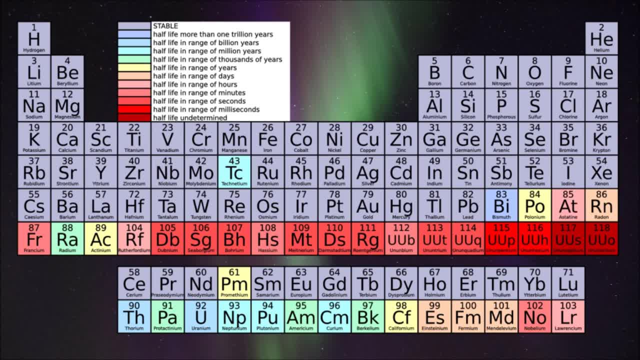 K, Potassium, CA, Calcium, SC, Scandium, TI, Titanium V, Vanadium, CR, Chromium, MN, Manganese, FE, Iron, CO, Cobalt, NI, Nickel. 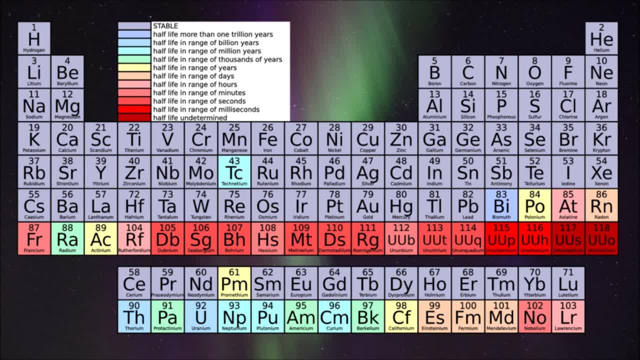 CU, Copper, ZN, Zinc, GA, Gallium, GE, Germanium, AS, Arsenic, SE, Selenium, BR, Bromine, KR, Krypton, RB, Rubidium. 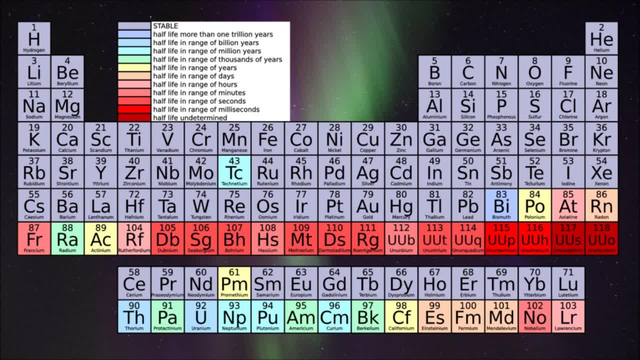 SR Strontium, Y Yttrium, ZR Zirconium, NB, Niobium, MO, Molybdenum, TC Technetium RU Ruthenium. 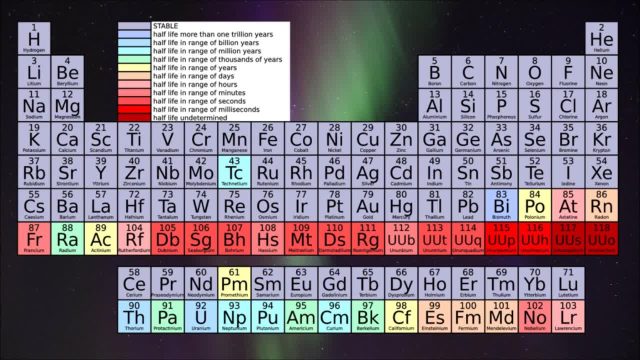 RH, Rhodium, PD, Palladium, AG, Silver, CD, Cadmium IN Indium, SN, Tin, SB, Antimony, TE, Tellurium I, Iodon. 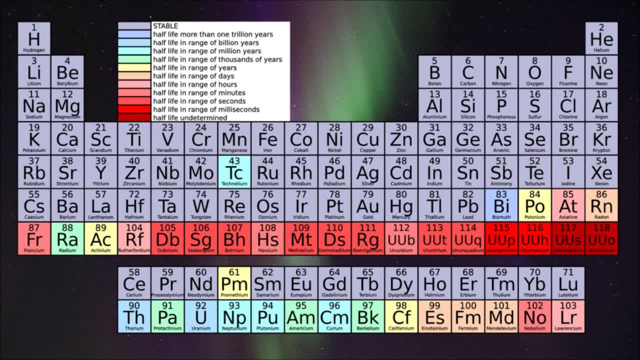 XE, Xenon, CS, Cesium, BA, Barium, LA, Lanthanum, CE, Cerium, PR, Praseodynium, ND, Neodynium, PM, Promethium. 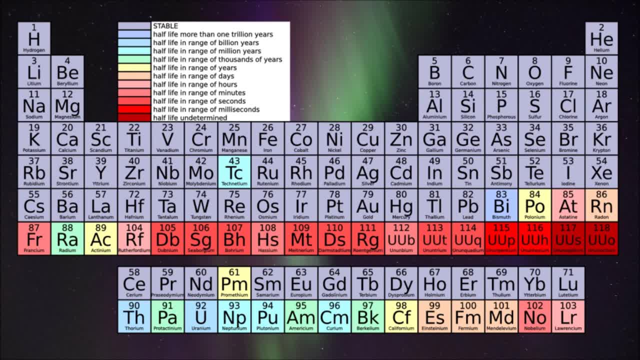 SM Cimmerium EU, Europium GD. Gadolinium TB Terbium DY. Dysprosium HO. Holmium ER Erbium TM Thulium. 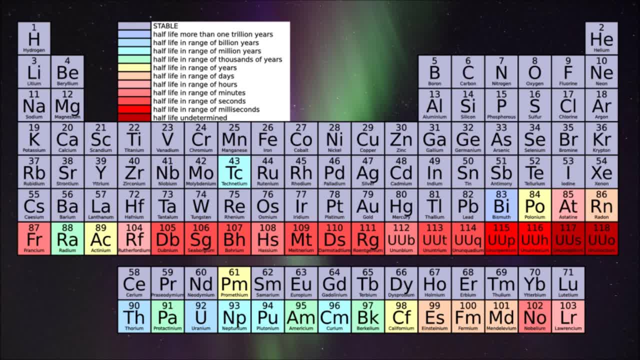 IR Iridium: PT, Platinum, AU, Gold, HG, Mercury, TL, Thallium, PB, Lead, BI, Bismuth, PO, Polonium, AT Astatine. 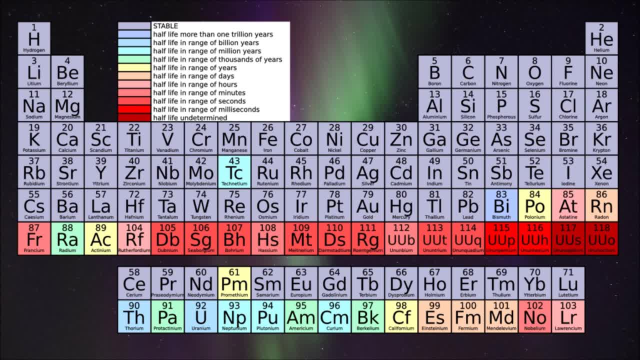 RN, Radon, FR, Francium, RA, Radium AC, Actinium, TH, Thorium, PA, Protactinium U, Uranium, NP, Neptunium, PU, Plutonium. AM, Ameritium, CM, Curium, BK, Berkelium, CF, Californium, ES, Einsteinium, FM, Fermium, MD. Mendelevium, NO Nobellium. 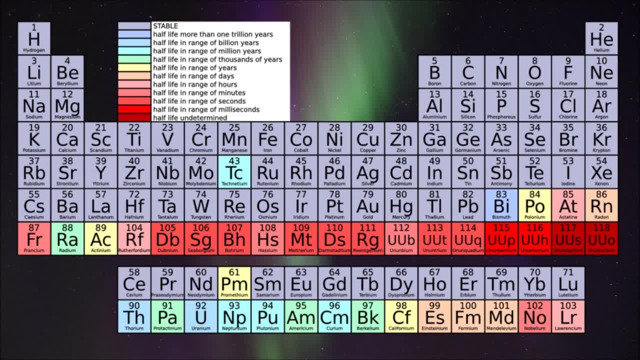 LR, Laurentium, RF Rutherfordium, DB, Dubnium, SG, Cyborgium, BH, Borium, HS, Hassium, MT, Mitnerium, DS, Darmstadium. RG. Runtinium CN. Copernicium UUT. Anuntrium FL. Florovium UUP. Anunpincium LV. Livermorium UUS- Anunseptium. UUO, Anunoxium, HHydrogen, HE, Helium, LI, Lithium, BE, Beryllium, BB, Boron, CC, Carbon, NNitrogen, OOxygen. 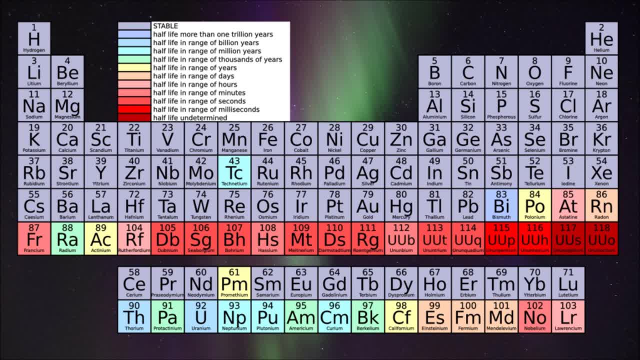 FFluorine, NE, Neon, NA, Sodium, MG, Magnesium, AL, Aluminum, SI, Silicon, PP, Phosphorus, SSulfur, CL, Chlorine, AR, Argon. 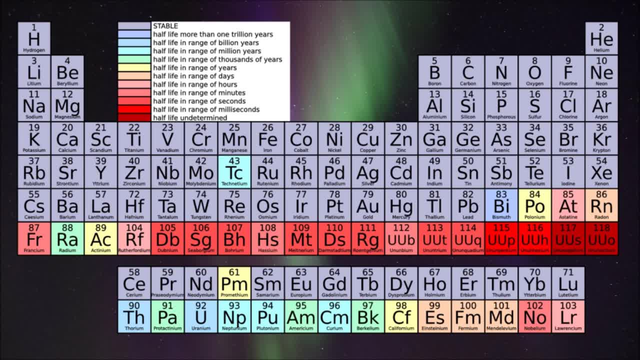 KK, Potassium, CA, Calcium, SC, Scandium, TI, Titanium, VVanadium, CR, Chromium, MN, Manganese, FE, Iron, CO, Cobalt, NI, Nickel. 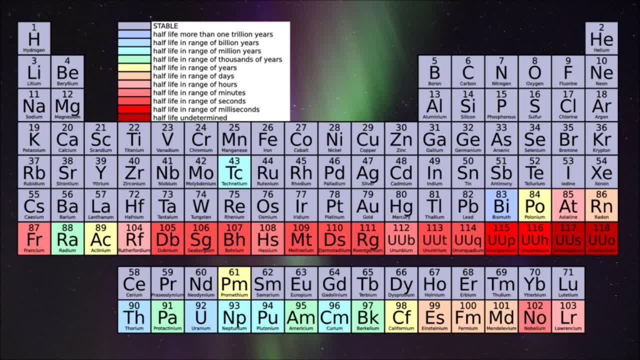 CU, Copper, ZN, Zinc, GA, Gallium, GE, Germanium, AS, Arsenic, SE, Selenium, BR, Bromine, KR, Krypton, RB, Rubidium. 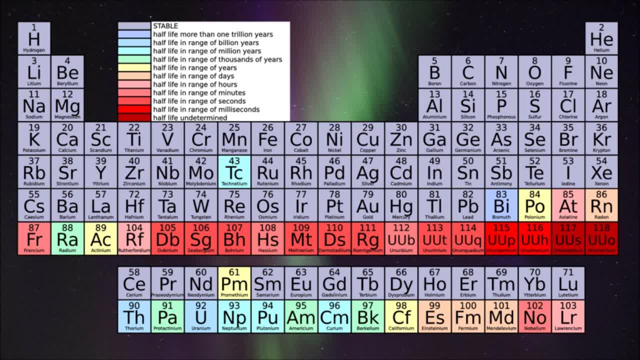 SR Strontium, Y Yttrium, ZR Zirconium, NB, Niobium, MO, Molybdenum, TC Technetium RU Ruthenium. 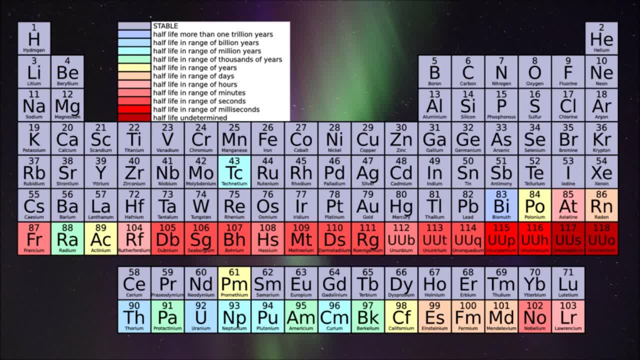 RH, Rhodium, PD, Palladium, AG, Silver, CD, Cadmium IN Indium, SN, Tin, SB, Antimony, TE, Tellurium I, Iodine. 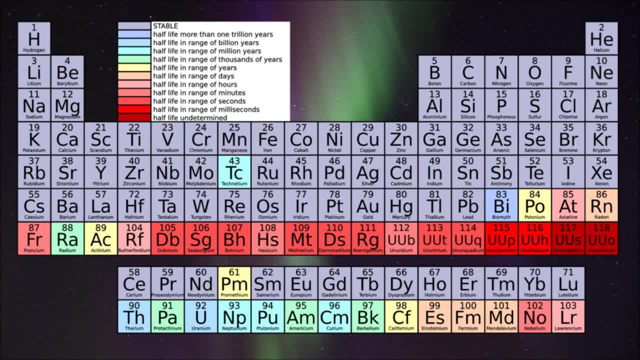 XE, Xenon, CS, Cesium, BA, Barium, LA, Lanthanum, CE, Cerium, PR, Praseodynium, ND, Neodynium, PM, Promethium. 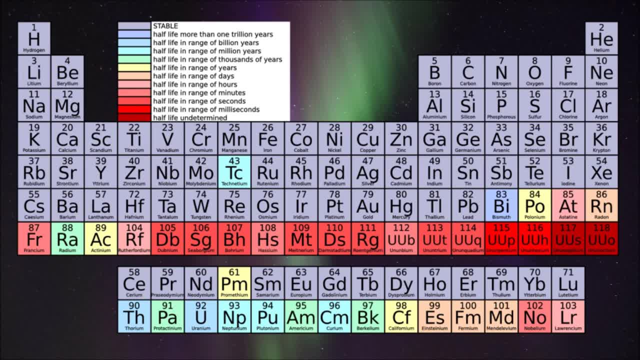 SM Cimmerium EU, Europium GD. Gadolinium TB Terbium DY. Dysprosium HO. Holmium ER Erbium TM Thulium. 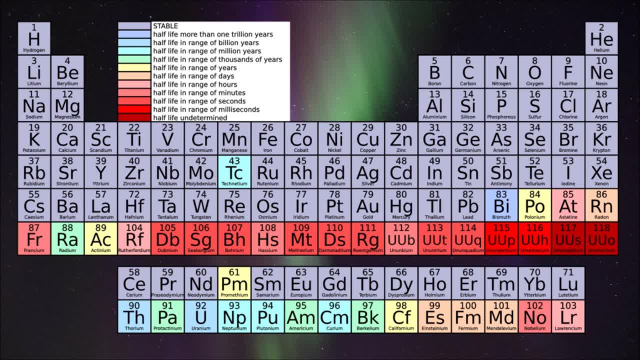 IR Iridium: PT, Platinum, AU, Gold, HG, Mercury, TL, Thallium, PB, Lead, BI, Bismuth, PO, Polonium, AT Astatine. 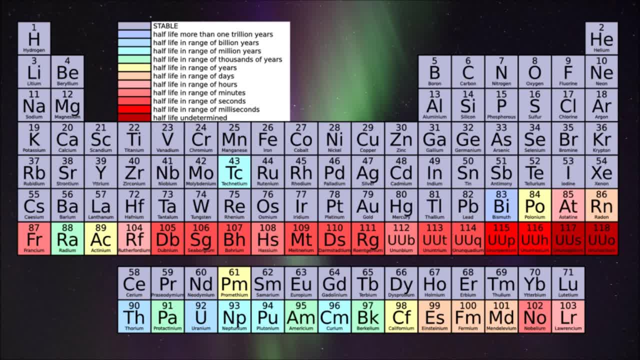 RN, Radon, FR, Francium, RA, Radium AC, Actinium, TH, Thorium, PA, Protactinium U, Uranium, NP, Neptunium, PU, Plutonium. AM, Emeritium, CM, Curium BK, Berkelium, CF. Californium, ES, Einsteinium, FM, Fermium, MD. Mendelevium, NO Nobelium. LR, Laurentium, RF Rutherfordium DB, Dubnium, SG, Cyborgium, BH, Borium, HS, Hacium, MT, Mitnerium, DS, Darmstadium. RG. Runtinium CN. Copernicium UUT. Anuntrium FL. Fluorovium UUP. Anunpincium LV. Livermorium UUS- Anunception. UUO Anunoxium H, Hydrogen, HE, Helium LI, Lithium BE, Beryllium, BE, Boron, CE, Carbon, NE, Nitrogen. 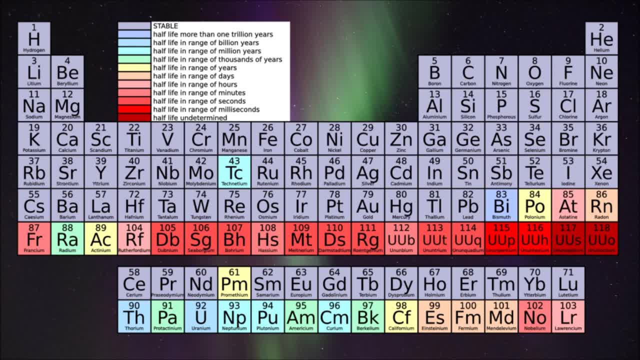 OE, Oxygen, FE, Fluorine, NE, Neon, NA, Sodium, MG, Magnesium, AL, Aluminum, SI, Silicon, P, Phosphorus S, Sulfur, CL, Chlorine. 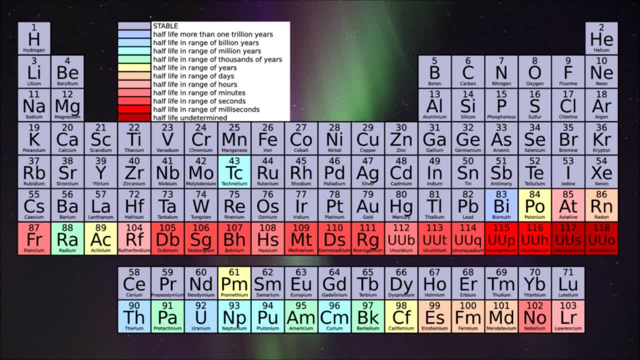 AR, Argon K, Potassium, CA, Calcium, SC, Scandium, TI, Titanium V, Vanadium, CR, Chromium, MN, Manganese, FE, Iron, CO, Cobalt. 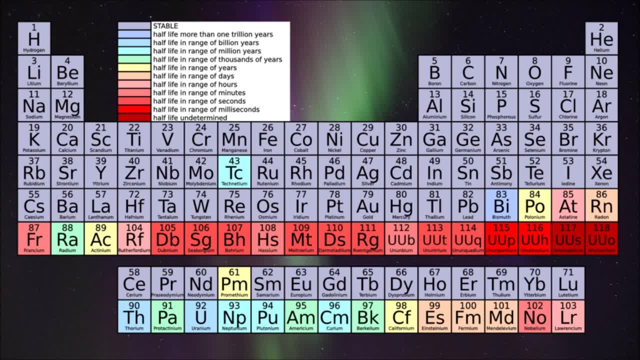 NI, Nickel, CU, Copper, ZN, Zinc, GA, Gallium, GE, Germanium, AS, Arsenic, SE, Selenium, BR, Bromine, KR, Krypton. 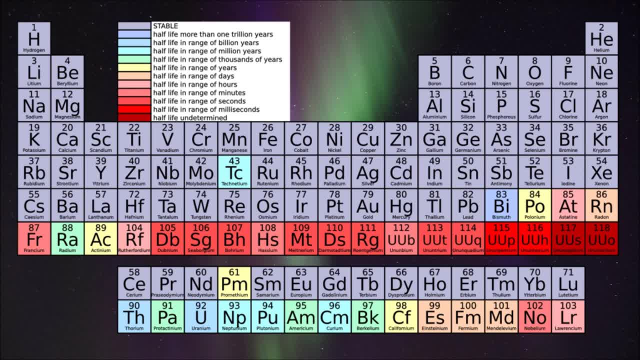 RB Rubidium, SR, Strontium, Y. Yttrium, ZR, Zirconium, NB, Niobium, MO, Molybdenum, TC. Technetium. 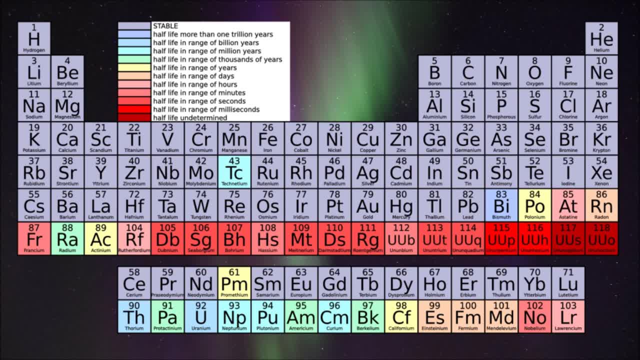 RU, Ruthenium, RH, Rhodium, PD, Palladium, AG, Silver, CD, Cadmium, IN Indium, SN, Tin, SB, Antimony ET Tellurium. 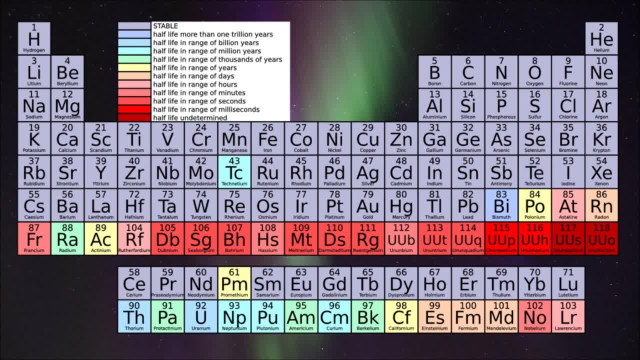 IIodon, XE, Xenon, CS, Cesium, BA, Barium, LA, Lanthanum, CE, Cerium, PR, Praseodynium, ND, Neodynium. 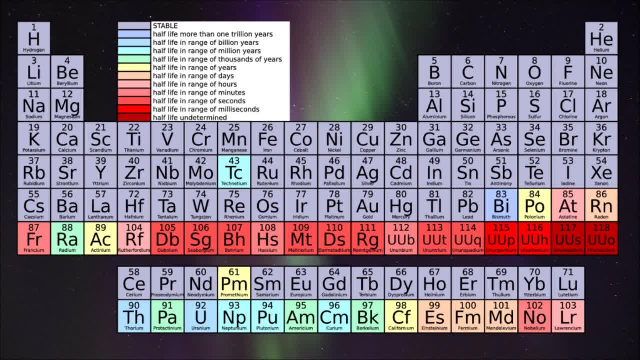 PM. Promethium, SM, Samarium, EU, Europium, GD, Gadolinium, TB, Terbium, DY, Dysprosium, HO, Holmium, ER, Erbium. 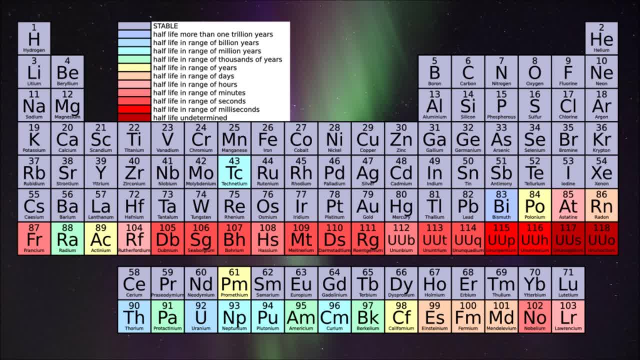 OS, Osmium, IR, Iridium, PT, Platinum, AU, Gold, HG, Mercury, TL, Thallium, PB, Lead, BI, Bismuth, PO, Polonium. 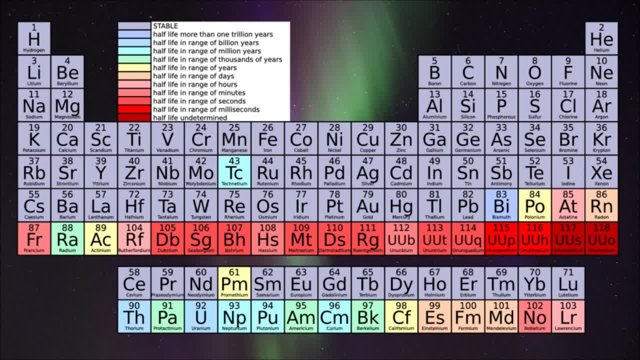 AT. Astatine, RN, Radon, FR, Francium, RA. Radium AC, Actinium, TH, Thorium, PA, Protactinium U, Uranium, NP, Neptunium. 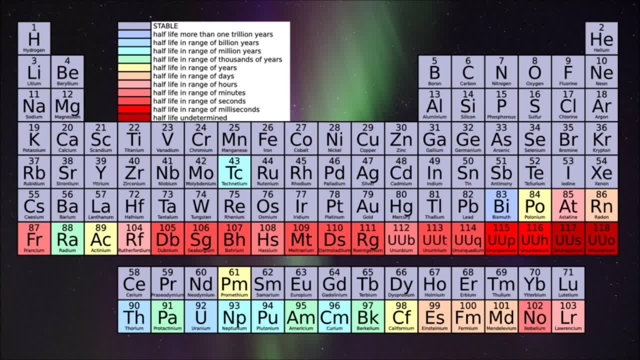 PU Plutonium, AM, Ameritium, CM, Curium BK, Berkelium, CF. Californium, ES, Einsteinium, FM, Fermium MD. Mendelevium. NO. Nobelium, LR, Laurentium, RF, Rutherfordium DB, Dubnium, SG, Cyborgium, BH, Borium, HS, Hassium, MT, Metnerium. DS: Darmstadium RG. Runtinium CN. Copernicium UUT- Anuntrium FL. Florovium UUP. Anunpincium LV- Livermorium. 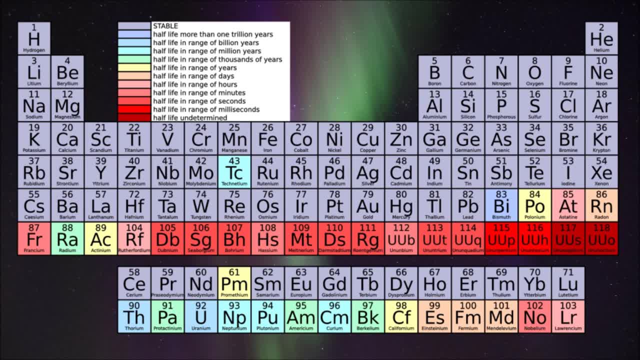 UUS, Anunseptium, UUO, Anunoxium HHydrogen, HE, Helium LI, Lithium BE, Beryllium, BB, Boron, CC, Carbon. 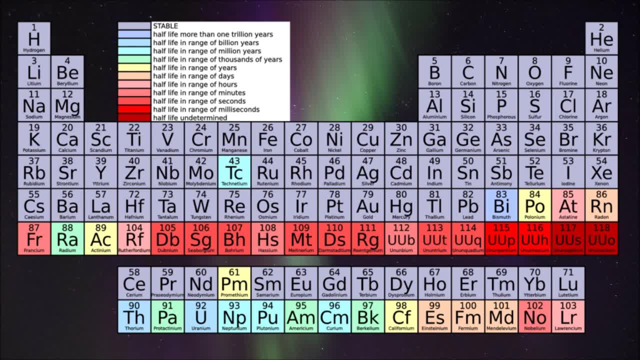 NNitrogen, OOxygen, FFluorine, NE, Neon, NA, Sodium, MG, Magnesium, AL, Aluminum, SI, Silicon, P, Phosphorus S, Sulfur. 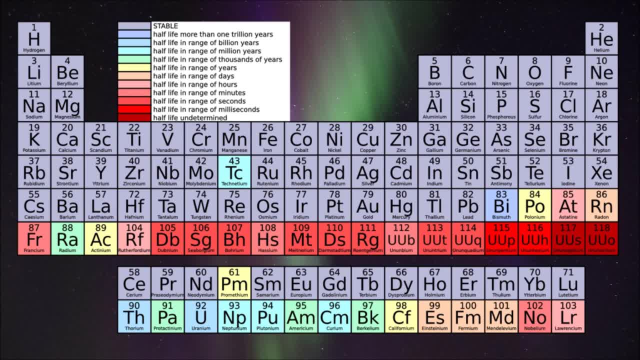 CL, Chlorine, AR, Argon K, Potassium, CA, Calcium, SC, Scandium, TI, Titanium V, Vanadium, CR, Chromium, MN, Manganese, FE, Iron. 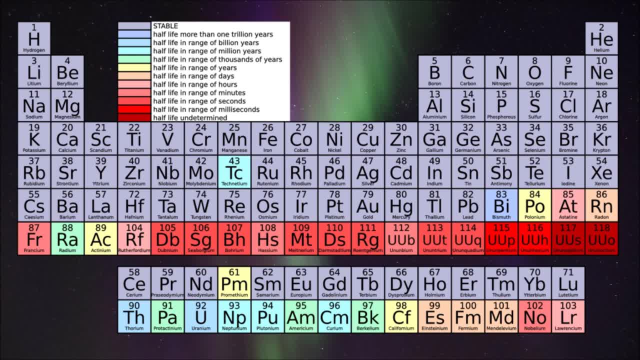 CO, Cobalt, NI, Nickel, CU Copper, ZN, Zinc, GA, Gallium, GE, Germanium, AS, Arsenic, SE, Selenium, BR, Bromine. 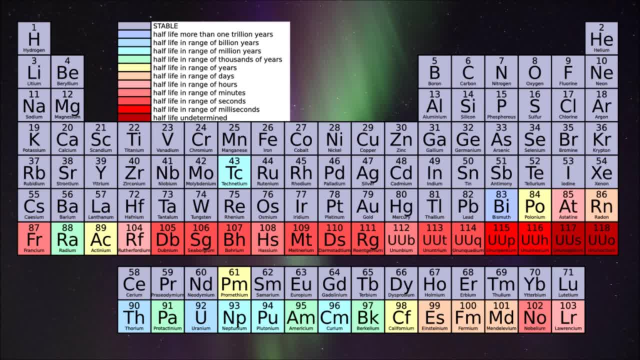 KR, Krypton, RB. Rubidium, SR, Strontium Y, Yttrium, ZR. Zirconium NB, Niobium, MO, Molybdenum, TC, Technetium. 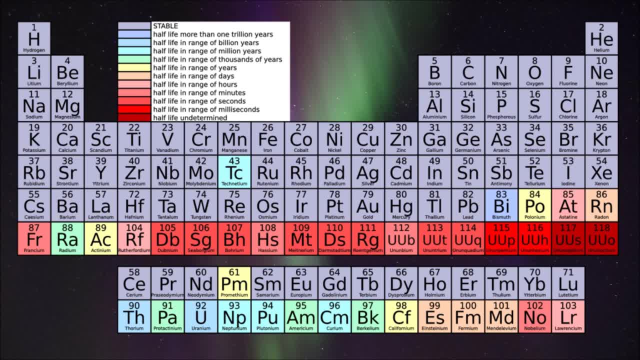 RU, Ruthenium, RH, Rhodium, PD, Palladium, AG, Silver, CD, Cadmium IN Indium, SN, Tin, SB, Antimony, TE Tellurium. 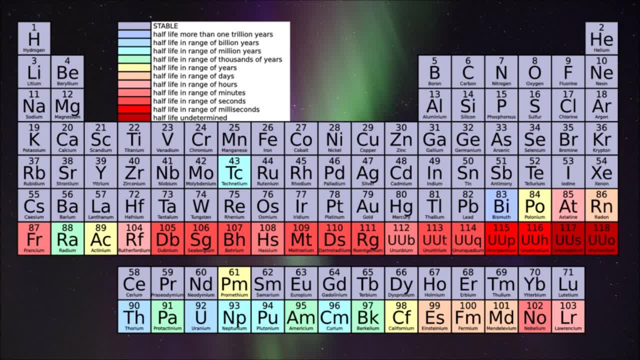 IIodon, XE, Xenon, CS, Cesium, BA, Barium, LA, Lanthanum, CE, Cerium, PR, Praseodynium, ND, Neodynium. 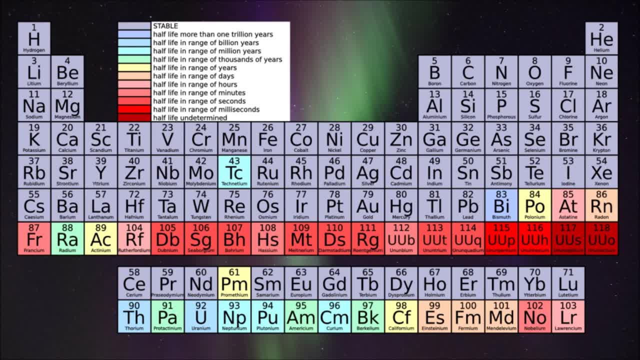 PM Promethium, SM, Cimmerium, EU, Europium GD, Gadolinium, TB, Terbium DY, Dysprosium, HO, Holmium ER, Erbium. TM Thulium YB. Ytterbium LU. Lutetium HF. Hafnium TA. Tantalum W Tungsten RE Rhenium. 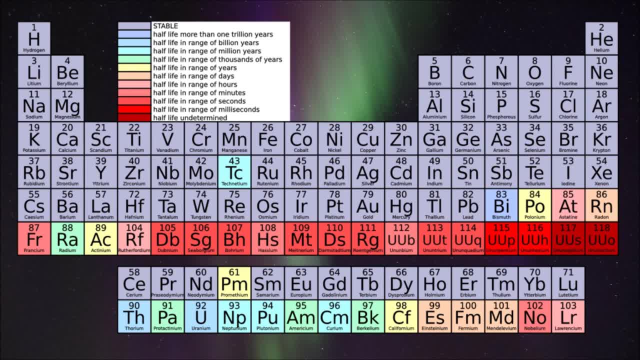 OS, Osmium, IR, Iridium, PT, Platinum, AU, Gold, HG, Mercury, TL, Thallium, PB, Lead, BI, Bismuth, PO, Polonium. 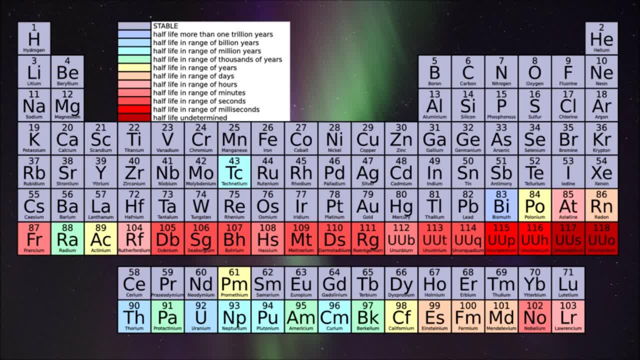 AT. Astatine, RN, Radon, FR, Francium, RA. Radium AC, Actinium, TH, Thorium, PA, Protactinium U, Uranium, NP, Neptunium. 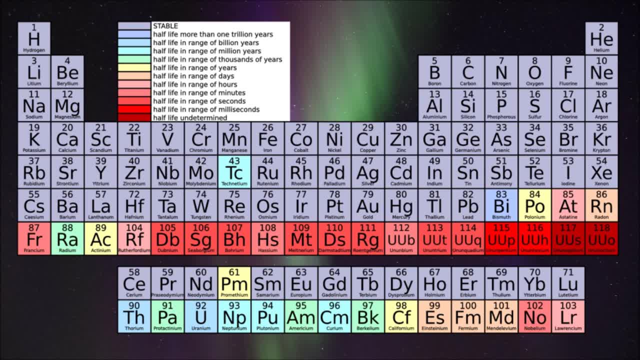 PU Plutonium, AM, Ameritium, CM, Curium BK, Berkelium, CF. Californium, ES, Einsteinium, FM, Fermium MD. Mendelevium. NO Nobellium, LR, Laurentium, RF, Rutherfordium, DB, Dubnium, SG, Cyborgium, BH, Borium, HS, Hassium, MT, Metneum. DM, Mirium, DS, Darmstadium RG, Runtinium, CN. Copernicium, UUT, Anuntrium FL. Florovium- UUP- Anunpincium. 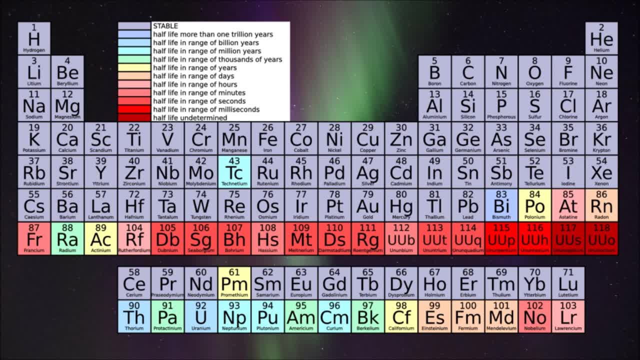 LV Livermorium UUS. Anunception UUO. Anunoxium HHydrogen HE, Helium LI, Lithium BE, Beryllium BB Boron. 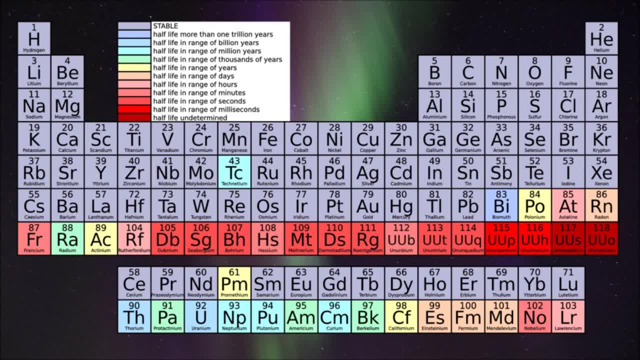 CC, Carbon, NNitrogen, OOxygen, FFluorine, NE, Neon, NA, Sodium, MG, Magnesium, AL, Aluminum, SI, Silicon, P, Phosphorus. 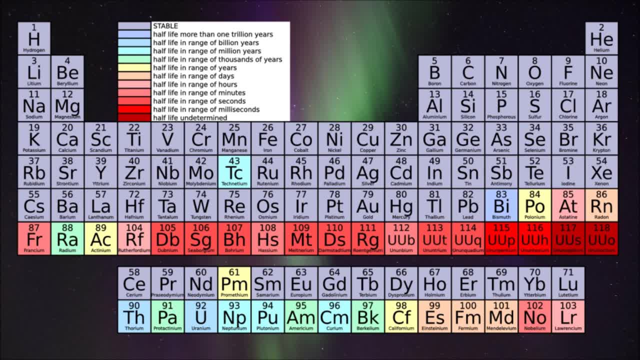 SSulfur, CL, Chlorine, AR, Argon K, Potassium, CA, Calcium, SC, Scandium TI, Titanium V, Vanadium CR, Chromium, MN, Manganese. 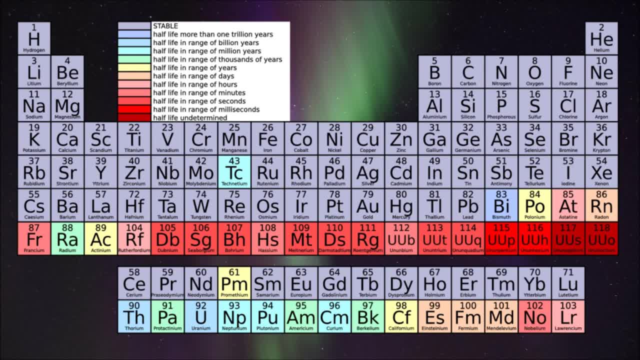 FE, Iron, CO Cobalt, NI Nickel, CU Copper, ZN, Zinc, GA, Gallium, GE, Germanium, AS, Arsenic, SE, Selenium, BR, Bromine. 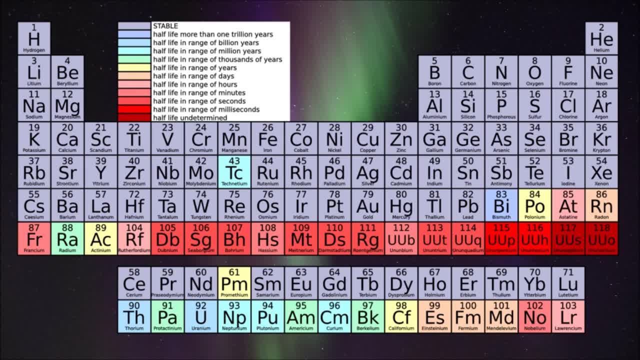 KR, Krypton, RB. Rubidium, SR, Strontium Y, Yttrium, ZR. Zirconium NB, Niobium, MO, Molybdenum, TC, Technetium. 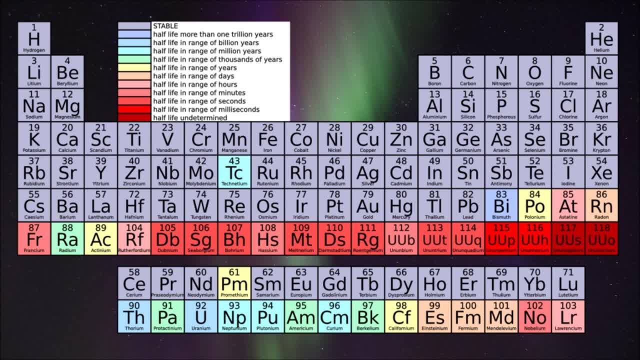 RU, Ruthenium, RH, Rhodium, PD, Palladium, AG, Silver, CD, Cadmium IN Indium, SN, Tin, SB, Antimony, TE Tellurium. 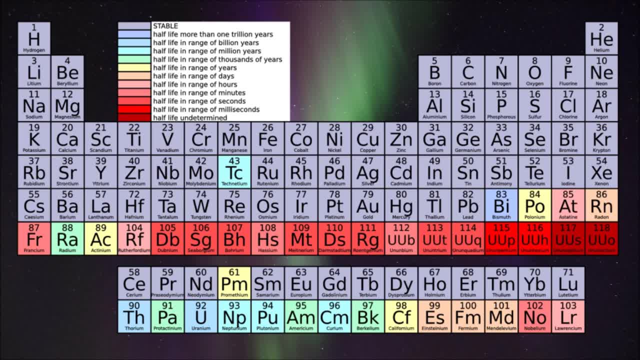 I. Iodine, XE, Xenon, CS, Cesium, BA, Barium, LA, Lanthanum, CE, Cerium, PR, Praseodynium, ND, Neodynium. 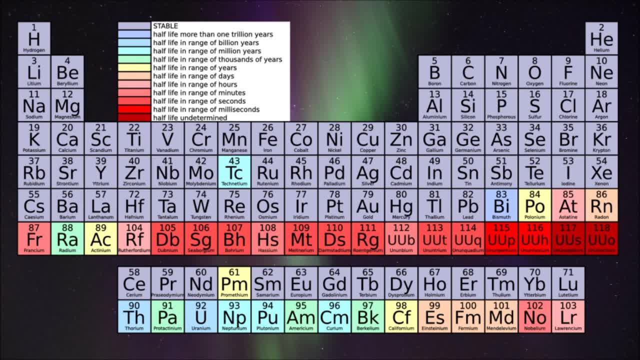 PM Promethium, SM, Cimmerium, EU, Europium GD, Gadolinium, TB, Terbium DY, Dysprosium, HO, Holmium ER, Erbium. TM Thulium YB. Ytterbium LU. Lutetium HF. Hafnium TA. Tantalum W Tungsten RE Rhenium. 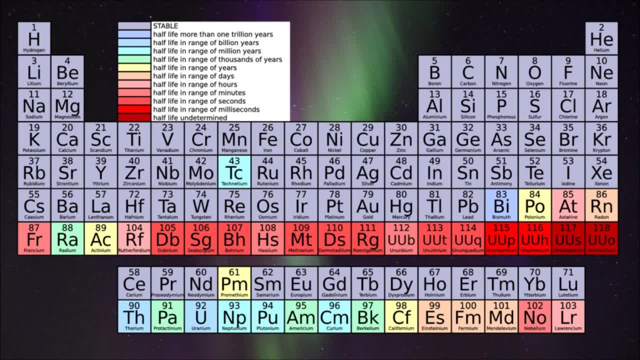 OS, Osmium, IR, Iridium, PT, Platinum, AU, Gold, HG, Mercury, TL, Thallium, PB, Lead, BI, Bismuth, PO, Polonium. 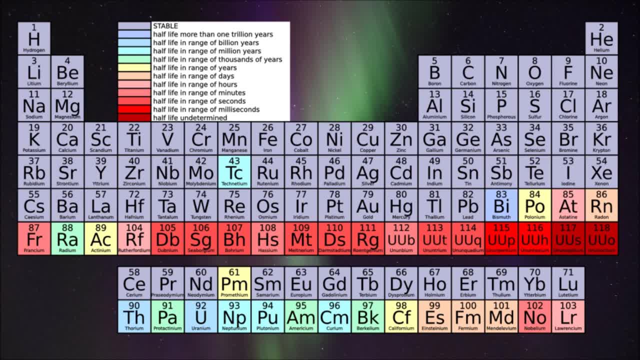 AT. Astatine, RN, Radon, FR, Francium, RA. Radium AC, Actinium, TH, Thorium, PA, Protactinium U, Uranium, NP, Neptunium. 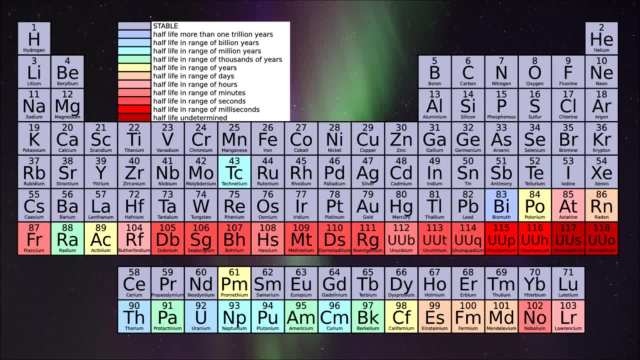 PU Plutonium, AM, Ameritium, CM, Curium BK, Berkelium, CF. Californium, ES, Einsteinium, FM, Fermium MD. Mendelevium. NO. Nobelium, LR, Laurentium, RF, Rutherfordium DB, Dubnium, SG, Cyborgium, BH, Borium HS, Hassium, MT, Mitnerium. DS: Darmstadium RG. Runtinium CN. Copernicium UUT- Anuntrium FL. Florovium UUP. Anunpincium LV- Livermorium. UUS, Anunseptium, UUO, Anunoxium: H, Hydrogen, HE, Helium LI, Lithium BE, Beryllium, BB, Boron, CC, Carbon. 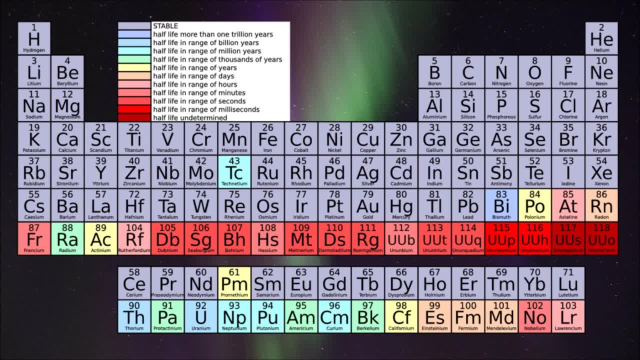 NNitrogen, OOxygen, FFluorine, NE, Neon, NA, Sodium, MG, Magnesium, AL, Aluminum, SI, Silicon, PP, Phosphorus, SS, Sulfur. 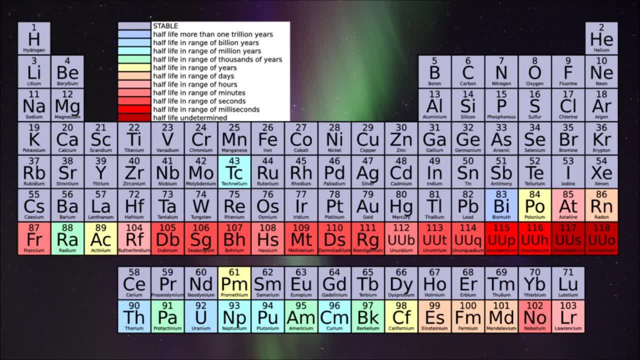 CL, Chlorine, AR, Argon, KK, Potassium, CA, Calcium, SC, Scandium, TI, Titanium, VVanadium, CR, Chromium, MN, Manganese. 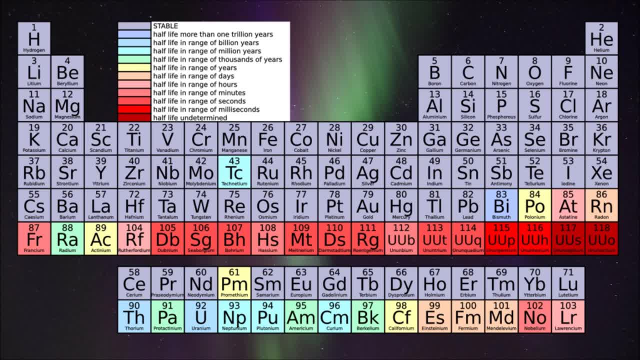 FE, Iron, CO Cobalt, NI Nickel, CU Copper, ZN, Zinc, GA, Gallium, GE, Germanium, AS, Arsenic, SE, Selenium, BR, Bromine. 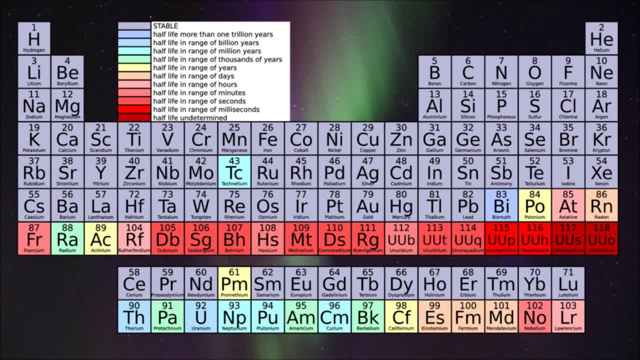 KR, Krypton, RB. Rubidium, SR, Strontium Y, Yttrium, ZR. Zirconium NB, Niobium, MO, Molybdenum, TC, Technetium. 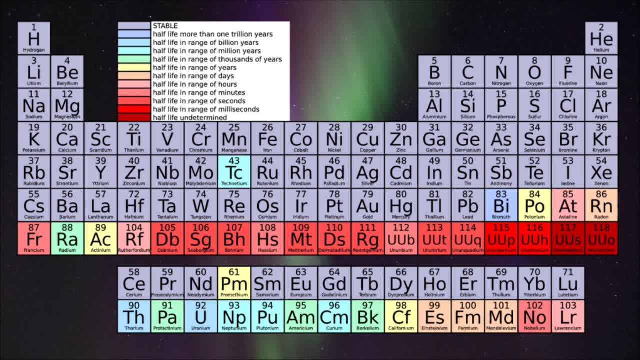 RU, Ruthenium, RH, Rhodium CD, Palladium, AG, Silver CD, Cadmium IN Indium, SN, Tin, SB, Antimony, TE Tellurium. 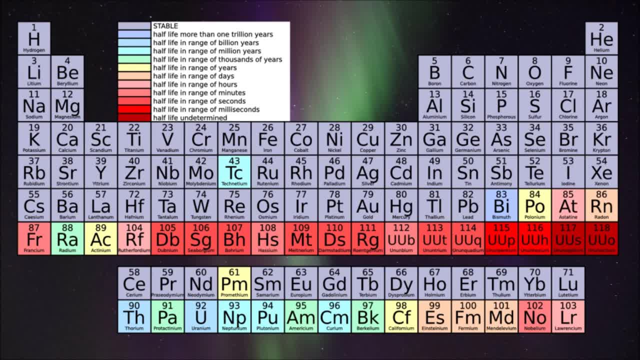 I, Iodon, XE, Xenon, CS, Cesium BA, Barium, LA, Lanthanum, CE, Cerium, PR, Praseodynium, ND, Neodynium. 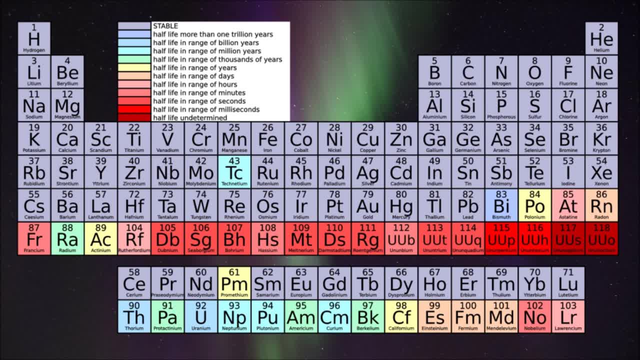 PM Promethium, SM, Cimmerium, EU, Europium GD, Gadolinium, TB, Terbium DY, Dysprosium, HO, Holmium ER, Erbium. TM Thulium YB. Ytterbium LU. Lutetium HF. Hafnium TA. Tantalum W Tungsten RE Rhenium. 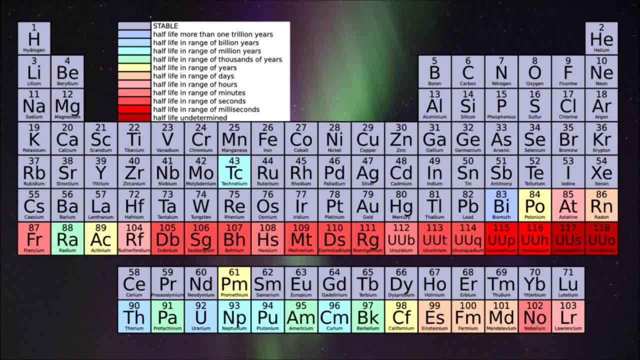 OS, Osmium, IR, Iridium, PT, Platinum, AU, Gold, HG, Mercury, TL, Thallium, PB, Lead, BI, Bismuth, PO, Polonium. 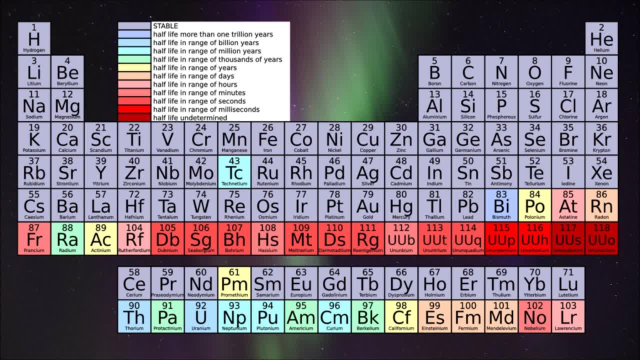 AT. Astatine, RN, Radon, FR, Francium, RA. Radium AC, Actinium, TH, Thorium, PA, Protactinium U, Uranium, NP, Neptunium. 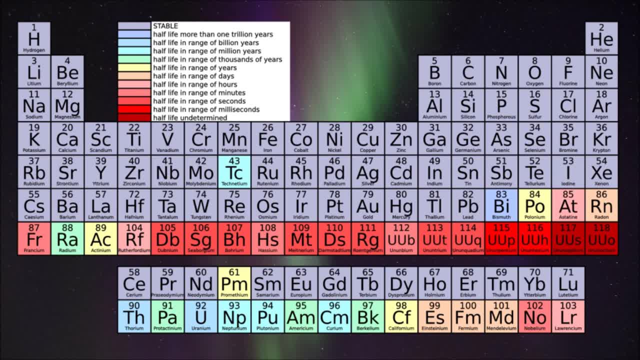 PU, Plutonium, AM, Emeritium, CM, Curium BK, Berkelium, CF. Californium, ES. Einsteinium, FM, Fermium MD. Mendelevium. 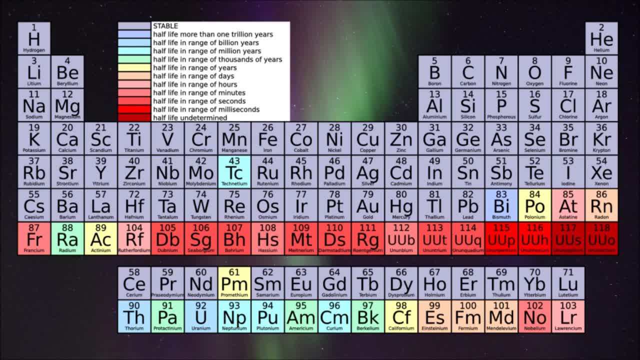 NE, Nitrogen, OE, Oxygen, FE, Fluorine, NE, Neon, NA, Sodium, MG, Magnesium, AL, Aluminum, SI, Silicon, P, Phosphorus S, Sulfur. 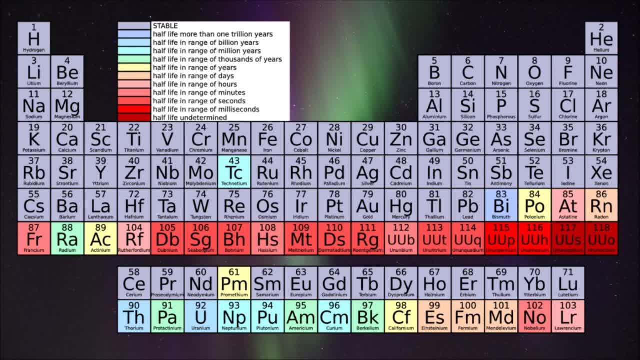 CL, Chlorine, AR, Argon K, Potassium, CA, Calcium, SC, Scandium, TI, Titanium V, Vanadium, CR, Chromium, MN, Manganese, FE, Iron. 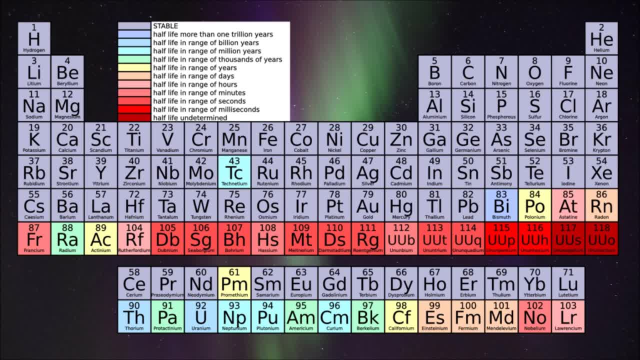 CO, Cobalt, NI, Nickel, CU Copper, ZN, Zinc, GA, Gallium, GE, Germanium, AS, Arsenic, SE, Selenium, BR, Bromine. 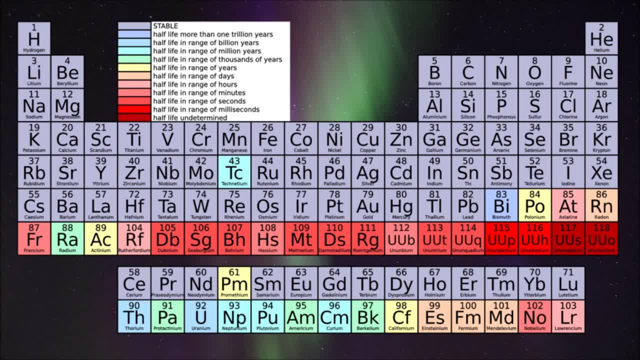 KR, Krypton, RB. Rubidium, SR, Strontium Y, Yttrium, ZR. Zirconium NB, Niobium, MO, Molybdenum, TC, Technetium. 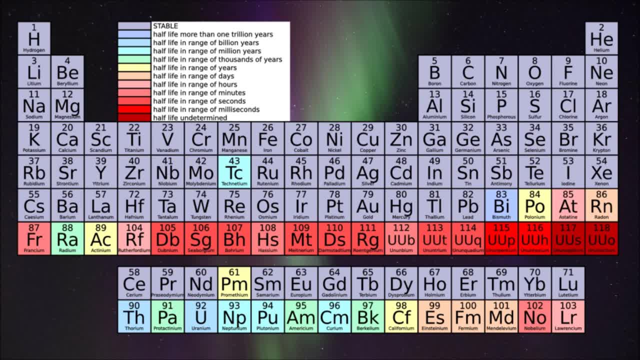 RU, Ruthenium, RH, Rhodium, PD, Palladium, AG, Silver, CD, Cadmium IN Indium, SN, Tin, SB, Antimony, CE, Tellurium. 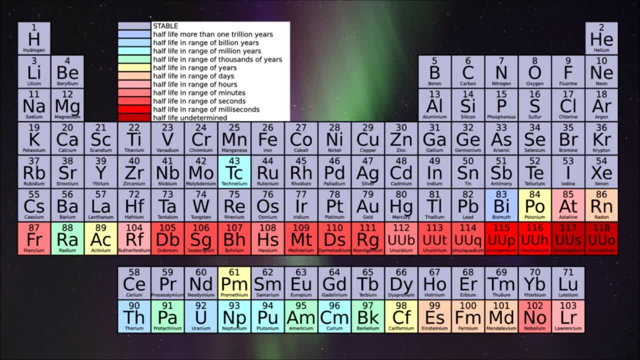 IIodon, XE, Xenon, CS, Cesium, BA, Barium, LA, Lanthanum, CE, Cerium, PR, Praseodynium, ND, Neodynium. 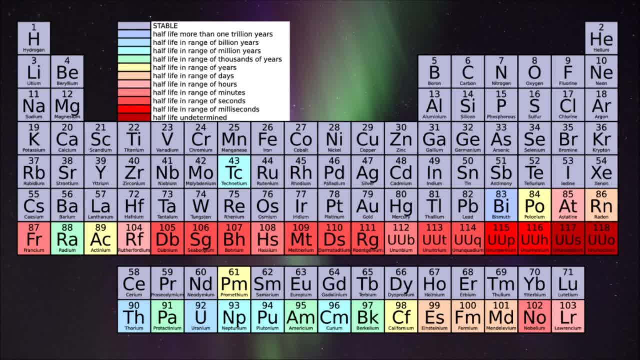 PM. Promethium, SM, Samarium, EU, Europium, GD, Gadolinium, TB, Terbium, DY, Dysprosium, HO, Holmium, ER, Erbium. TM Thulium YB. Ytterbium LU. Lutetium HF. Hafnium TA. Tantalum W Tungsten RE Rhenium. 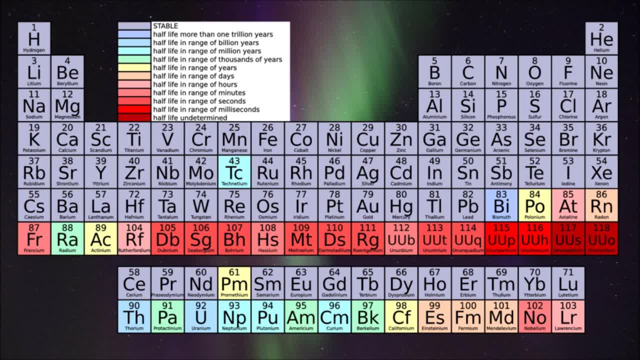 OS, Osmium, YR, Iridium, PT, Platinum, AU, Gold, HG, Mercury, TL, Thallium, PB, Lead, BI, Bismuth, PO, Polonium. 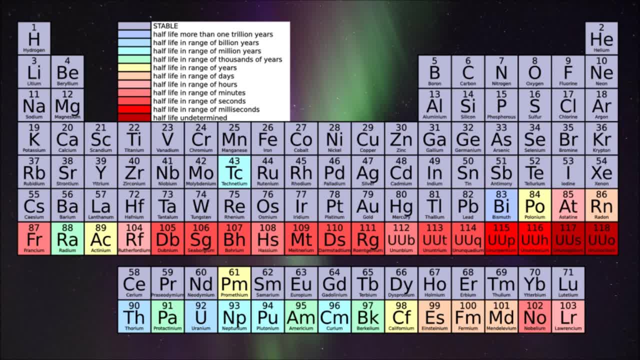 AT. Astatine, RN, Radon, FR, Francium, RA. Radium AC, Actinium, TH, Thorium, PA, Protactinium U, Uranium, NP, Neptunium. 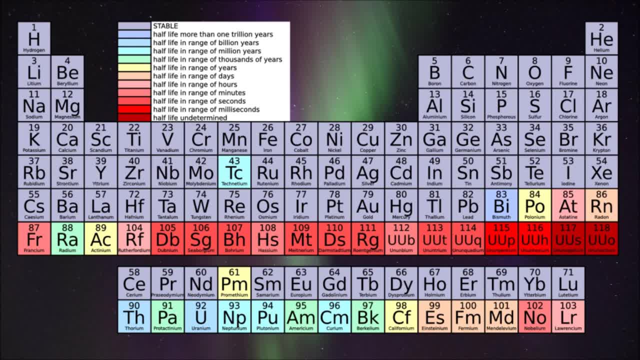 PU Plutonium, AM, Ameritium, CM, Curium BK, Berkelium, CF. Californium, ES, Einsteinium, FM, Fermium MD. Mendelevium. NO, Nobellium, LR, Laurentium, RF, Rutherfordium DB, Dubnium, SG, Cyborgium, BH, Borium, HS, Hassium, MT, Metnerium. DS: Darmstadium RG. Runtinium CN. Copernicium UUT- Anuntrium FL. Fluorovium UUP. Anunpincium LV- Livermorium. 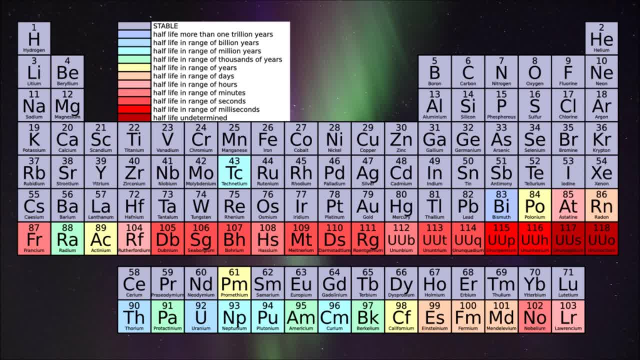 UUS Anunseption. UUO Anunoxium HHydrogen, HE, Helium LI, Lithium BE, Beryllium, BB, Boron, CC, Carbon. 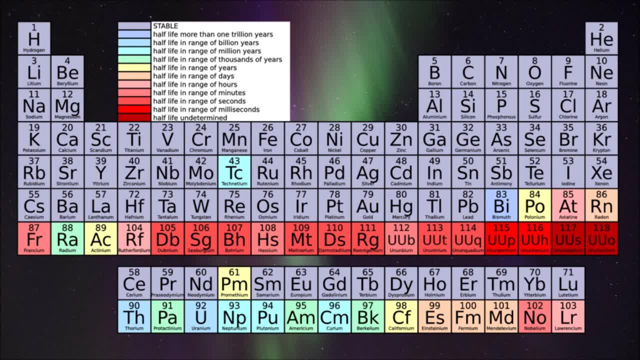 NNitrogen, OOxygen, FFluorine, NE, Neon, NA, Sodium, MG, Magnesium, AL, Aluminum, SI, Silicon, P, Phosphorus S, Sulfur. 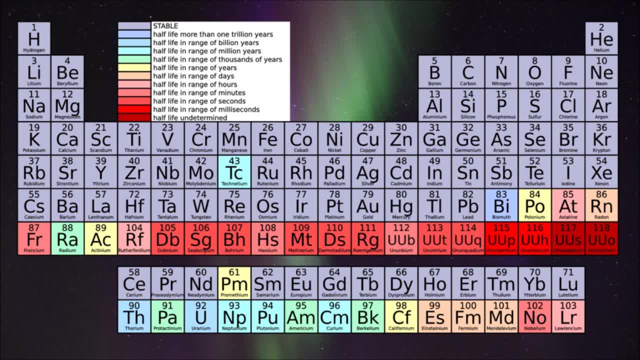 CL, Chlorine, AR, Argon K, Potassium, CA, Calcium, SC, Scandium, TI, Titanium V, Vanadium, CR, Chromium, MN, Manganese, FE, Iron. 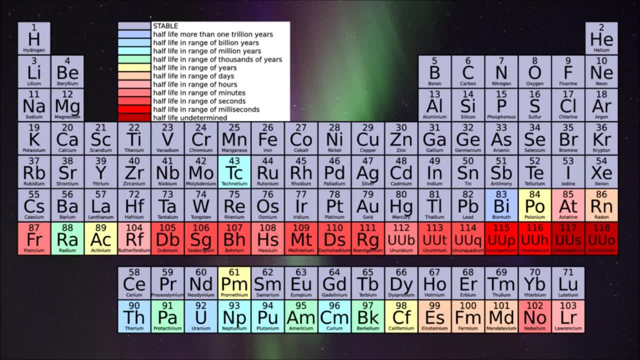 CO, Cobalt, NI, Nickel, CU Copper, ZN, Zinc, GA, Gallium, GE, Germanium, AS, Arsenic, SE, Selenium, BR, Bromine. 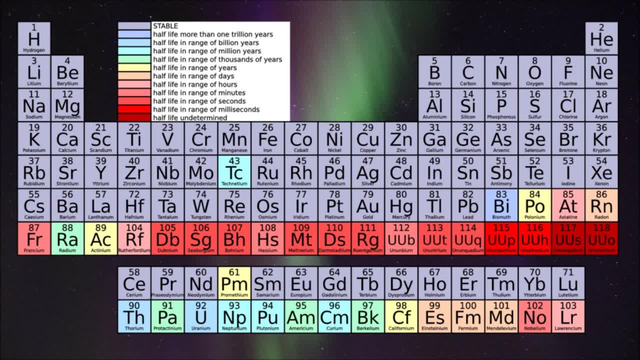 KR, Krypton, RB. Rubidium, SR, Strontium Y, Yttrium, ZR. Zirconium NB, Niobium, MO, Molybdenum, TC, Technetium. 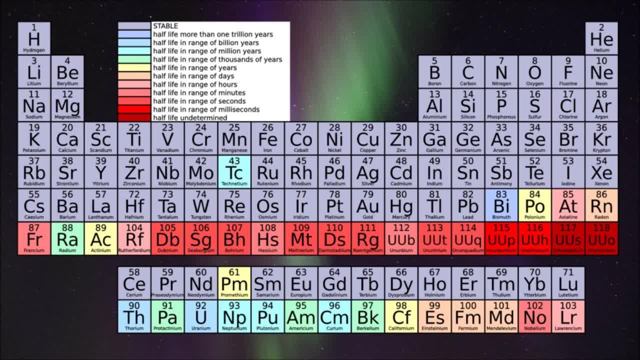 RU, Ruthenium, RH, Rhodium, PD, Palladium, AG, Silver, CD, Cadmium IN Indium, SN, Tin, SB, Antimony, TE Tellurium. 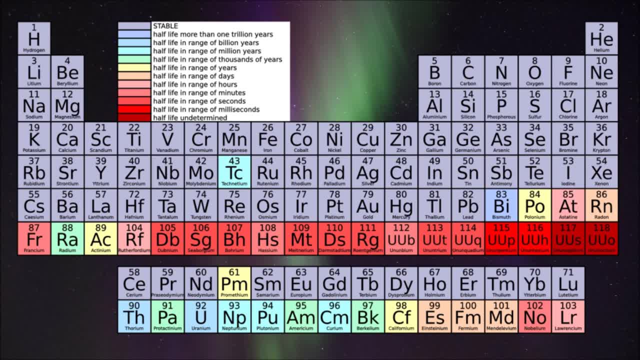 I, Iodon, XE, Xenon, CS, Cesium BA, Barium, LA, Lanthanum, CE, Cerium, PR, Praseodynium, ND, Neodynium. 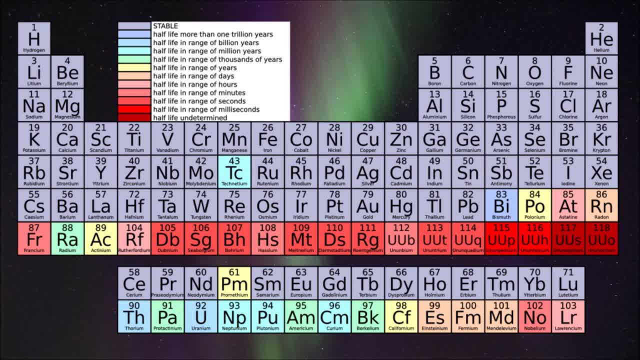 PM Promethium, SM, Cimmerium, EU, Europium GD, Gadolinium, TB, Terbium DY, Dysprosium, HO, Holmium ER, Erbium. TM Thulium YB. Ytterbium LU. Lutetium HF. Hafnium TA. Tantalum W Tungsten RE Rhenium. 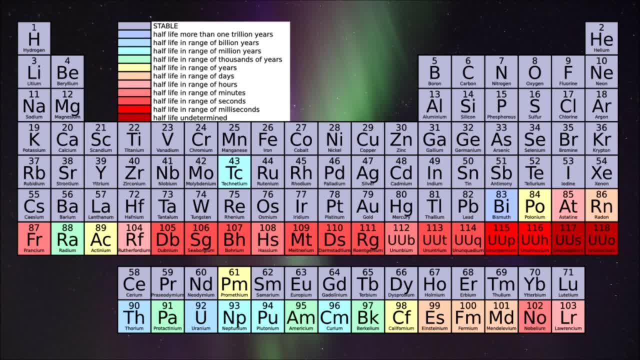 OS, Osmium, IR, Iridium, PT, Platinum, AU, Gold, HG, Mercury, TL, Thallium, PB, Lead, BI, Bismuth, PO, Polonium. 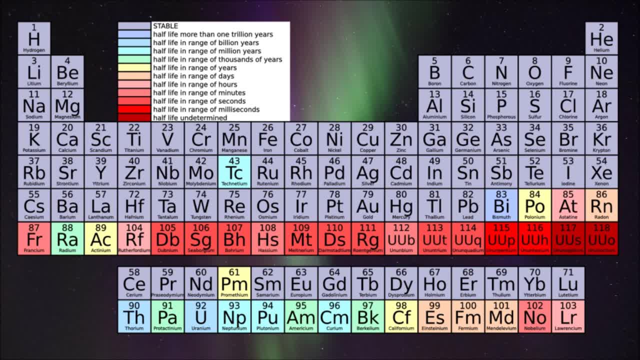 AT. Astatine, RN, Radon, FR, Francium, RA. Radium AC, Actinium, TH, Thorium, PA, Protactinium U, Uranium, NP, Neptunium. 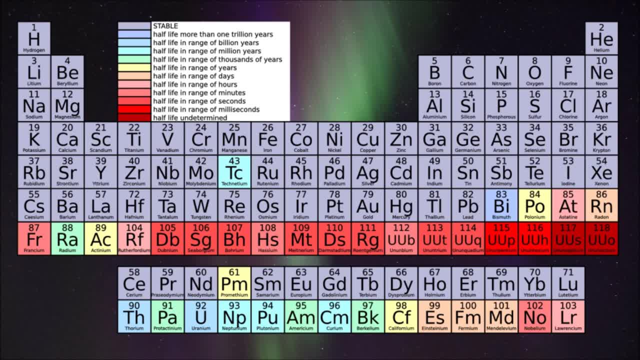 PU Plutonium, AM, Ameritium, CM, Curium BK, Berkelium, CF. Californium, ES, Einsteinium, FM, Fermium MD. Mendelevium. NO Nobellium, LR, Laurentium, RF, Rutherfordium DB, Dubnium, SG, Cyborgium, BH, Borium, HS, Hacium, MT, Mitnerium. DS: Darmstadium RG. Runtinium CN. Copernicium UUT- Anuntrium FL. Florovium UUP. Anunpincium LV- Livermorium. UUS, Anunseptium, UUO, Anunoxium: H, Hydrogen, HE, Helium LI, Lithium BE, Beryllium, BB, Boron, CC, Carbon. 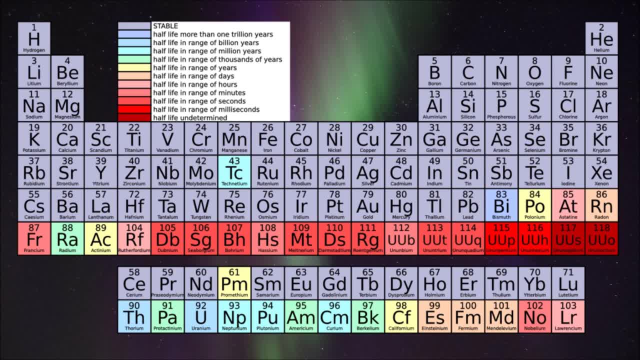 NNitrogen, OOxygen, FFluorine, NE, Neon, NA, Sodium, MG, Magnesium, AL, Aluminum, SI, Silicon, P, Phosphorus S, Sulfur. 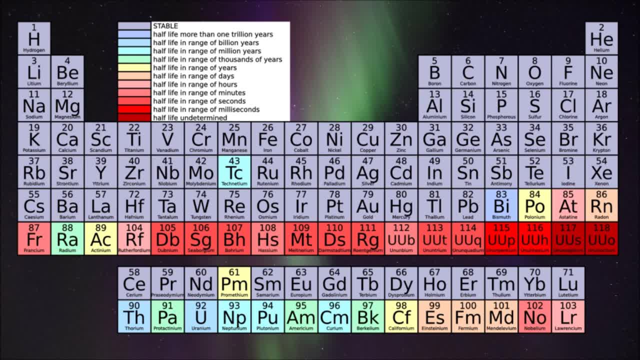 CL, Chlorine, AR, Argon, K, Potassium, CA, Calcium, SC, Scandium, TI, Titanium, VVanadium, CR, Chromium, MN, Manganese, FE, Iron. 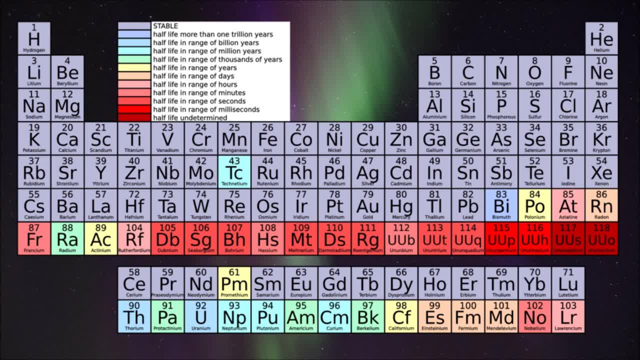 CO, Cobalt, NI, Nickel, CU Copper, ZN, Zinc, GA, Gallium, GE, Germanium, AS, Arsenic, SE, Selenium, BR, Bromine. 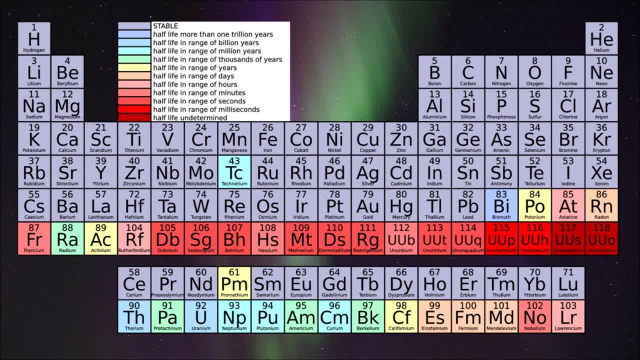 KR, Krypton, RB. Rubidium, SR, Strontium Y, Yttrium, ZR. Zirconium NB, Niobium, MO, Molybdenum, TC, Technetium. 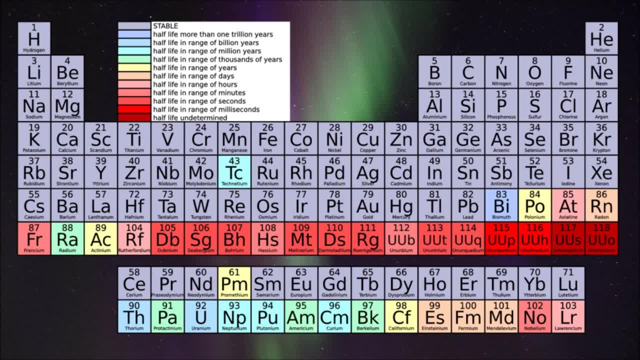 RU, Ruthenium, RH, Rhodium, PD, Palladium, AG, Silver, CD, Cadmium IN Indium, SN, Tin, SB, Antimony, TE Tellurium. 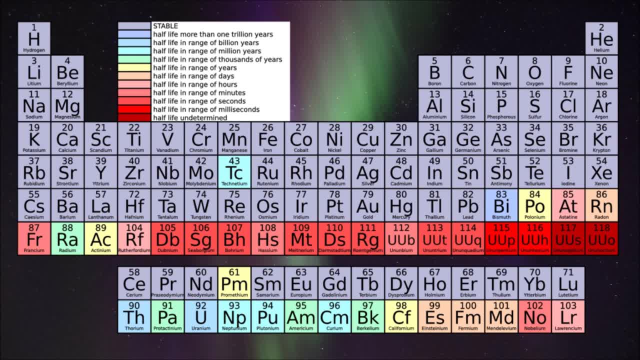 I. Iodine, XE, Xenon, CS, Cesium, BA, Barium, LA, Lanthanum, CE, Cerium, PR, Praseodynium, ND, Neodynium. 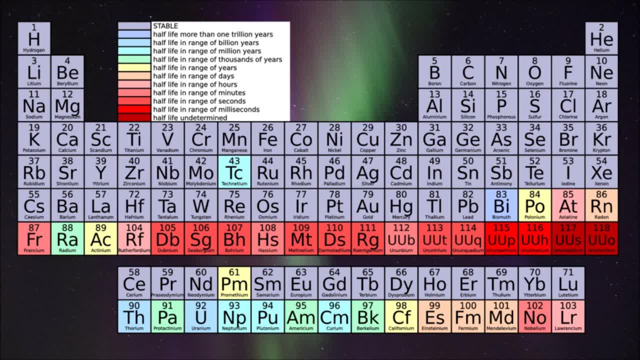 PM Promethium, SM, Cimmerium, EU, Europium GD, Gadolinium, TB, Terbium DY, Dysprosium, HO, Holmium ER, Erbium. TM Thulium YB. Ytterbium LU. Lutetium HF. Hafnium TA. Tantalum W Tungsten RE Rhenium. 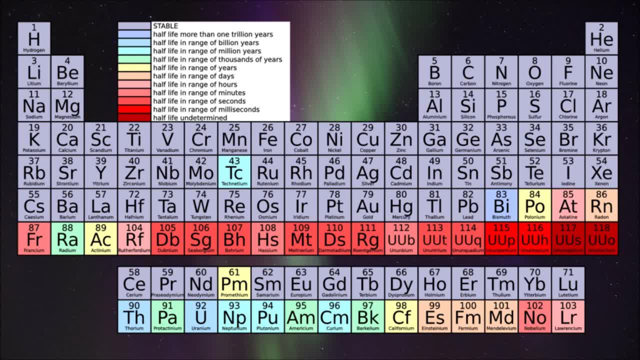 OS, Osmium, IR, Iridium, PT, Platinum, AU, Gold, HG, Mercury, TL, Thallium, PB, Lead, BI, Bismuth, PO, Polonium. 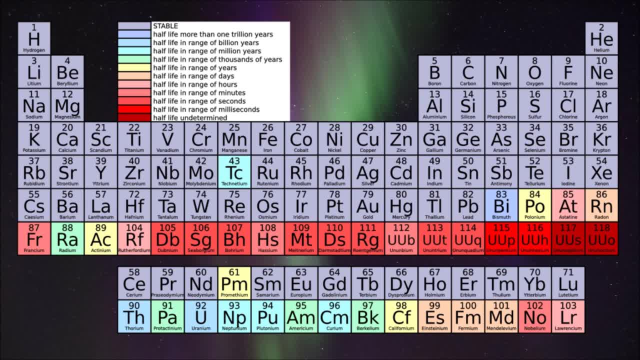 AT. Astatine, RN, Radon, FR, Francium, RA. Radium AC, Actinium, TH, Thorium, PA, Protactinium U, Uranium, NP, Neptunium. 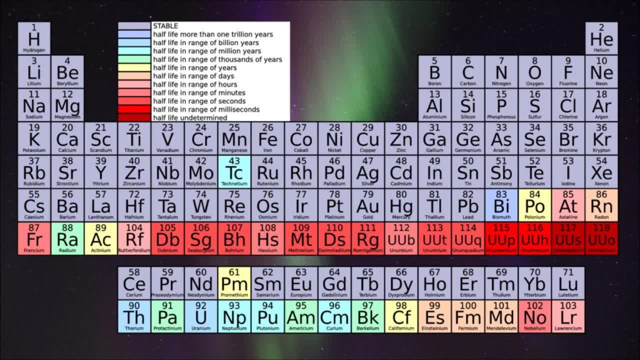 PU, Plutonium, AM, Emeritium, CM, Curium BK, Berkelium, CF. Californium, ES. Einsteinium, FM, Fermium MD. Mendelevium. NO. Nobelium, LR, Laurentium, RF, Rutherfordium DB, Dubnium, SG, Cyborgium, BH, Borium, HS, Hacium, MT, Mitnerium. DS: Darmstadium RG. Runtinium CN. Copernicium UUT- Anuntrium FL. Fluorovium UUP. Anunpincium LV- Livermorium. UUS, Anunseptium, UUO, Anunoxium: H, Hydrogen, HE, Helium LI, Lithium BE, Beryllium BE, Boron, CE, Carbon. 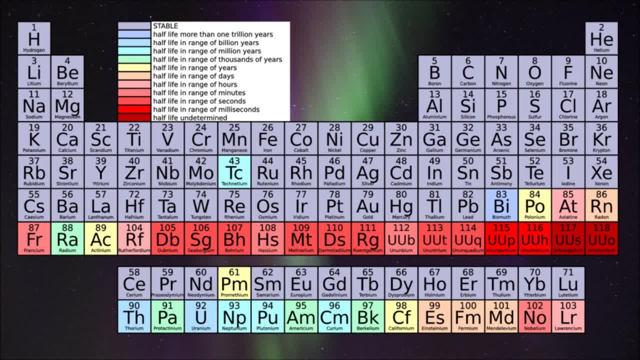 NE, Nitrogen, OE, Oxygen, FE, Fluorine, NE, Neon, NA, Sodium, MG, Magnesium, AL, Aluminum, SI, Silicon, P, Phosphorus S, Sulfur. 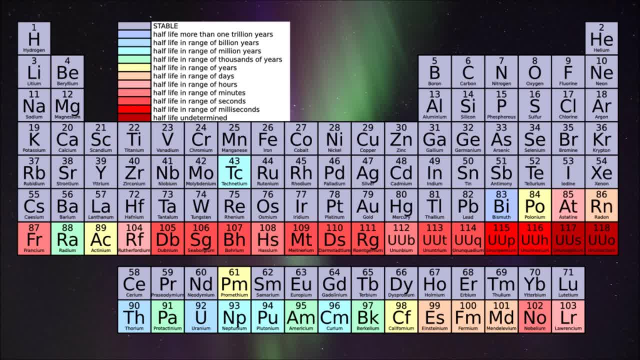 CL, Chlorine, AR, Argon K, Potassium, CA, Calcium, SC, Scandium, TI, Titanium V, Vanadium, CR, Chromium, MN, Manganese, FE, Iron. 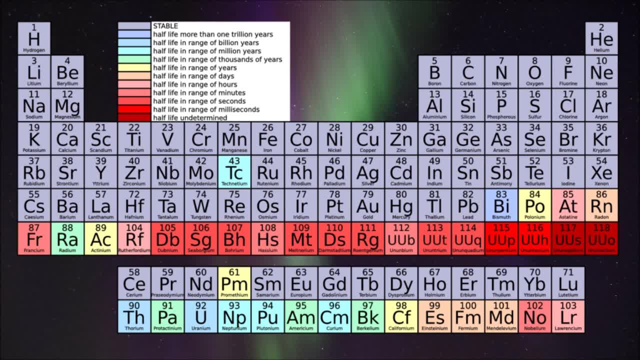 CO, Cobalt, NI, Nickel, CU Copper, ZN, Zinc, GA, Gallium, GE, Germanium, AS, Arsenic, SE, Selenium, BR, Bromine. 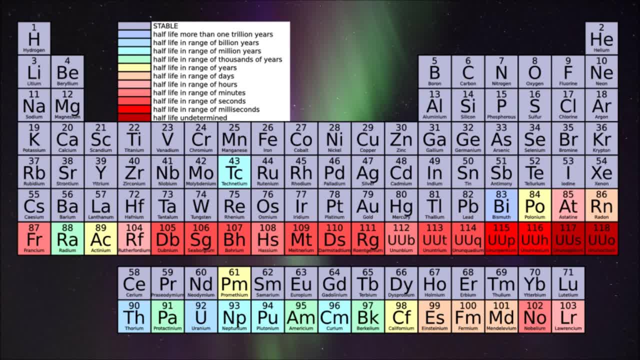 KR, Krypton, RB, Rubidium, SR, Strontium, Y, Yttrium, ZR, Zirconium, NB, Niobium, MO, Molybdenum, TC, Technesium. 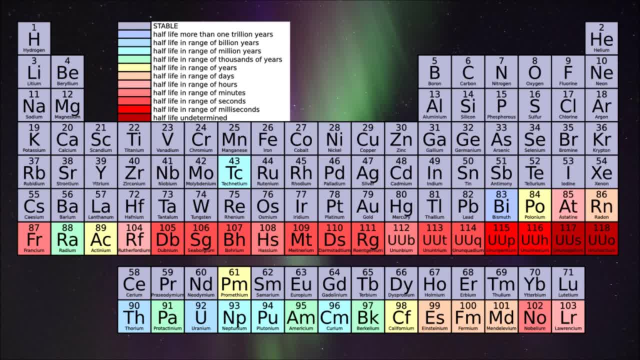 RU, Ruthenium, RH, Rhodium, PD, Palladium, AG, Silver, CD, Cadmium IN Indium, SN, Tin, SB, Antimony, TE Tellurium. 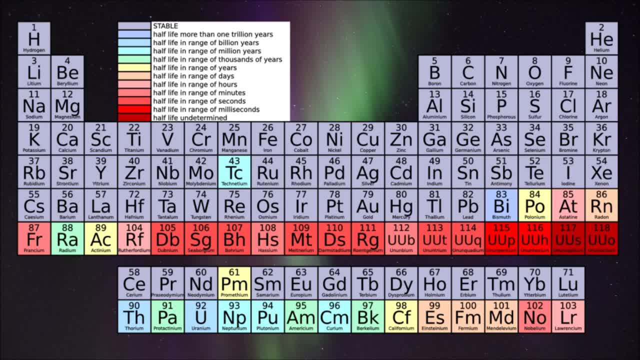 I. Iodine, XE, Xenon, CS, Cesium, BA, Barium, LA, Lanthanum, CE, Cerium, PR, Praseodynium, ND, Neodynium. 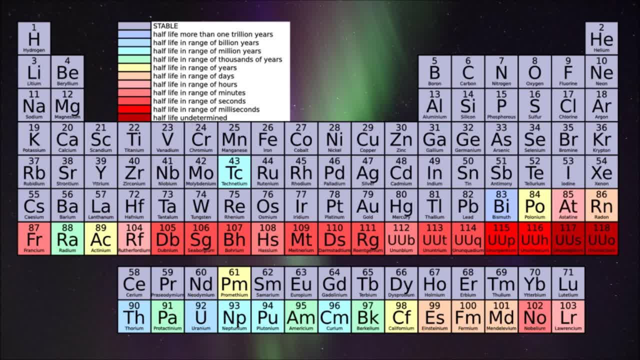 PM. Promethium, SM, Samarium, EU, Europium, GD, Gadolinium, TB, Terbium, DY, Dysprosium, HO, Holmium, ER, Erbium. TM Thulium YB. Yterbium LU. Lutetium HF. Hafnium TA. Tantalum W Tungsten RE Rhenium. 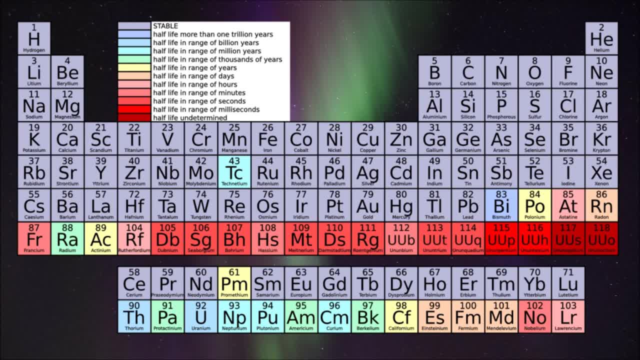 OS, Osmium, IR, Iridium, PT, Platinum, AU, Gold, HG, Mercury, TL, Thallium, PB, Lead, BI, Bismuth, PO, Polonium. 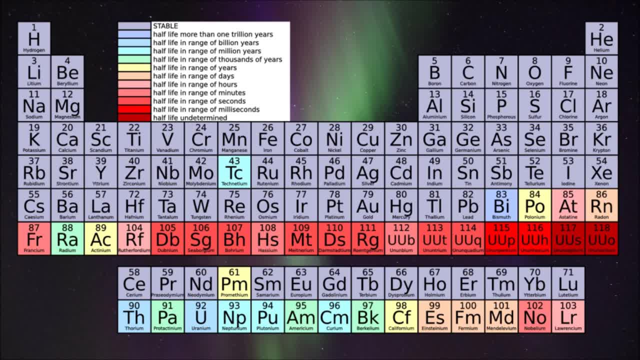 AT. Astatine, RN, Radon, FR, Francium, RA. Radium AC, Actinium, TH, Thorium, PA, Protactinium U, Uranium, NP, Neptunium. 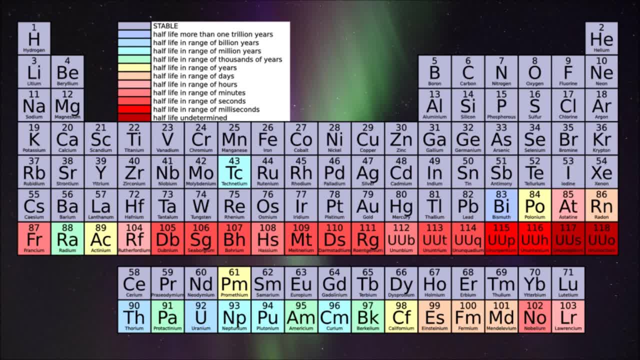 PU, Plutonium, AM, Emeritium, CM, Curium BK, Berkelium, CF. Californium, ES. Einsteinium, FM, Fermium MD. Mendelevium. NO. Nobelium, LR, Laurentium, RF, Rutherfordium DB, Dubnium, SG, Cyborgium, BH, Borium, HS, Hacium, MT, Metnerium. DS: Darmstadium RG. Runtinium CN. Copernicium UUT- Anuntrium FL. Fluorovium UUP. Anunpincium LV- Livermorium. 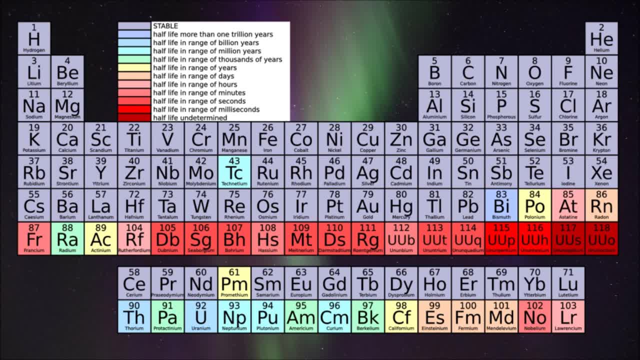 UUS Anunseption- UUO Anunoxium H, Hydrogen HE, Helium LI, Lithium BE, Beryllium BE, Boron C Carbon. N, Nitrogen O, Oxygen F, Fluorine, NE, Neon, NA, Sodium, MG, Magnesium, AL, Aluminum, SI, Silicon, P, Phosphorus S, Sulphur. 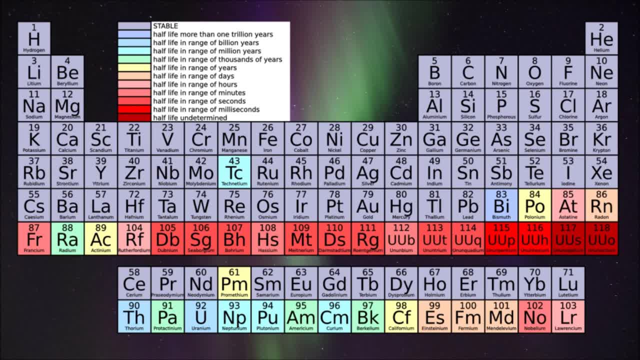 CL, Chlorine, AR, Argon K, Potassium, CA, Calcium, SC, Scandium, TI, Titanium V, Vanadium, CR, Chromium, MN, Manganese, FE, Iron. 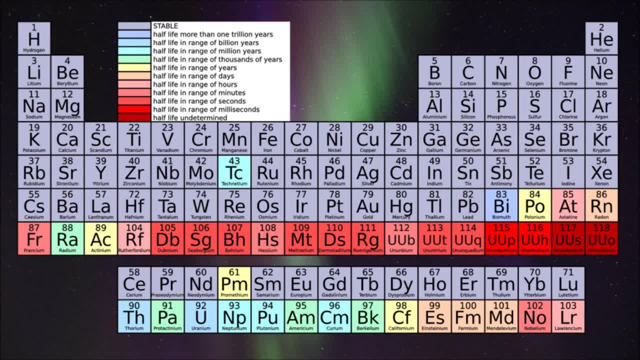 CO, Cobalt, NI, Nickel, CU Copper, ZN, Zinc, GA, Gallium, GE, Germanium, AS, Arsenic, SE, Selenium, ER Bromine. 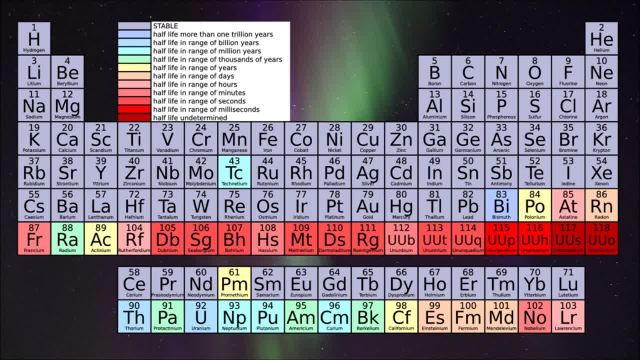 KR. Krypton, RB. Rubidium, SR, Strontium, Y. Yttrium, ZR. Zirconium, NB, Niobium, MO, Molybdenum, CC, Technetium. 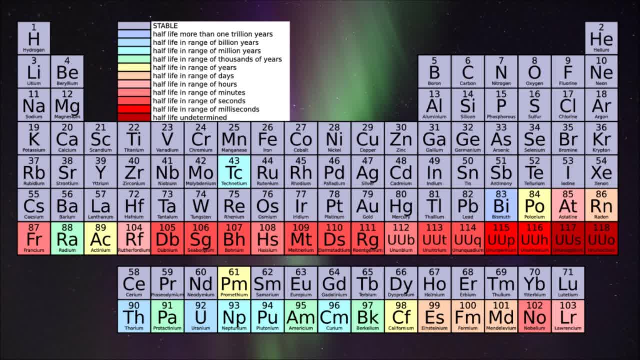 RU, Ruthenium, RH, Rhodium, PD, Palladium, AG, Silver, CD, Cadmium IN Indium, SN, Tin, SB, Antimony, TE Tellurium. 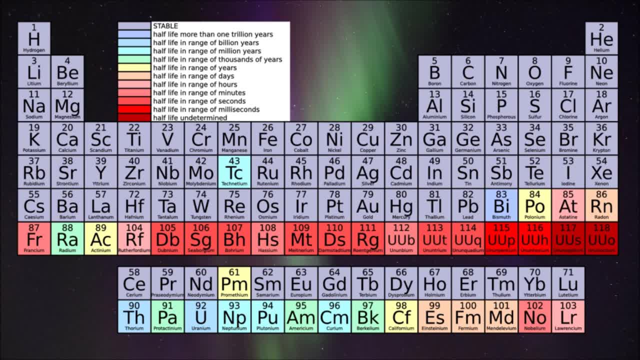 IIodon, XE, Xenon, CS, Cesium, BA, Barium, LA, Lanthanum, CE, Cerium, PR, Praseodynium, ND, Neodynium. 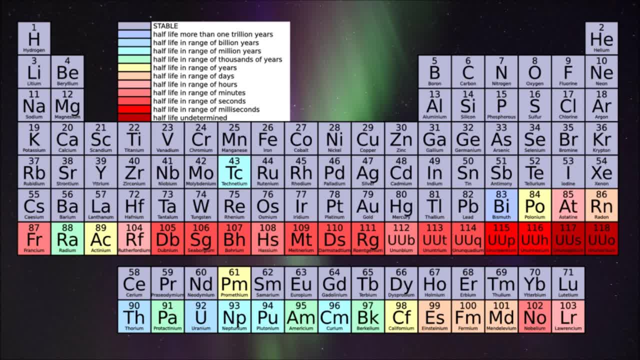 PM Promethium, SM, Cimmerium, EU, Europium GD, Gadolinium, TB, Terbium DY, Dysprosium, HO, Holmium ER, Erbium. TM Thulium YB. Ytterbium LU. Lutetium HF. Hafnium TA. Tantalum W Tungsten RE Rhenium. 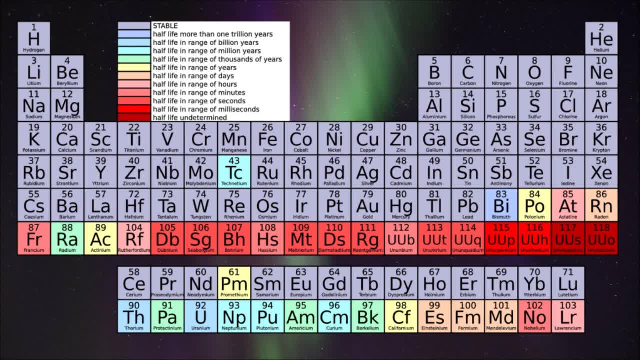 OS, Osmium, IR, Iridium, PT, Platinum, AU, Gold, HG, Mercury, TL, Thallium, PB, Lead, BI, Bismuth, PO, Polonium. 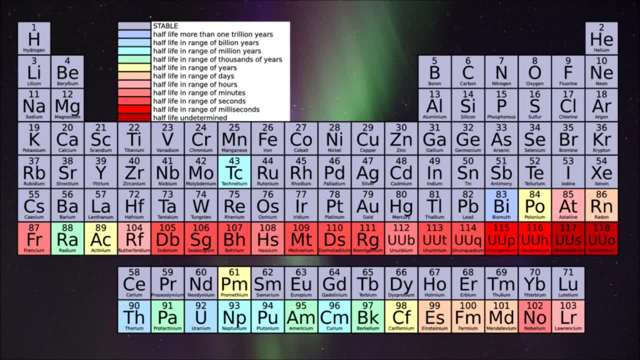 AT. Astatine, RN, Radon, FR, Francium, RA. Radium AC, Actinium, TH, Thorium, PA, Protactinium U, Uranium, NP, Neptunium. 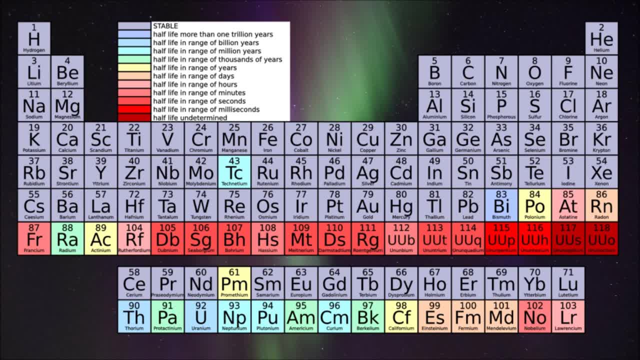 PU Plutonium, AM, Ameritium, CM, Curium BK, Berkelium, CF. Californium, ES, Einsteinium, FM, Fermium MD. Mendelevium. NO, Nobellium, LR, Laurentium, RF, Rutherfordium DB, Dubnium, SG, Cyborgium, BH, Borium, HS, Hassium, MT, Metnerium. DS: Darmstadium RG. Runtinium CN. Copernicium UUT- Anuntrium FL. Florovium UUP. Anunpincium LV- Livermorium. 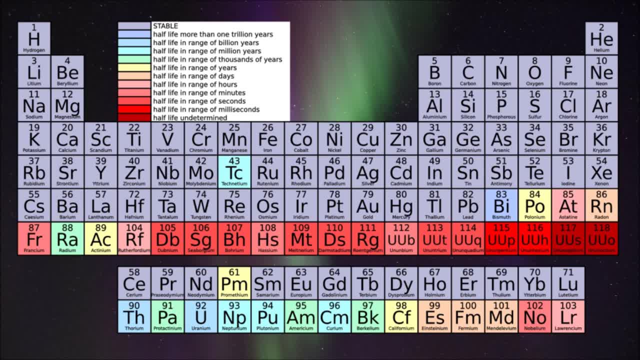 UUS, Anunseptium, UUO, Anunoxium HHydrogen, HE, Helium LI, Lithium BE, Beryllium, BB, Boron, CC, Carbon. 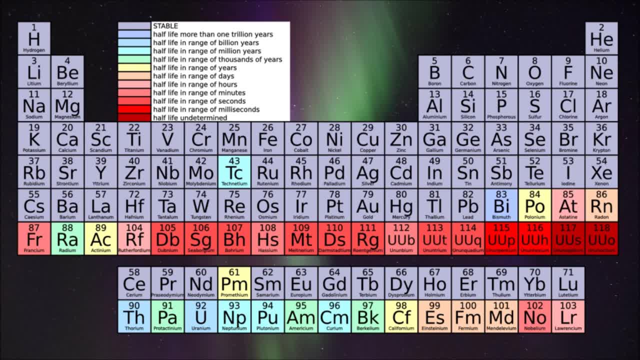 NNitrogen, OOxygen, FFluorine, NE, Neon, NA, Sodium, MG, Magnesium, AL, Aluminum, SI, Silicon, P, Phosphorus S, Sulfur. 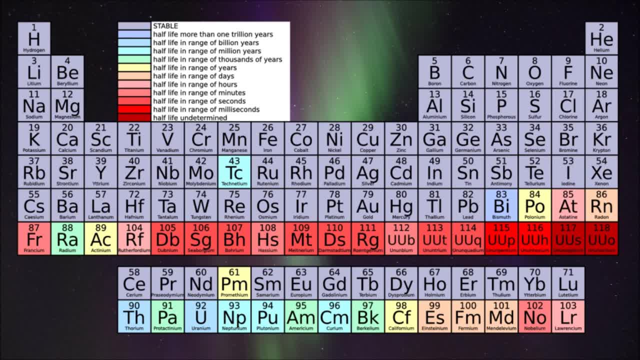 CL, Chlorine, AR, Argon K, Potassium, CA, Calcium, SC, Scandium, TI, Titanium V, Vanadium, CR, Chromium, MN, Manganese, FE, Iron. 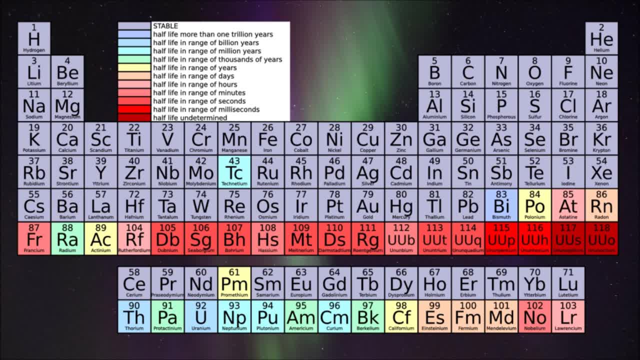 CO, Cobalt, NI, Nickel, CU Copper, ZN, Zinc, GA, Gallium, GE, Germanium, AS, Arsenic, SE, Selenium, BR, Bromine. 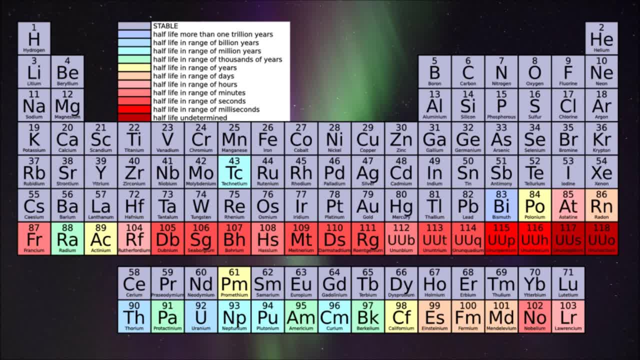 KR, Krypton, RB. Rubidium, SR, Strontium Y, Yttrium, ZR. Zirconium NB, Niobium, MO, Molybdenum, TC, Technetium. 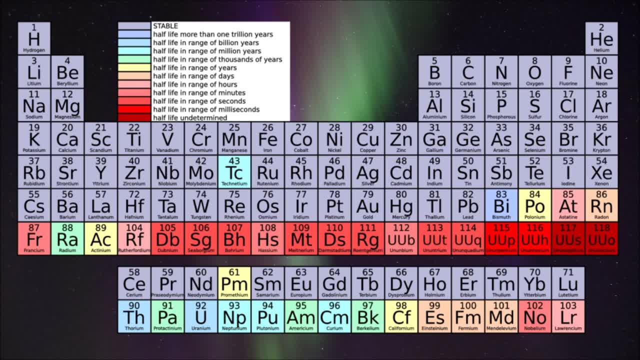 RU, Ruthenium, RH, Rhodium, PD, Palladium, AG, Silver, CD, Cadmium IN Indium, SN, Tin, SB, Antimony, TE Tellurium. 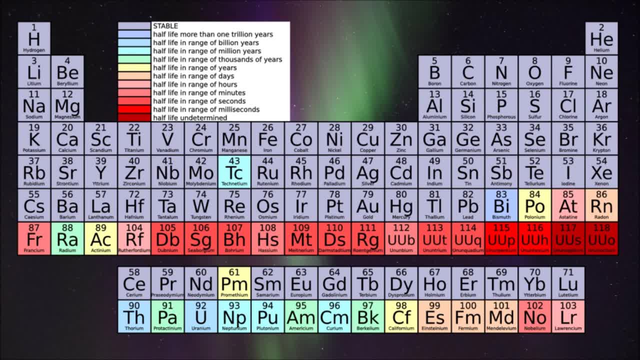 I, Iodon, XE, Xenon, CS, Cesium BA, Barium, LA, Lanthanum, CE, Cerium, PR, Praseodynium, ND, Neodynium. 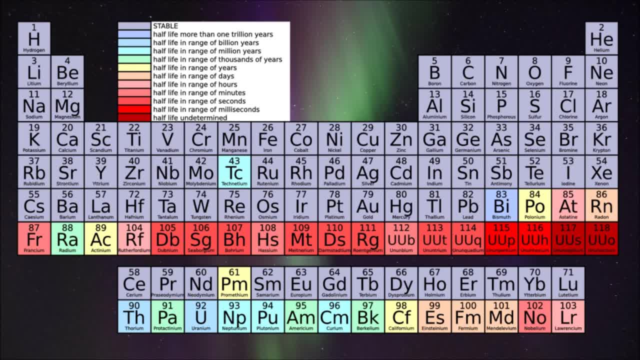 PM Promethium, SM, Cimmerium, EU, Europium GD, Gadolinium, TB, Terbium DY, Dysprosium, HO, Holmium ER, Erbium. 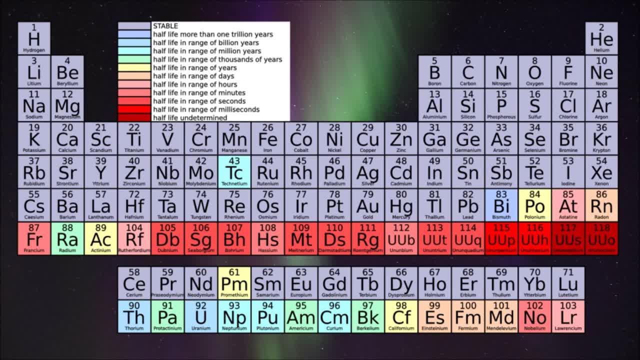 OS, Osmium, IR, Iridium, PT, Platinum, AU, Gold, HG, Mercury, TL, Thallium, PB, Lead, BI, Bismuth, PO, Polonium. 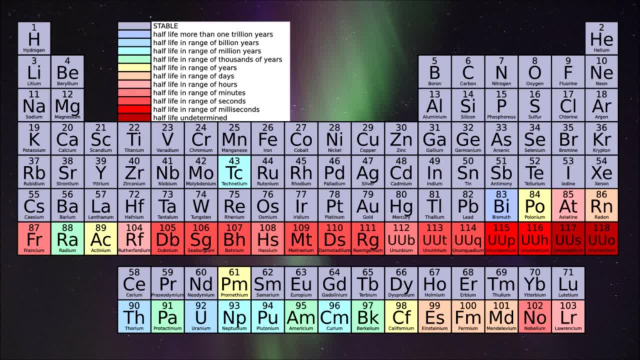 AT. Astatine, RN, Radon, FR, Francium, RA. Radium AC, Actinium, TH, Thorium, PA, Protactinium U, Uranium, NP, Neptunium. 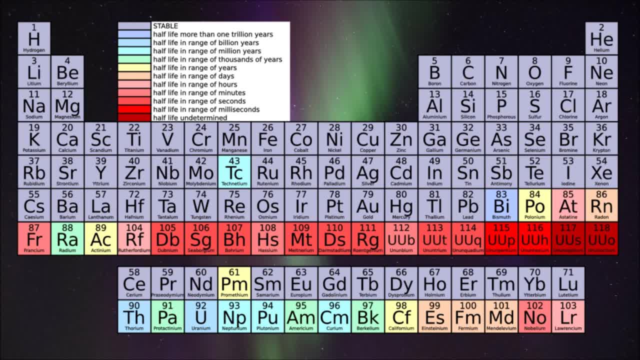 PU Plutonium, AM, Ameritium, CM, Curium BK, Berkelium, CF. Californium, ES, Einsteinium, FM, Fermium MD. Mendelevium. NO Nobellium, LR, Laurentium, RF, Rutherfordium DB, Dubnium, SG, Cyborgium, BH, Borium HS, Hassium, MT, Mitnerium. DS: Darmstadium RG. Runtinium CN. Copernicium UUT- Anuntrium FL. Florovium UUP. Anunpincium LV- Livermorium. 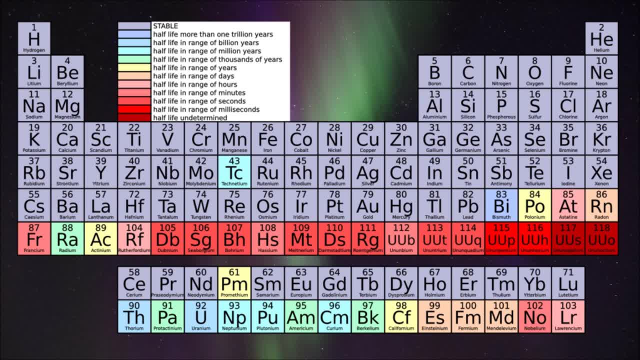 UUS, Anunseptium, UUO, Anunoxium HHydrogen, HE, Helium LI, Lithium BE, Beryllium, BB, Boron, CC, Carbon. 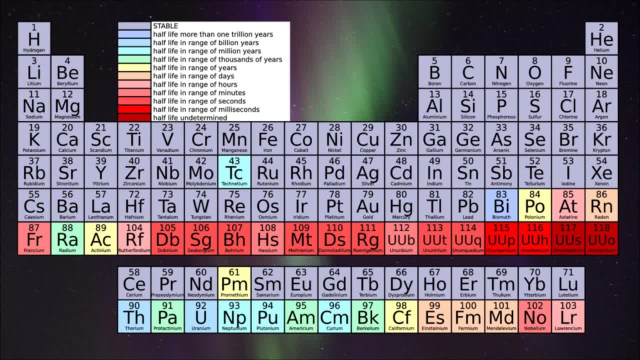 NNitrogen, OOxygen, FFluorine, NE, Neon, NA, Sodium, MG, Magnesium, AL, Aluminum, SI, Silicon, PP, Phosphorus, SSulfur. 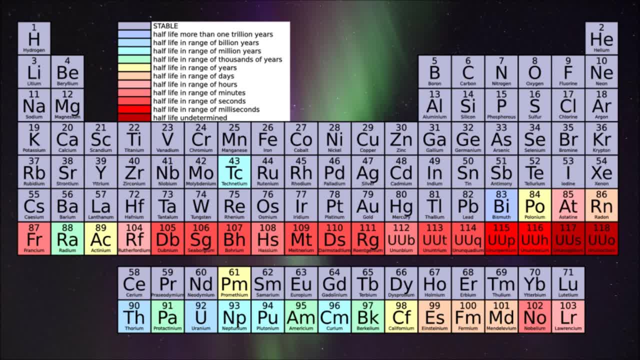 CL, Chlorine, AR, Argon, KK, Potassium, CA, Calcium, SC, Scandium, TI, Titanium, VVanadium, CR, Chromium, MN, Manganese. 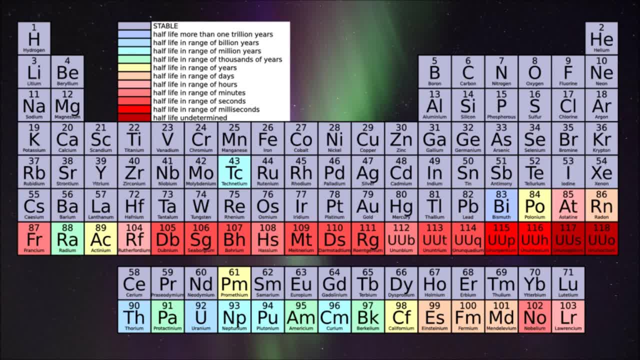 FE, Iron, CO Cobalt, NI Nickel, CU Copper, ZN, Zinc, GA, Gallium, GE, Germanium, AS, Arsenic, SE, Selenium, BR, Bromine. 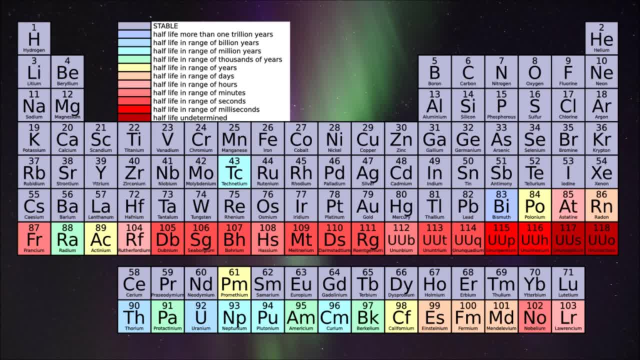 KR, Krypton, RB. Rubidium, SR, Strontium Y, Yttrium, ZR. Zirconium NB, Niobium, MO, Molybdenum, TC, Technetium. 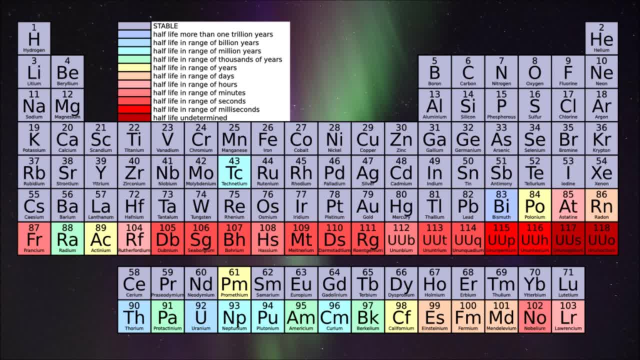 RU, Ruthenium, RH, Rhodium, PD, Palladium, CG, Silver, CD, Cadmium, IN Indium, SN, Tin, SB, Antimony, TE, Tellurium. 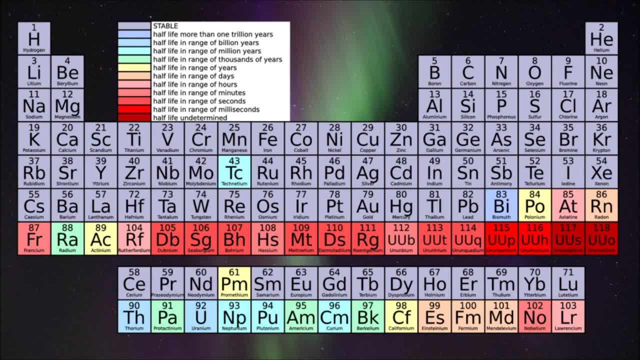 I. Iodine, XE, Xenon, CS, Cesium, BA, Barium, LA, Lanthanum, CE, Cerium, PR, Praseodynium, ND, Neodynium. 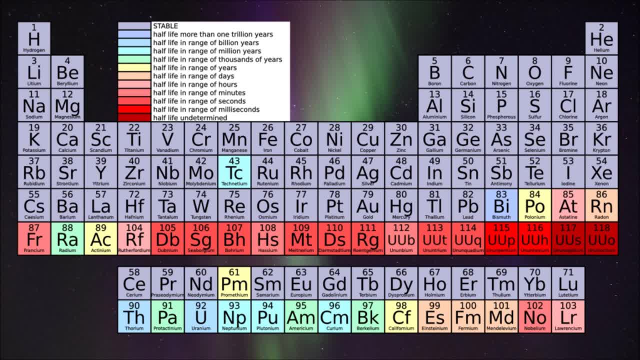 PM Promethium, SM, Cimmerium, EU, Europium GD, Gadolinium, TB, Terbium DY, Dysprosium, HO, Holmium ER, Erbium. TM Thulium YB. Ytterbium LU. Lutetium HF. Hafnium TA. Tantalum W Tungsten RE Rhenium. 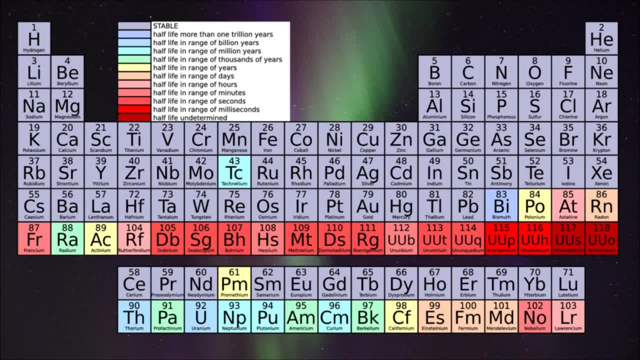 OS, Osmium, IR, Iridium, PT, Platinum, AU, Gold, HG, Mercury, TL, Thallium, PB, Lead, BI, Bismuth, PO, Polonium. 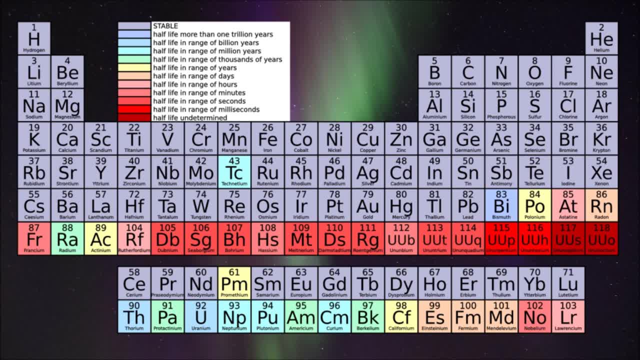 AT. Astatine, RN, Radon, FR, Francium, RA. Radium AC, Actinium, TH, Thorium, PA, Protactinium U, Uranium, NP, Neptunium. 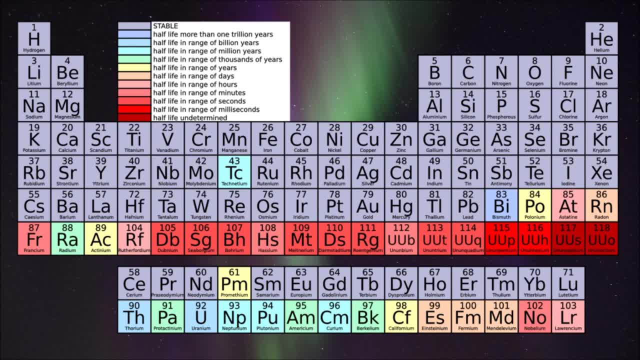 PU, Plutonium, AM, Emeritium, CM, Curium BK, Berkelium, CF. Californium, ES. Einsteinium, FM, Fermium MD. Mendelevium. NO. Nobelium, LR, Laurentium, RF, Rutherfordium DB, Dubnium, SG, Cyborgium, BH, Borium, HS, Hacium, MT, Mitnerium. DS: Darmstadium RG. Runtinium CN. Copernicium UUT- Anuntrium FL. Fluorovium UUP. Anunpincium LV- Livermorium. 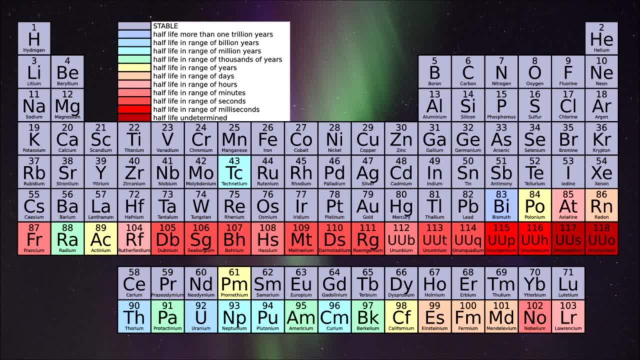 UUS Anunception- UUO Anunoxium: H, Hydrogen, HE, Helium LI, Lithium BE, Beryllium BE, Boron, CE, Carbon. 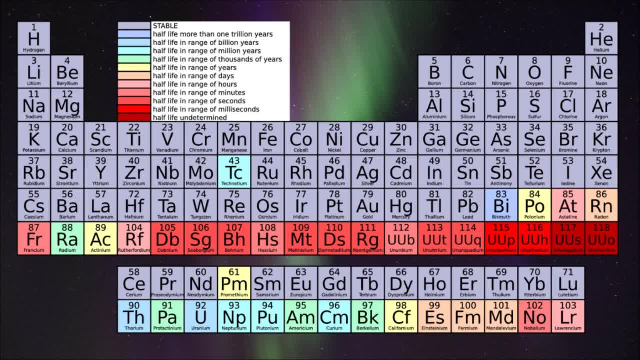 NE, Nitrogen, OE, Oxygen, FE, Fluorine, NE, Neon, NA, Sodium, MG, Magnesium, AL, Aluminum, SI, Silicon, P, Phosphorus S, Sulfur. 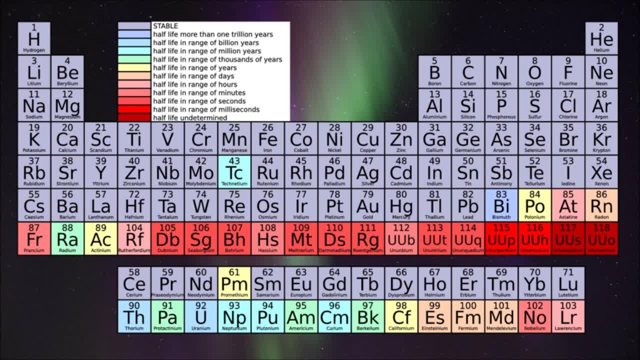 CL, Chlorine, AR, Argon K, Potassium, CA, Calcium, SC, Scandium, TI, Titanium V, Vanadium, CR, Chromium, MN, Manganese, FE, Iron. 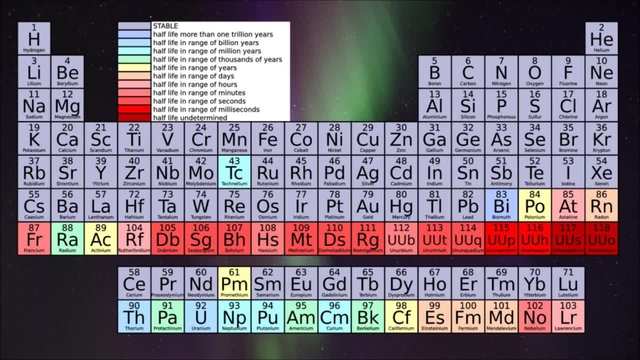 CO, Cobalt, NI, Nickel, CU Copper, ZN, Zinc, GA, Gallium, GE, Germanium, AS, Arsenic, SE, Selenium, BR, Bromine. 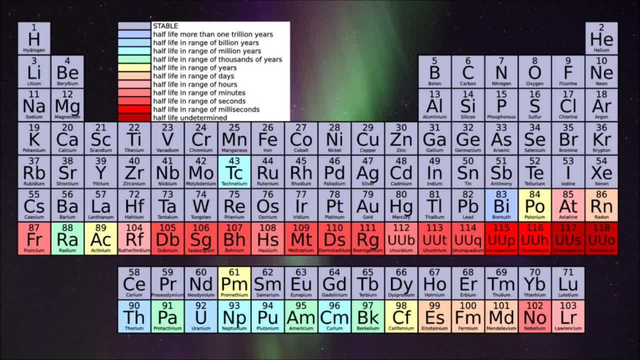 KR, Krypton, RB. Rubidium, SR, Strontium Y, Yttrium, ZR. Zirconium NB, Niobium, MO, Molybdenum, TC, Technetium. 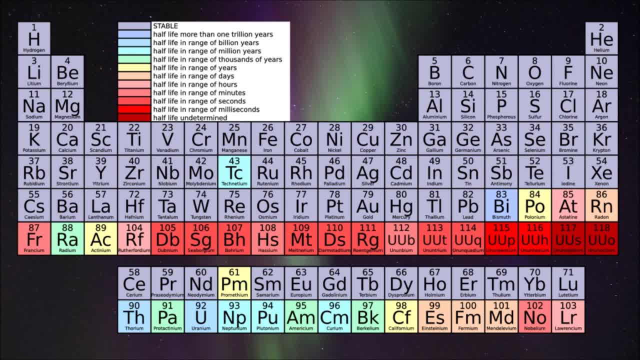 RU, Ruthenium, RH, Rhodium, PD, Palladium, AG, Silver, CD, Cadmium IN Indium, SN, Tin, SB, Antimony, TE Tellurium. 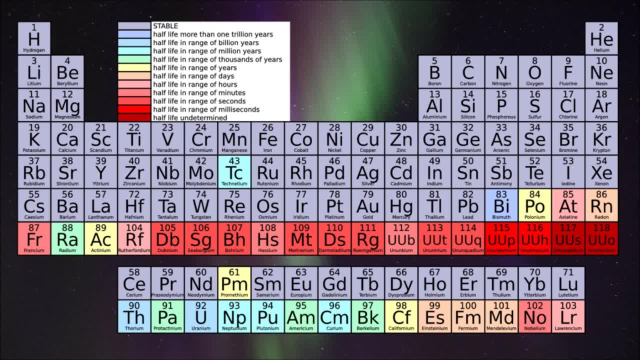 I, Iodon, XE, Xenon, CS, Cesium BA, Barium, LA, Lanthanum, CE, Cerium, PR, Praseodynium, ND, Neodynium. 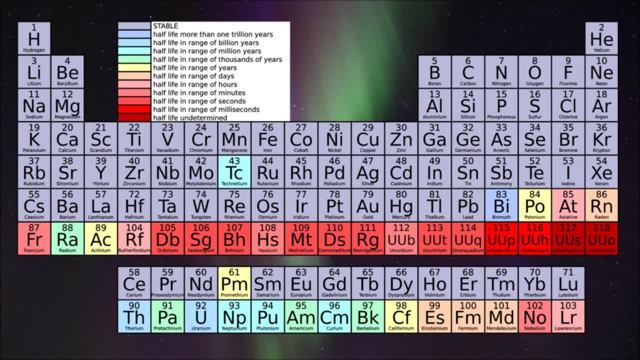 PM. Promethium, SM, Samarium, EU, Europium, GD, Gadolinium, TB, Terbium, DY, Dysprosium, HO, Holmium, ER, Erbium. TM Thulium YB. Ytterbium LU. Lutetium HF. Hafnium TA. Tantalum W Tungsten RE Rhenium. 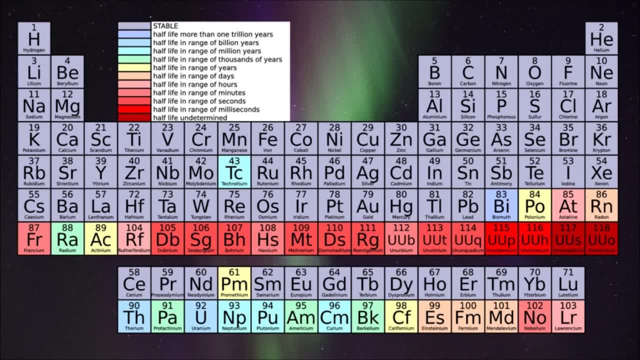 OS, Osmium, IR, Iridium, PT, Platinum, AU, Gold, HG, Mercury, TL, Thallium, PB, Lead, BI, Bismuth, PO, Polonium. 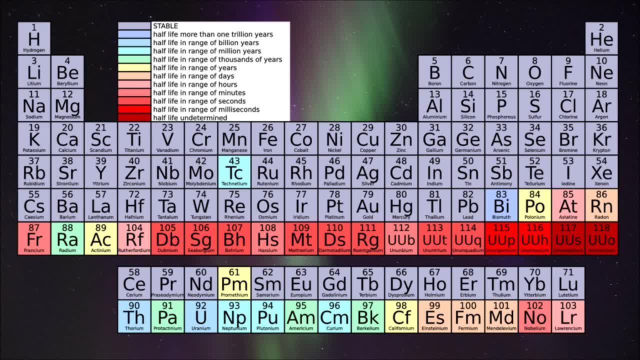 AT. Astatine, RN, Radon, FR, Francium, RA. Radium AC, Actinium, TH, Thorium, PA, Protactinium U, Uranium, NP, Neptunium. 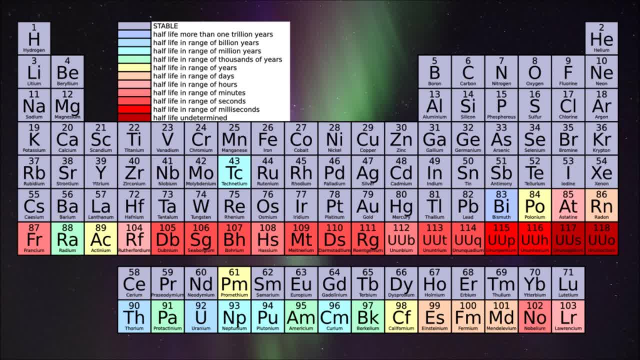 PU, Plutonium, AM, Emeritium, CM, Curium BK, Berkelium, CF. Californium, ES. Einsteinium, FM, Fermium MD. Mendelevium. 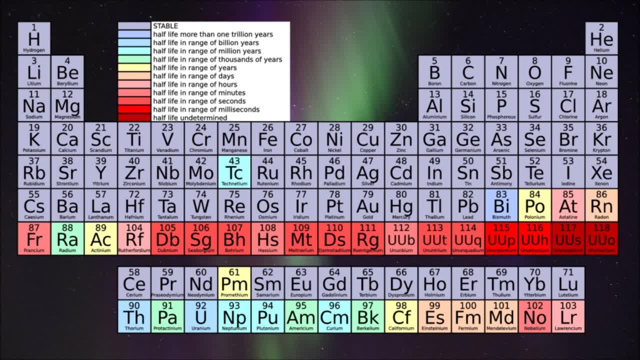 UUS Anunseption- UUO Anunoxium H, Hydrogen HE, Helium LI, Lithium BE, Beryllium BE, Boron C Carbon. N, Nitrogen O, Oxygen F, Fluorine, NE, Neon, NA, Sodium, MG, Magnesium, AL, Aluminum, SI, Silicon, P, Phosphorus S, Sulphur. 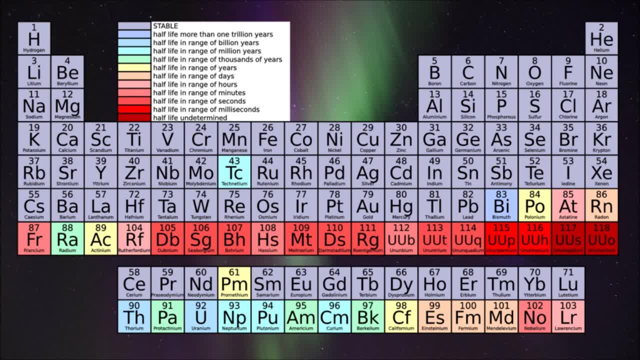 CL, Chlorine, AR, Argon K, Potassium, CA, Calcium, SC, Scandium, TI, Titanium V, Vanadium, CR, Chromium, MN, Manganese, FE, Iron. 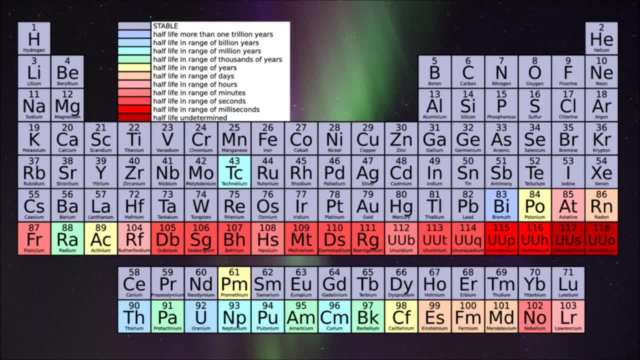 CO, Cobalt, NI, Nickel, CU Copper, ZN, Zinc, GA, Gallium, GE, Germanium, AS, Arsenic, SE, Selenium, ER Bromine. 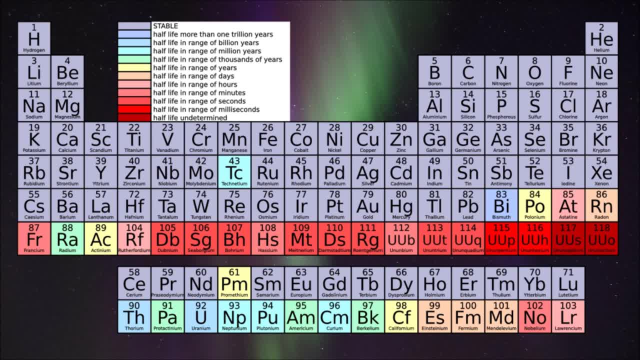 KR. Krypton, RB. Rubidium, SR, Strontium, Y. Yttrium, ZR. Zirconium, NB, Niobium, MO, Molybdenum, CC, Technetium. 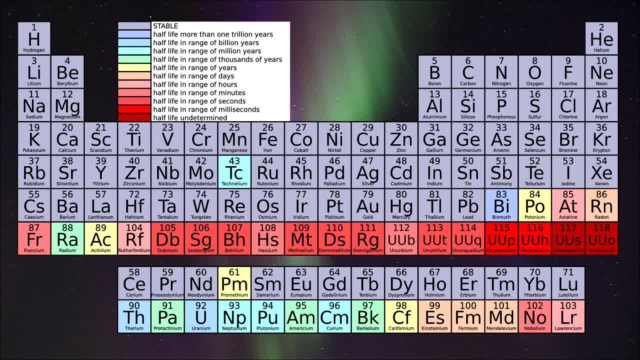 RU, Ruthenium, RH, Rhodium, PD, Palladium, AG, Silver, CD, Cadmium IN Indium, SN, Tin, SB, Antimony, TE Tellurium. 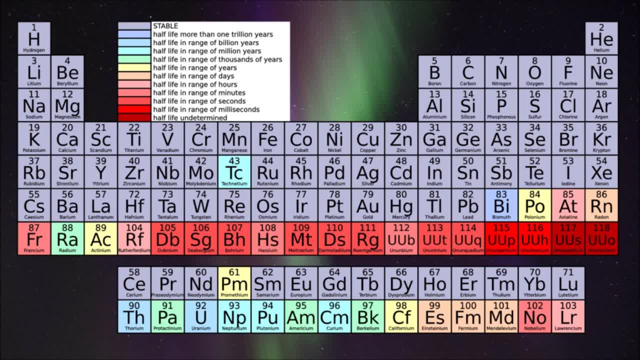 IIodon, XE, Xenon, CS, Cesium, BA, Barium, LA, Lanthanum, CE, Cerium, PR, Praseodynium, ND, Neodynium. 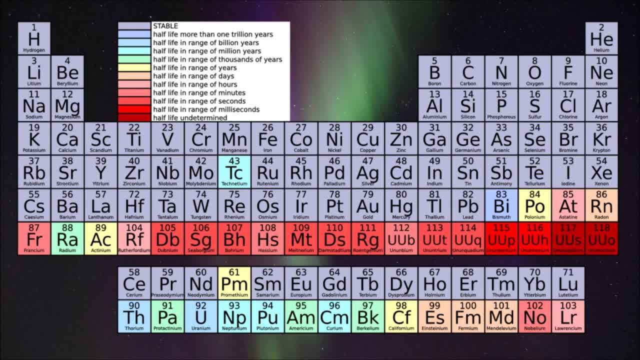 PM Promethium, SM, Cimmerium, EU, Europium GD, Gadolinium, TB, Terbium DY, Dysprosium, HO, Holmium ER, Erbium. TM Thulium YB. Ytterbium LU. Lutetium HF. Hafnium TA. Tantalum W Tungsten RE Rhenium. 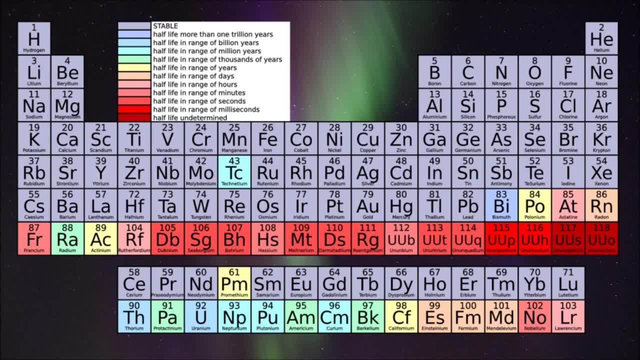 OS, Osmium, IR, Iridium, PT, Platinum, AU, Gold, HG, Mercury, TL, Thallium, PB, Lead, BI, Bismuth, PO, Polonium. 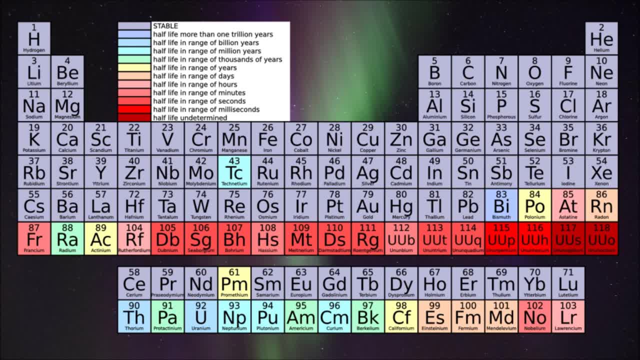 AT. Astatine, RN, Radon, FR, Francium, RA. Radium AC, Actinium, TH, Thorium, PA, Protactinium U, Uranium, NP, Neptunium. 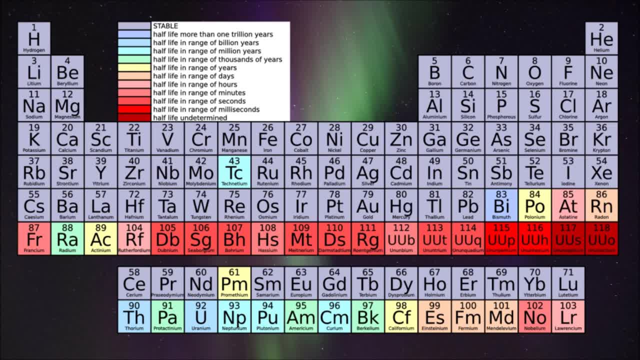 PU Plutonium, AM, Ameritium, CM, Curium BK, Berkelium, CF. Californium, ES, Einsteinium, FM, Fermium MD. Mendelevium. 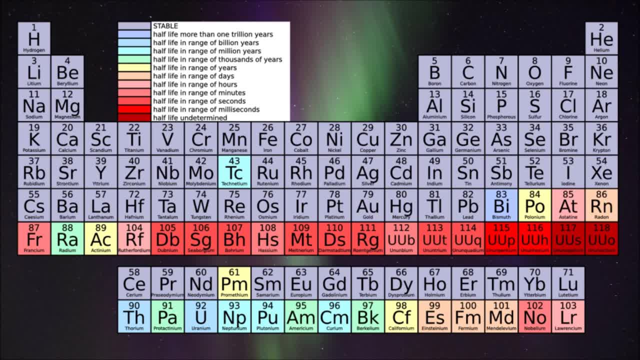 UUS, Anunseptium, UUO, Anunoxium HHydrogen, HE, Helium LI, Lithium BE, Beryllium, BB, Boron, CC, Carbon. 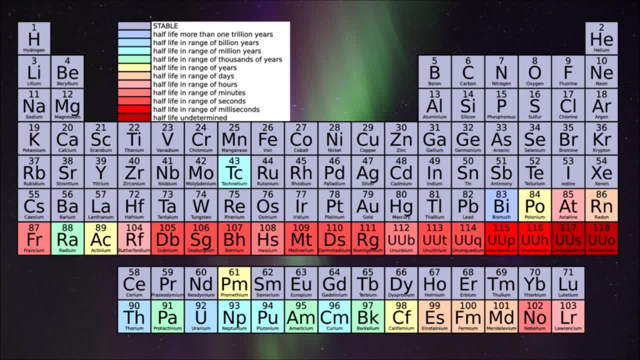 NNitrogen, OOxygen, FFluorine, NE, Neon, NA, Sodium, MG, Magnesium, AL, Aluminum, SI, Silicon, P, Phosphorus S, Sulfur. 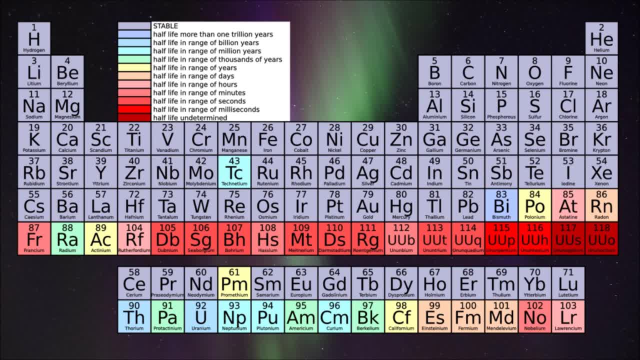 CL, Chlorine, AR, Argon K, Potassium, CA, Calcium, SC, Scandium, TI, Titanium V, Vanadium, CR, Chromium, MN, Manganese, FE, Iron. 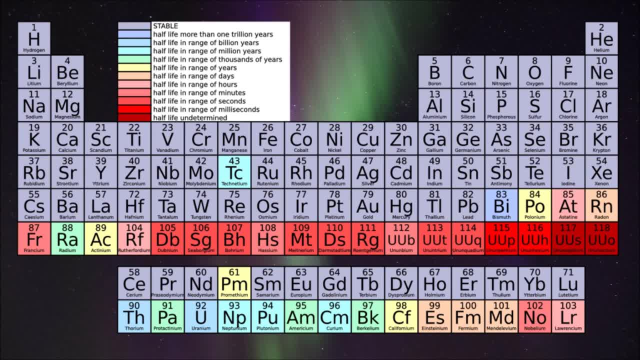 CO, Cobalt, NI, Nickel, CU Copper, ZN, Zinc, GA, Gallium, GE, Germanium, AS, Arsenic, SE, Selenium, BR, Bromine. 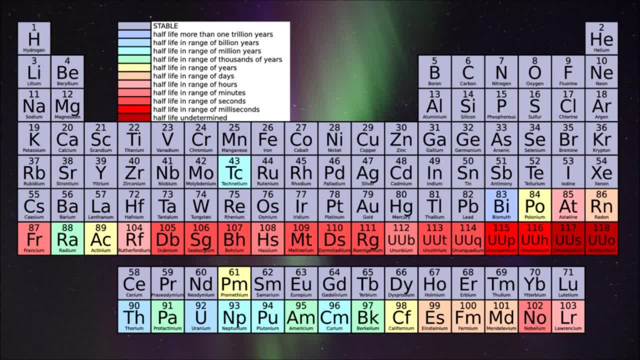 KR, Krypton, RB. Rubidium, SR, Strontium Y, Yttrium, ZR. Zirconium NB, Niobium, MO, Molybdenum, TC, Technetium. 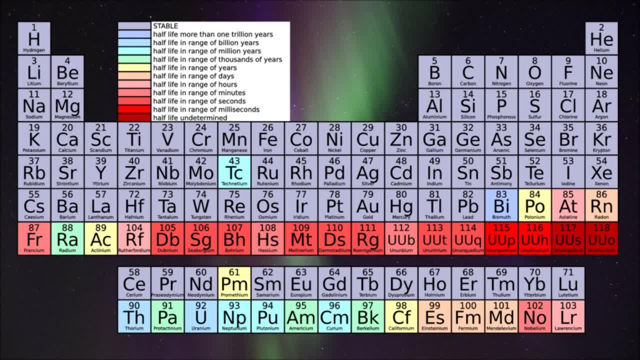 RU, Ruthenium, RH, Rhodium, PD, Palladium, AG, Silver, CD, Cadmium IN Indium, SN, Tin, SB, Antimony, TE Tellurium. 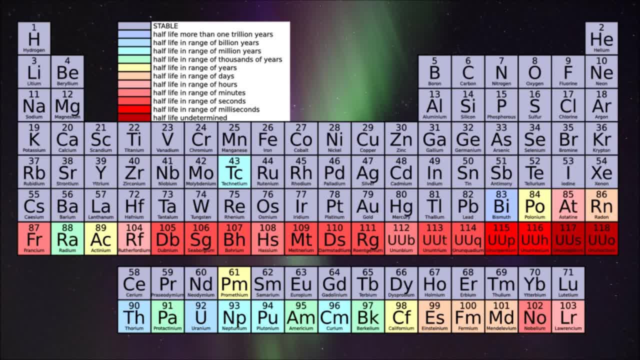 I, Iodon, XE, Xenon, CS, Cesium BA, Barium, LA, Lanthanum, CE, Cerium, PR, Praseodynium, ND, Neodynium. 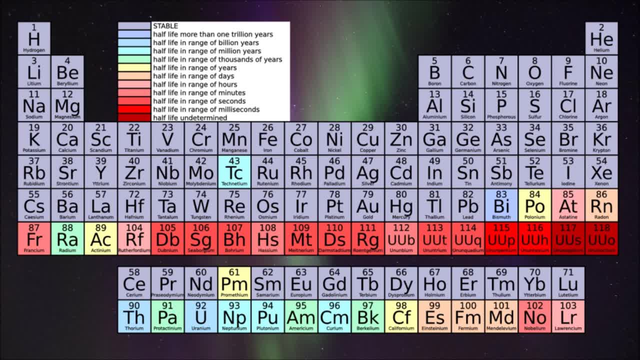 PM Promethium, SM, Cimmerium, EU, Europium GD, Gadolinium, TB, Terbium DY, Dysprosium, HO, Holmium ER, Erbium. TM Thulium YB. Ytterbium LU. Lutetium HF. Hafnium TA. Tantalum W Tungsten RE Rhenium. 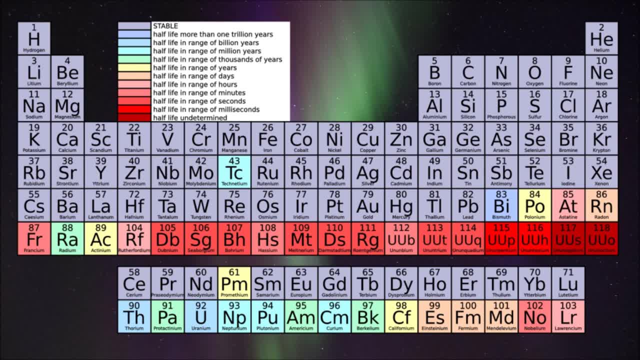 OS, Osmium, IR, Iridium, PT, Platinum, AU, Gold, HG, Mercury, TL, Thallium, PB, Lead, BI, Bismuth, PO, Polonium. 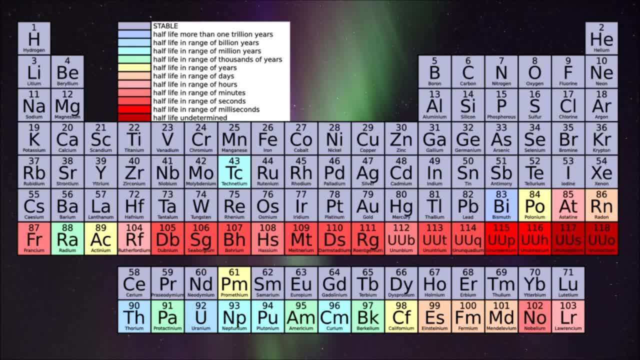 AT. Astatine, RN, Radon, FR, Francium, RA. Radium AC, Actinium, TH, Thorium, PA, Protactinium U, Uranium, NP, Neptunium. 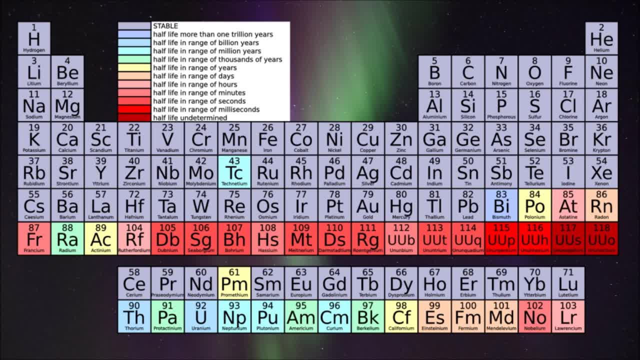 PU Plutonium, AM, Ameritium, CM, Curium BK, Berkelium, CF. Californium, ES, Einsteinium, FM, Fermium MD. Mendelevium. NO Nobellium, LR, Laurentium, RF, Rutherfordium DB, Dubnium, SG, Cyborgium, BH, Borium HS, Hassium, MT, Mitnerium. DS: Darmstadium RG. Runtinium CN. Copernicium UUT- Anuntrium FL. Florovium UUP. Anunpincium LV- Livermorium. 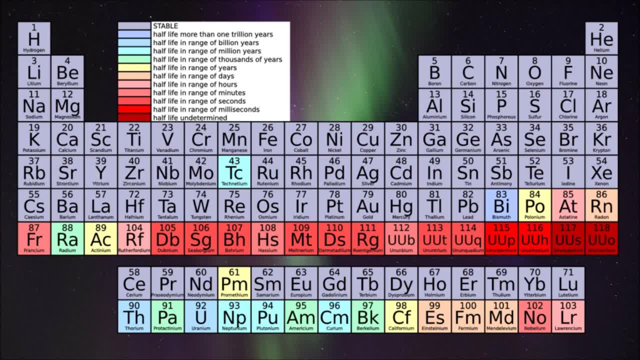 UUS Anunseption. UUO Anunoxium HHydrogen, HE, Helium LI, Lithium BE, Beryllium, BB, Boron, CC, Carbon. 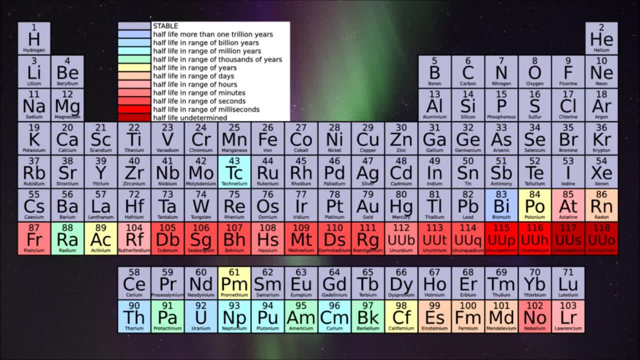 NNitrogen, OOxygen, FFluorine, NE, Neon, NA, Sodium, MG, Magnesium, AL, Aluminum, SI, Silicon, PP, Phosphorus, SSulfur. 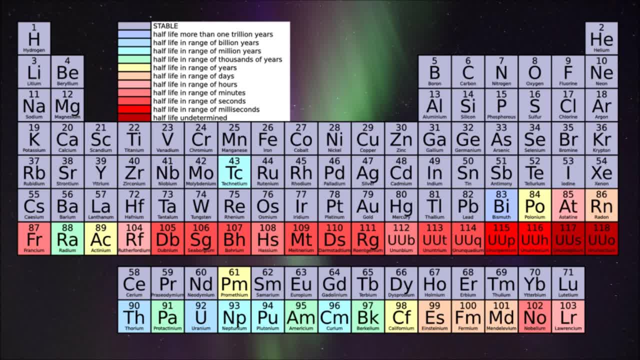 CL, Chlorine, AR, Argon, KK, Potassium, CA, Calcium, SC, Scandium, TI, Titanium, VV, Vanadium, CR, Chromium, MN, Manganese. 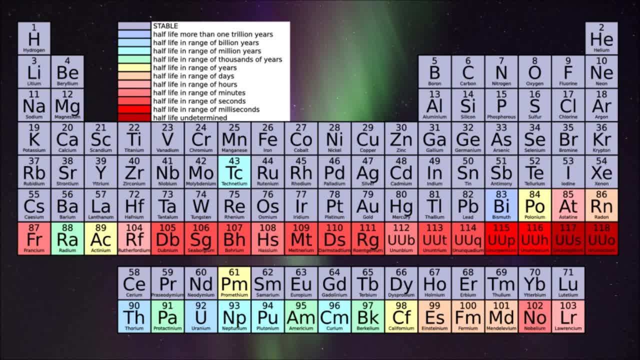 FE, Iron, CO Cobalt, NI Nickel, CU Copper, ZN, Zinc, GA, Gallium, GE, Germanium, AS, Arsenic, SE, Selenium, BR, Bromine. 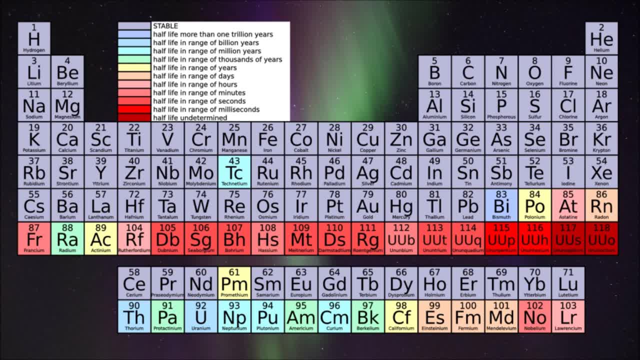 KR, Krypton, RB, Rubidium SR, Strontium, YYttrium, ZR, Zirconium NB, Niobium, MO, Molybdenum, TC, Technetium. 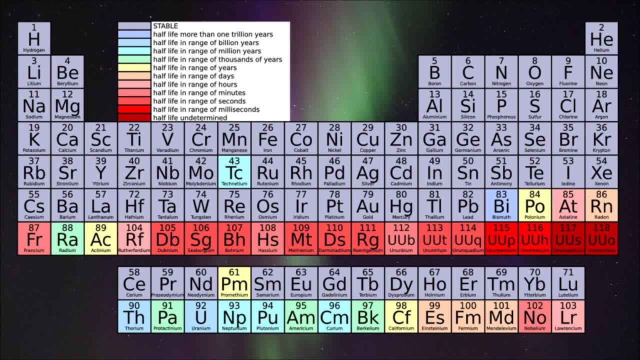 RU, Ruthenium, RH, Rhodium, PD, Palladium, CG, Silver, CD, Cadmium, IN Indium, SN, Tin, SB, Antimony, TE, Tellurium. 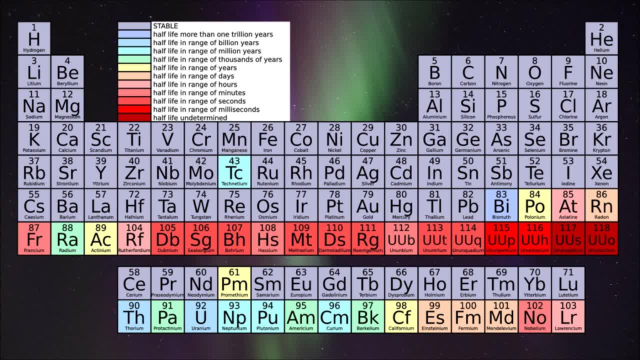 IIodon, XE, Xenon, CS, Cesium, BA, Barium, LA, Lanthanum, CE, Cerium, PR, Praseodynium, ND, Neodynium. 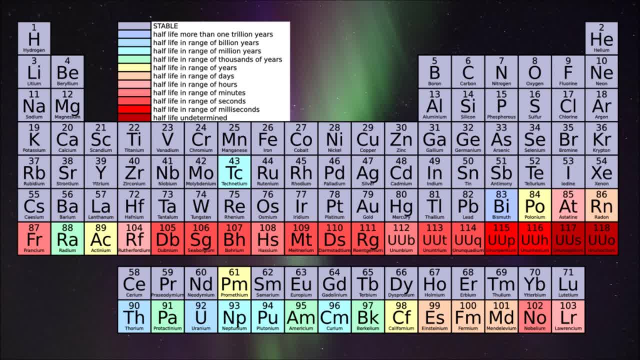 PM Promethium, SM, Cimmerium, EU, Europium GD, Gadolinium, TB, Terbium DY, Dysprosium, HO, Holmium ER, Erbium. TM Thulium YB. Ytterbium LU. Lutetium HF. Hafnium TA. Tantalum W Tungsten RE Rhenium. 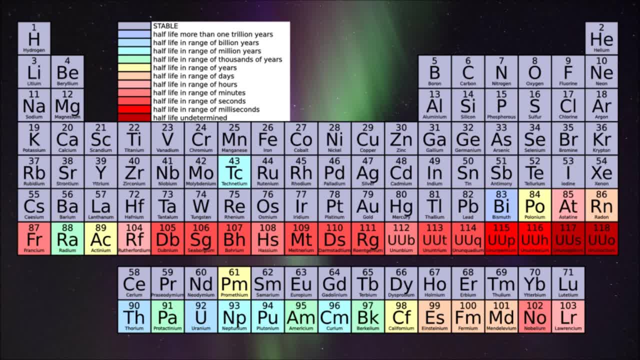 OS, Osmium, IR, Iridium, PT, Platinum, AU, Gold, HG, Mercury, TL, Thallium, PB, Lead, BI, Bismuth, PO, Polonium. 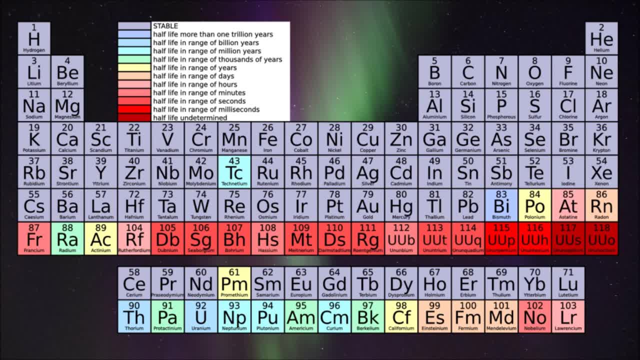 AT. Astatine, RN, Radon, FR, Francium, RA. Radium AC, Actinium, TH, Thorium, PA, Protactinium U, Uranium, NP, Neptunium. 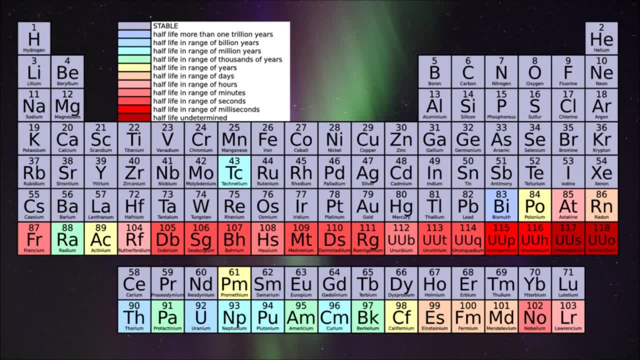 PU, Plutonium, AM, Emeritium, CM, Curium BK, Berkelium, CF. Californium, ES. Einsteinium, FM, Fermium MD. Mendelevium. NO. Nobelium, LR, Laurentium, RF, Rutherfordium DB, Dubnium, SG, Cyborgium, BH, Borium, HS, Hacium, MT, Mitnerium. DS: Darmstadium RG. Runtinium CN. Copernicium UUT- Anuntrium FL. Fluorovium UUP. Anunpincium LV- Livermorium. UUS, Anunseptium, UUO, Anunoxium: H, Hydrogen, HE, Helium LI, Lithium BE, Beryllium BE, Boron, CE, Carbon. 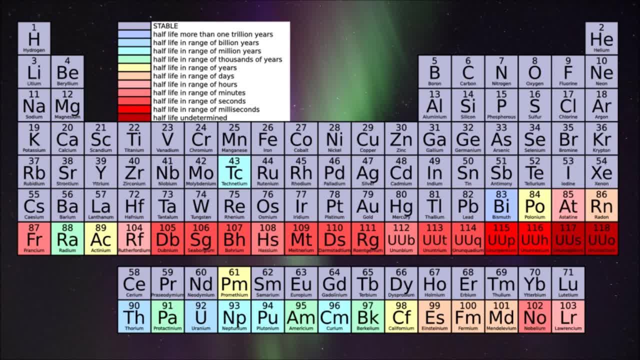 NE, Nitrogen, OE, Oxygen, FE, Fluorine, NE, Neon, NA, Sodium, MG, Magnesium, AL, Aluminum, SI, Silicon, P, Phosphorus S, Sulfur. 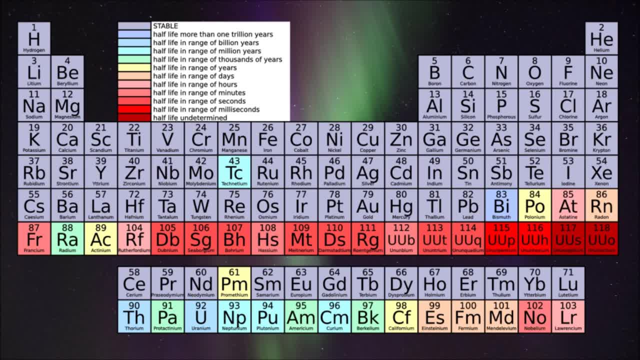 CL, Chlorine, AR, Argon K, Potassium, CA, Calcium, SC, Scandium, TI, Titanium V, Vanadium, CR, Chromium, MN, Manganese, FE, Iron. 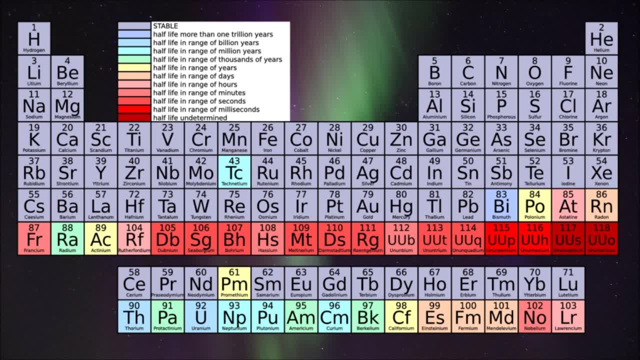 CO, Cobalt, NI, Nickel, CU Copper, ZN, Zinc, GA, Gallium, GE, Germanium, AS, Arsenic, SE, Selenium, BR, Bromine. 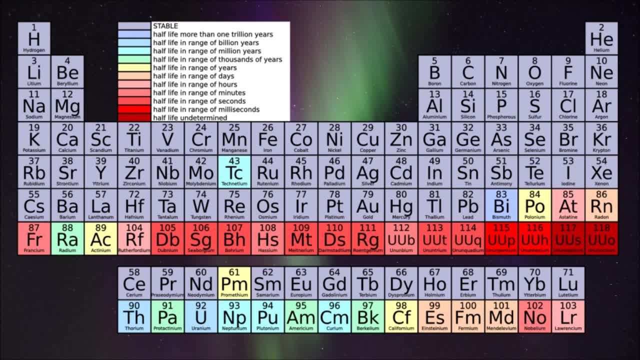 KR, Krypton, RB. Rubidium, SR, Strontium Y, Yttrium, ZR. Zirconium NB, Niobium, MO, Molybdenum, TC, Technetium. 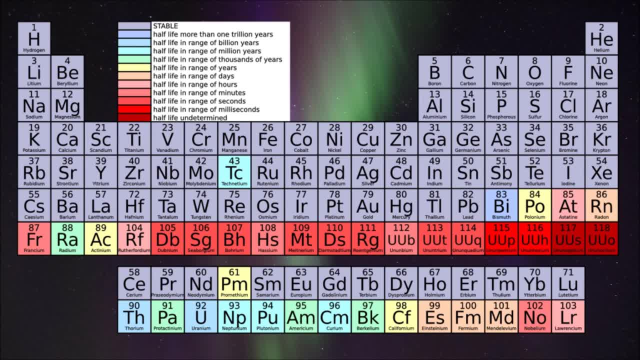 RU, Ruthenium, RH, Rhodium, PD, Palladium, AG, Silver, CD, Cadmium IN Indium, SN, Tin, SB, Antimony, TE Tellurium. 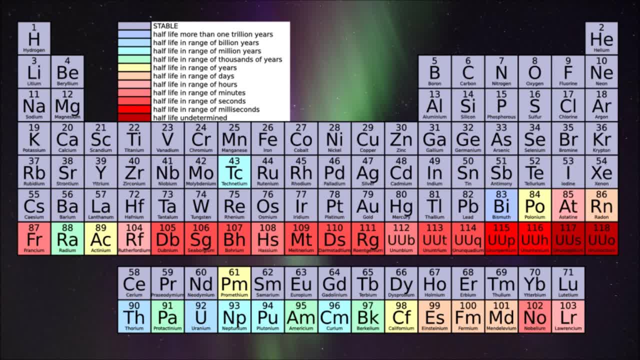 I, Iodon, XE, Xenon, CS, Cesium BA, Barium, LA, Lanthanum, CE, Cerium, PR, Praseodynium, ND, Neodynium. 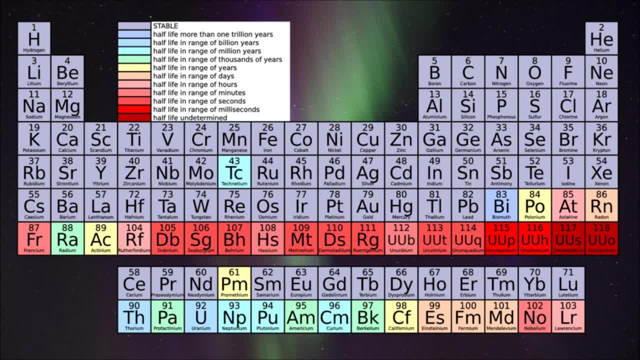 PM. Promethium, SM, Samarium, EU, Europium, GD, Gadolinium, TB, Terbium, DY, Dysprosium, HO, Holmium, ER, Erbium. TM Thulium YB. Yterbium LU. Lutetium HF. Hafnium TA. Tantalum W Tungsten RE Rhenium. 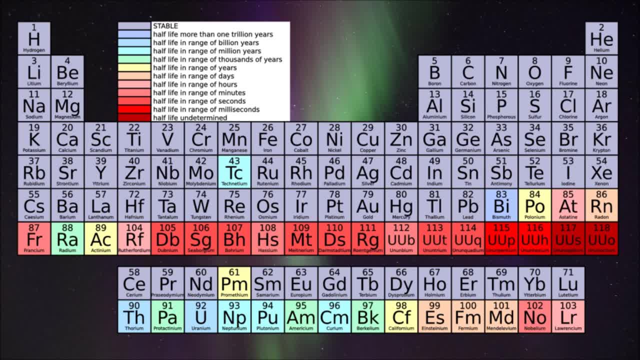 OS, Osmium, IR, Iridium, PT, Platinum, AU, Gold, HG, Mercury, TL, Thallium, PB, Lead, BI, Bismuth, PO, Polonium. 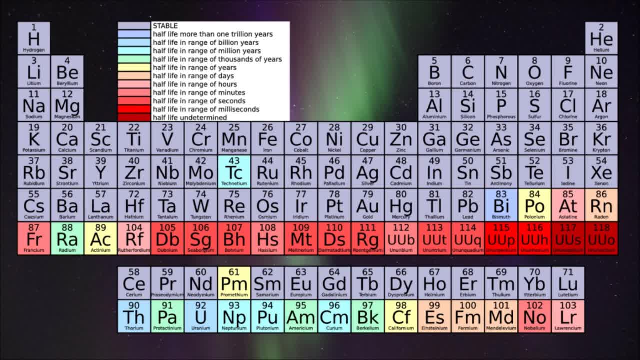 AT. Astatine, RN, Radon, FR, Francium, RA. Radium AC, Actinium, TH, Thorium, PA, Protactinium U, Uranium, NP, Neptunium. 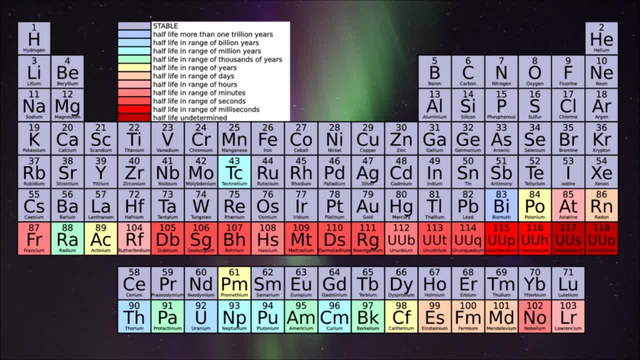 PU, Plutonium, AM, Emeritium, CM, Curium BK, Berkelium, CF. Californium, ES. Einsteinium, FM, Fermium MD. Mendelevium. NO. Nobelium, LR, Laurentium, RF, Rutherfordium DB, Dubnium, SG, Cyborgium, BH, Borium, HS, Hacium, MT, Mitnerium. DS: Darmstadium RG. Runtinium CN. Copernicium UUT- Anuntrium FL. Florovium UUP. Anunpincium LV- Livermorium. 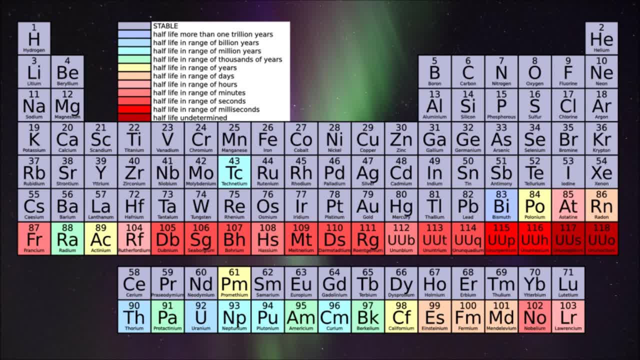 UUS Anunseptium, UUO, Anunnoxium A GS, CF, AG, AG, AG, AG, AG, AG. Thank you, Thank you. 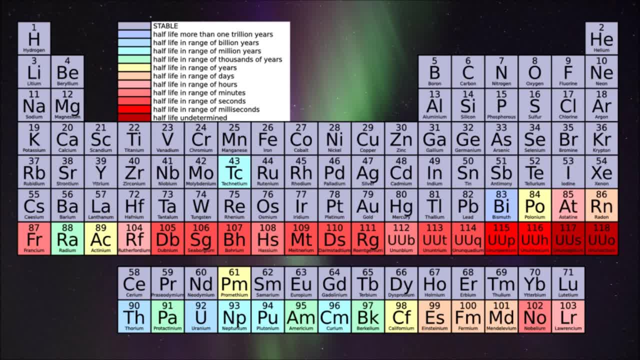 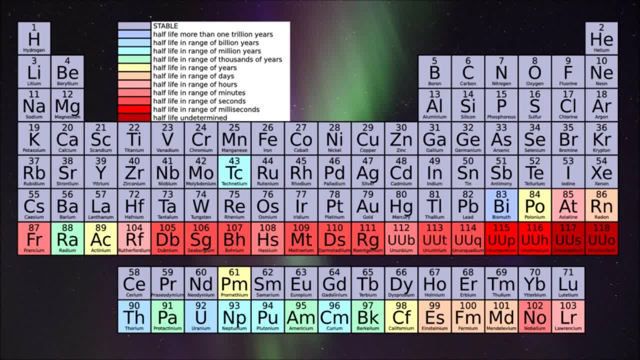